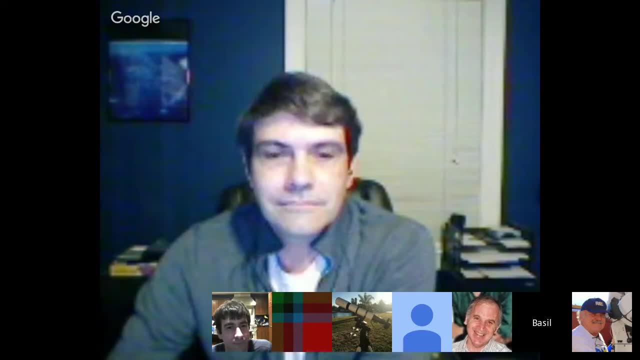 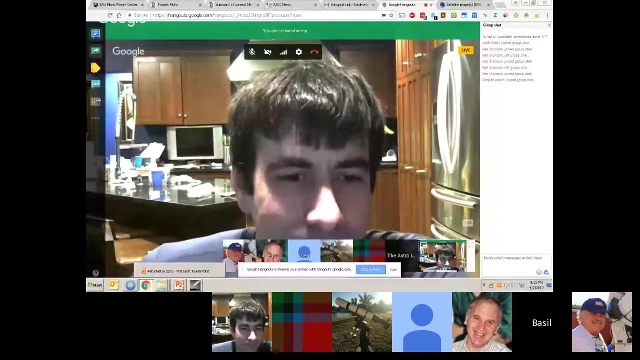 And Basil, the floor is yours. Okay, Thank you. Am I there? Can you hear me? You're here. yeah, All right, I'm going to screen share my entire screen. Get to my presentation. Can you see the presentation there? 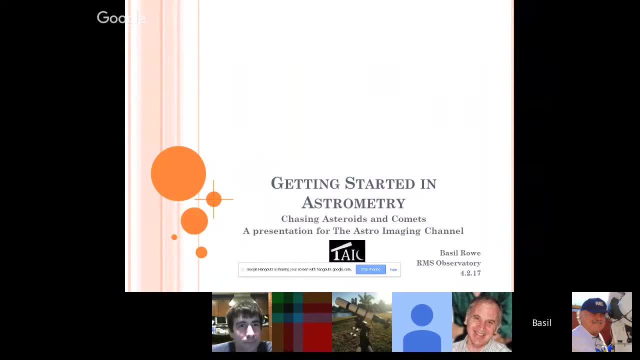 Go full screen with that. Yes, perfect, All right. Well, first I'd like to thank Adam very much for inviting me here to talk tonight. I've been watching the Astro Imaging channel for several months and I think the contribution to astronomy that this is making is just fantastic. 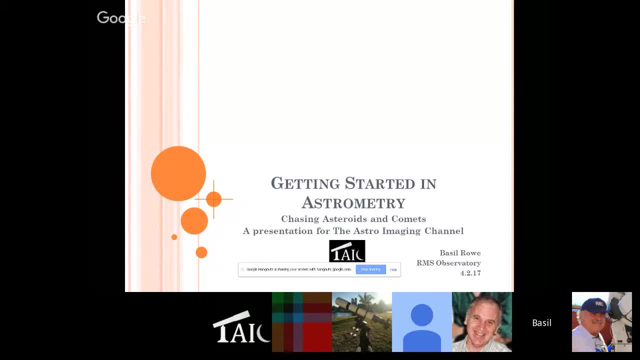 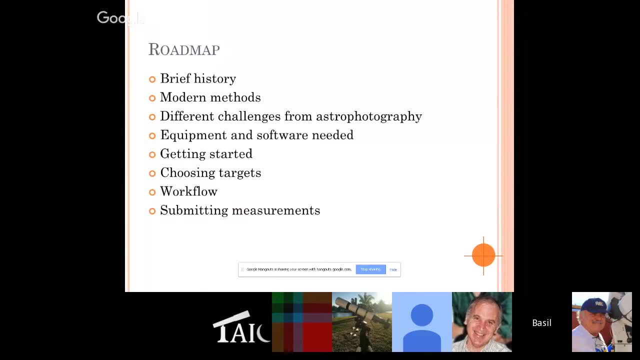 So getting started in astrometry To start off with this is kind of where I hope we go tonight. Talk a little bit about the history very briefly, modern methods I find it helpful to talk about. to look at the history to kind of see where we came from, to greater appreciate where we are. 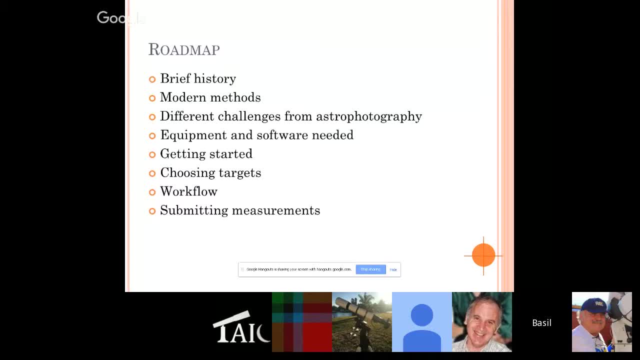 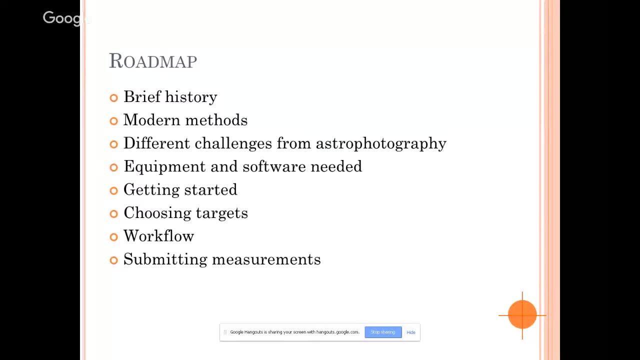 Also some of the different challenges from astrophotography. A little bit about the equipment and the software that you probably will need. Just a quick note about getting started And then talk a fair amount about how to choose targets. Where I first got into astrophotography, I was a photographer. 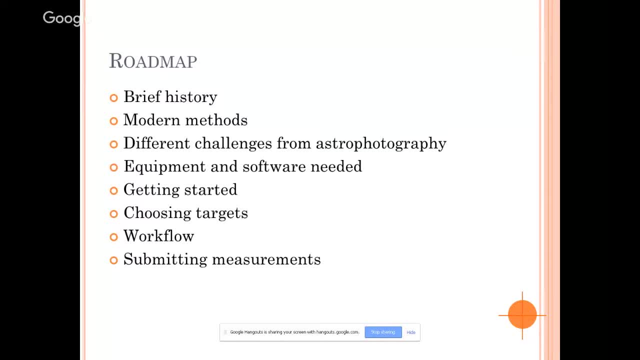 When I first got into this, choosing targets to image was very overwhelming, So hopefully I can help with that. A little bit about the workflow: This is just how I do it, which probably isn't the best way, But it's how I do it and it works pretty well for me. 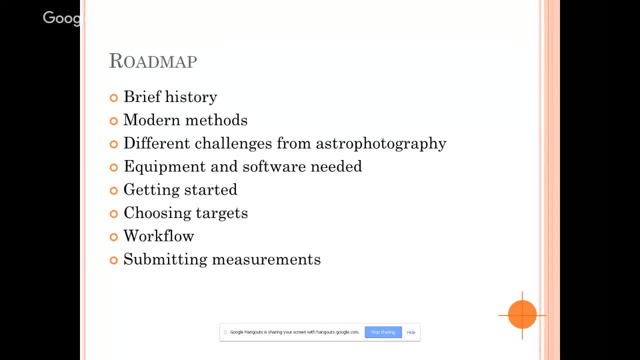 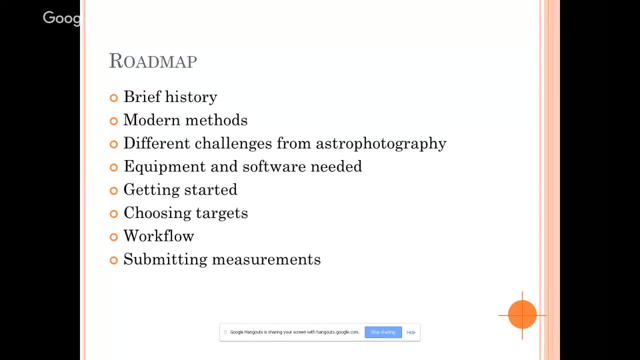 So, as I was putting this together, I realized that my hope is tonight to inspire some of you to explore this. It is, I think, an exciting and interesting field And there's probably way too much to try and communicate on how to perhaps get started with this. 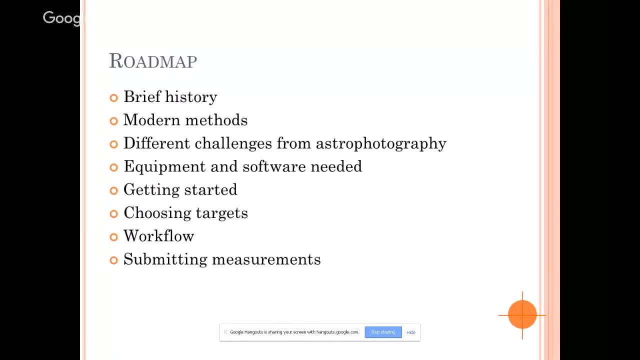 So I put together some screencasts And I put them on YouTube and I've shared them And at the end of this there's a link to get to that- And basically a lot of those are dealing with choosing targets in the workflow and stuff like that. 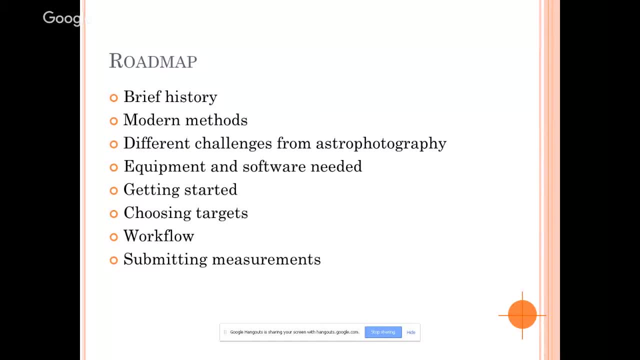 Some of the details. we're going to have some more time to actually go through some demonstration of that, So I'm going to go through some of that here, But hopefully this is just to kind of give you an idea and to hopefully inspire you. 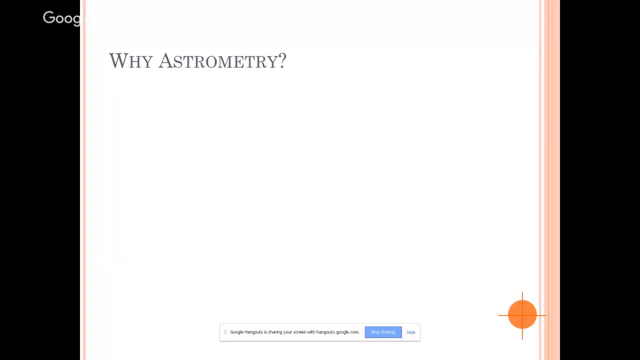 So to get started. So why astrometry? Well, and I'm talking here about just astrometry of comets and asteroids, You know, the positional astronomy is perhaps the oldest form of astronomy. Astronomers love to make measurements and take positions of things. 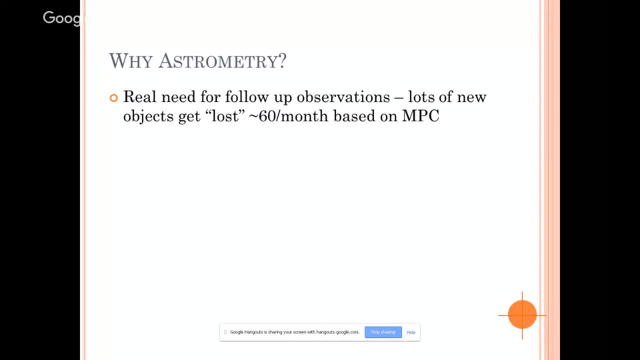 But for comets and asteroids there's a real need for follow-up observations of the new objects. A lot of these new objects that are discovered by these robotic surveys just get lost And going back Over Over the last three months from the listing in the Minor Planet Center, I counted about 60 a month that are just lost. 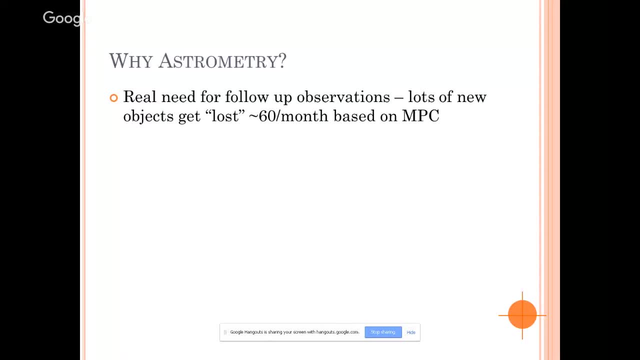 They don't get enough follow-up observations and they're gone. Another help is to help the radar astronomers. Those interesting images that the folks at Arecibo- What are you doing to me? Gee, what's the other one out there? 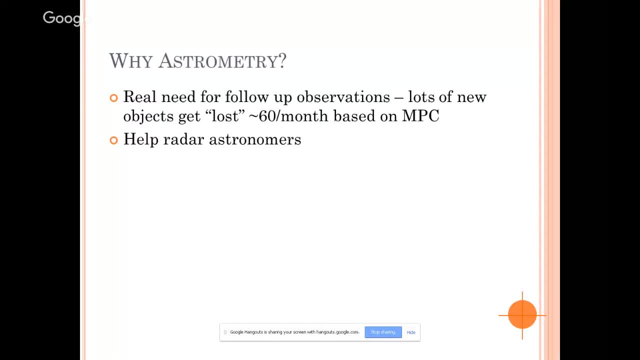 Anyway, the radar images. they need to be able to point their radio telescopes very accurately to get a bounce off of these things So good. astrometry helps them Also to refine occultation predictions. This is where an asteroid passes in front of a star and you get an idea of the true size of one of these things. 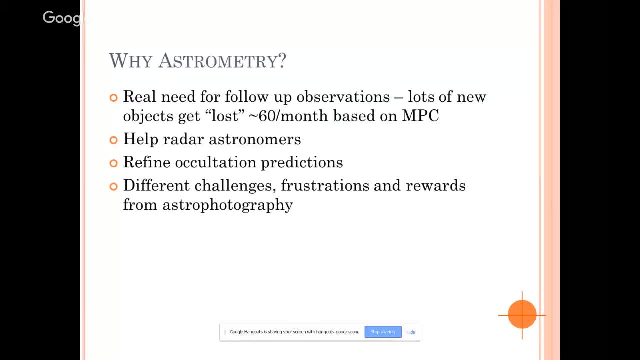 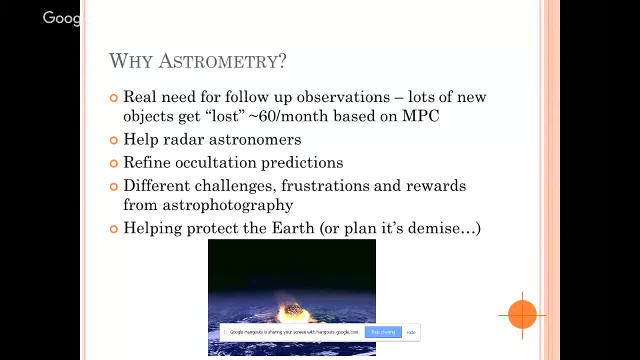 And I guess finally you can tell people that you're helping protect the earth or, I guess, planets' demise. That's always an interesting thing thing to bring up when you're at a social event and somebody asks you, what do you do? 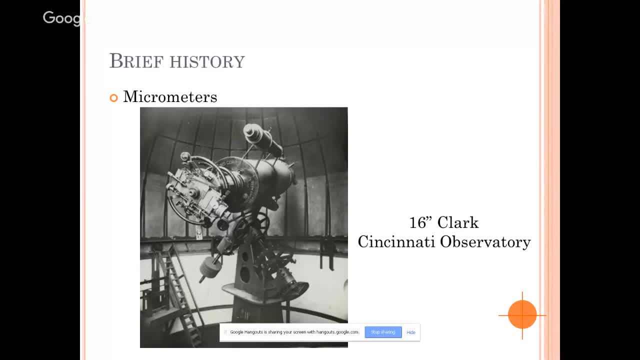 So a brief history. Before the days of film and photography, positional astronomy was done with mostly micrometers, And that's the thing you see here, attached to the end of a telescope. This particular telescope is a favorite of mine. It's given me many hours of enjoyment at the Cincinnati. 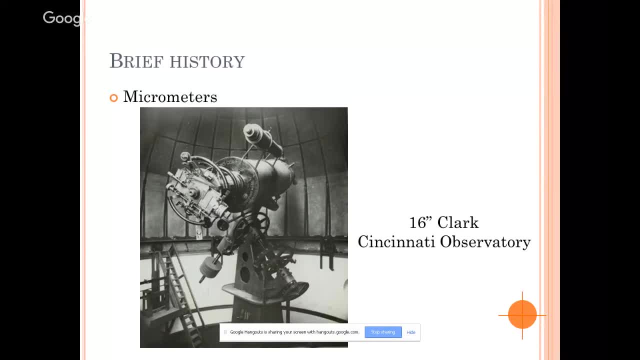 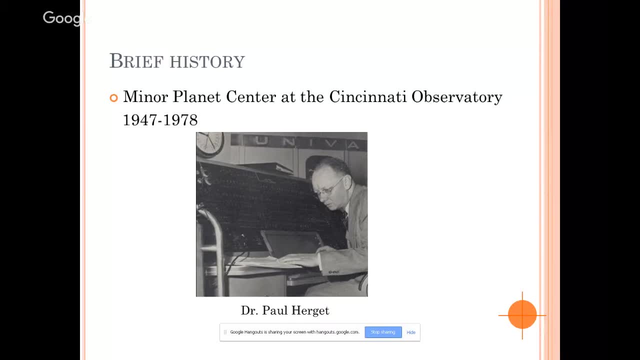 Observatory, although I've never looked at through it, with the micrometer tailpiece on there And an aside here, just total transgression for a second: The Minor Planet Center, which is the international clearinghouse for measurements of asteroids and comets, and the 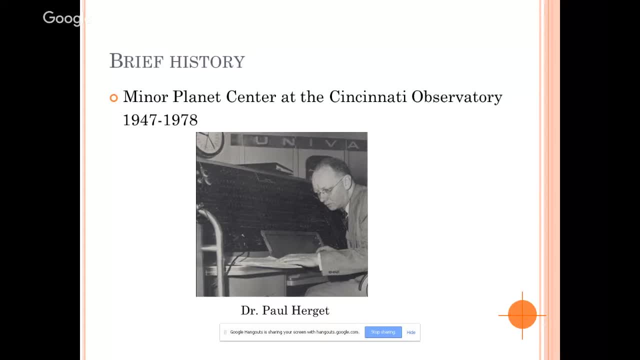 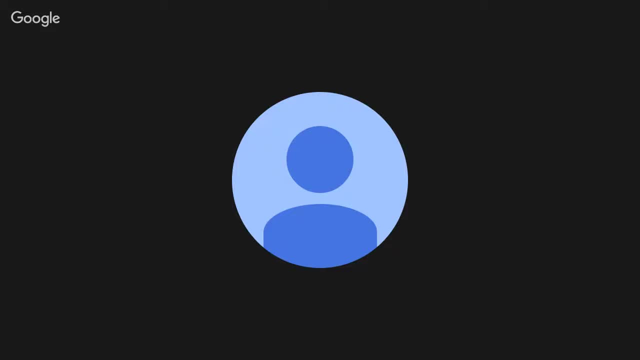 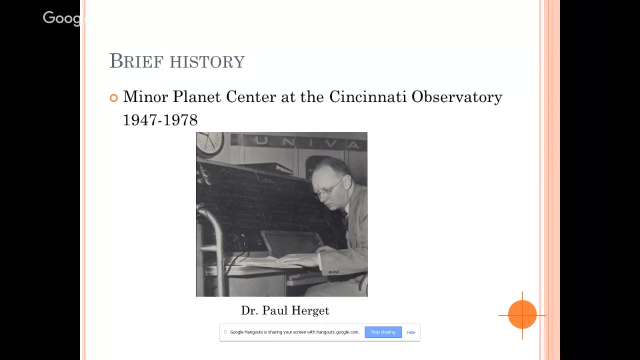 calculation of their orbits was at the Cincinnati Observatory when Dr Paul Herget was the director from the end of World War II until he retired in 78. And I'm sure his legacy me hanging around there. he was gone. I never met him, But his legacy is. 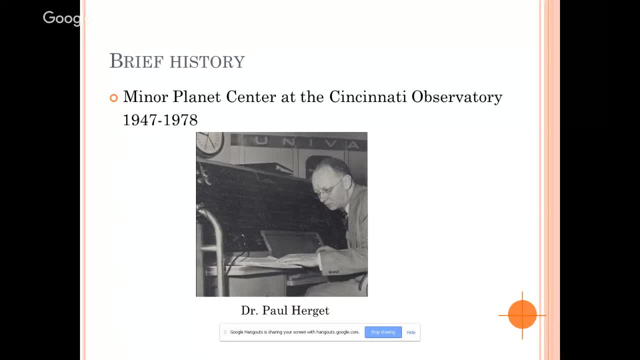 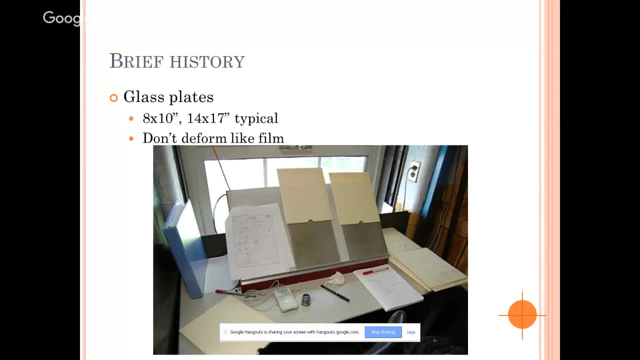 all over that place And I'm sure that has helped inspire me to kind of pursue this field a little bit. So traditionally you're talking about glass plates, typically 8 by 10 or so, And glass plates don't deform like film. Now, glass plates are pretty unwieldy, They're expensive, They're hard. 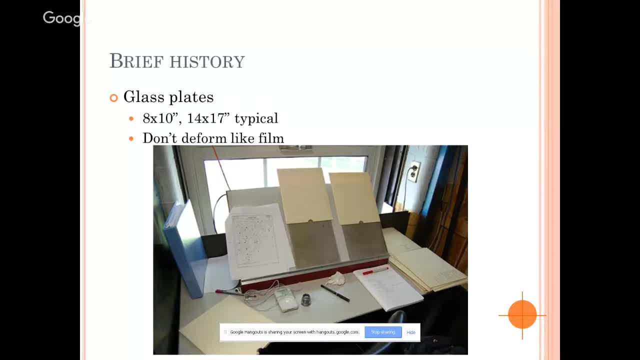 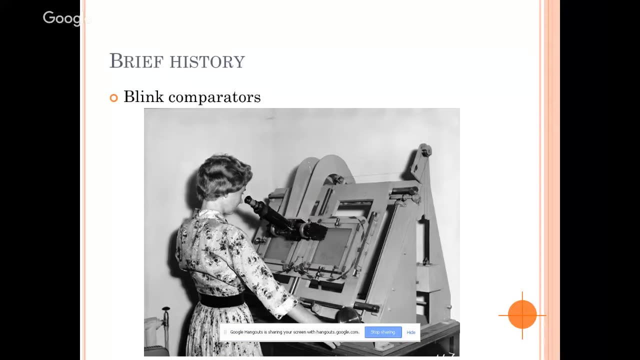 to get- And we're talking, you know, back in the day before the days of CCD cameras, And really something that amateurs didn't deal with. Then you needed something like this, a blink comparator, where you stick a couple of glass plates in there where they were exposed at different times And you go. 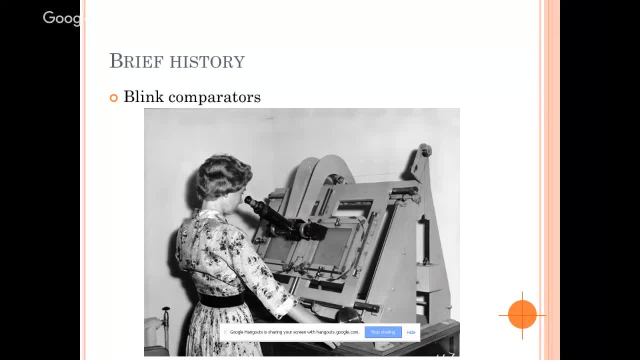 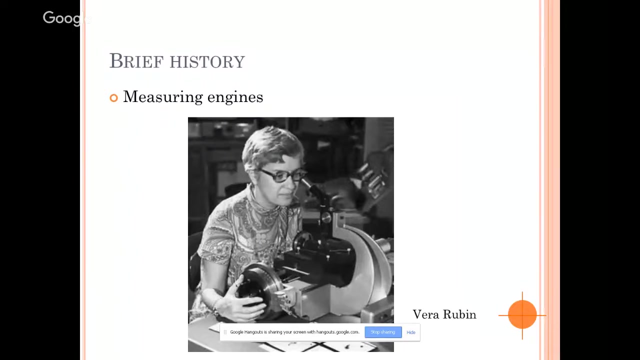 through the two images, blinking them back and forth, looking for things that move or things that change, And this şekilde unquote consumed. And you need something like a measuring engine This actually measures the positions on the glass plates to a very high precision, And this happens to be Vera. 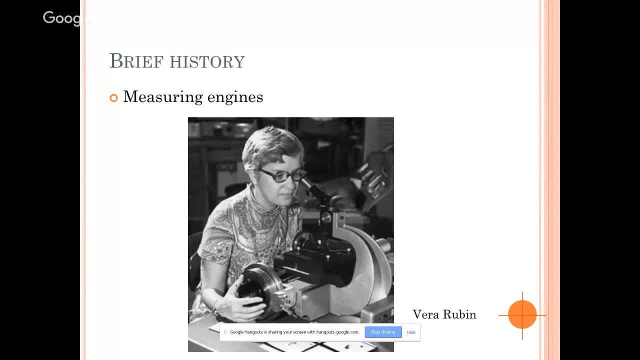 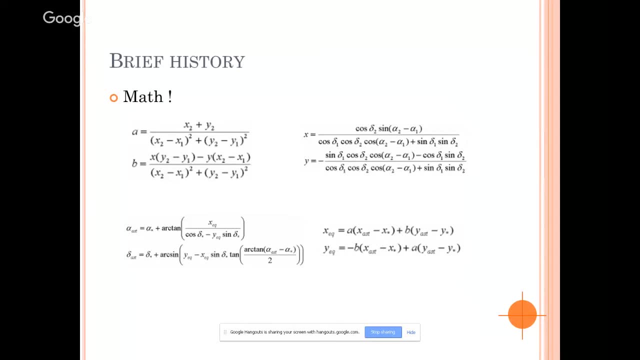 Rubin looking through one, Although she's probably looking at the spectra, obviously, of galaxies and not at asteroids or comets here and then, of course, you have math, um, lots of good math, and we're talking about math with a slide rule and log tables and trig tables. no pocket. 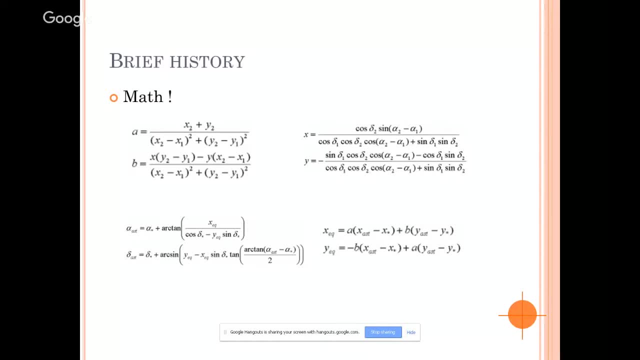 calculators available. uh, so that was you know another thing, and really this all kind of boils down to: there were hours of work to make one measurement, uh, and it's not really within the ability of amateurs and it, to be honest, it's not something that many professionals just wanted to. 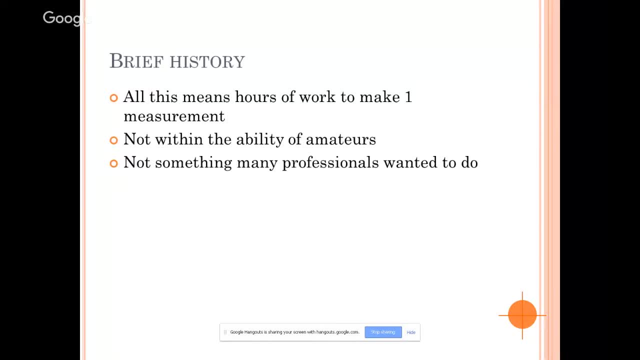 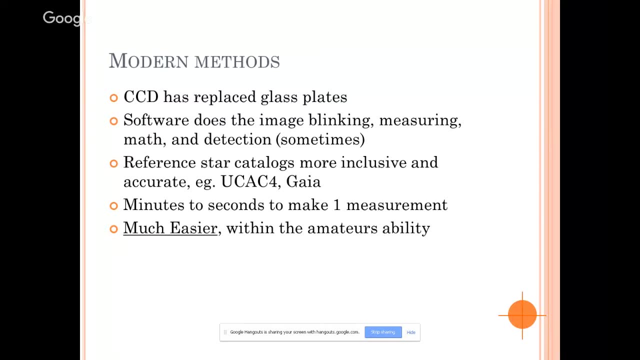 do. it was tedious, laborious and error prone. today, the modern methods, ccd has replaced the glass plates and the software today does the image blinking, the measuring, does all the math and it can do the detection automatically. uh, sometimes especially the robotic, the big robotic telescopes. 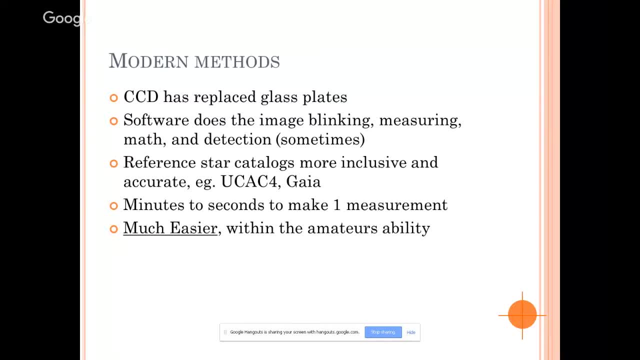 they find so many things on their, on their images. they have to have some type of automated process to to weed through all these things. um, another big difference today is the reference star catalogs. they are much better, much more inclusive. uh, the ucac4 and the gaia catalogs are are pretty much. 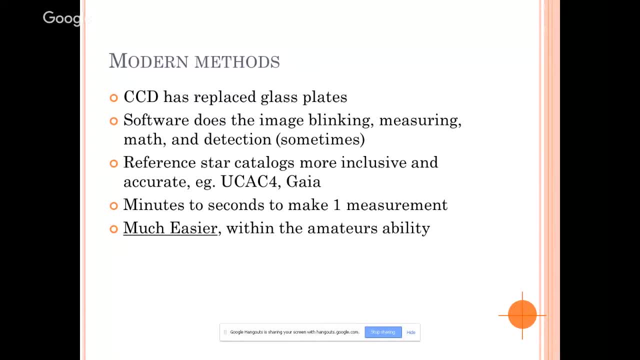 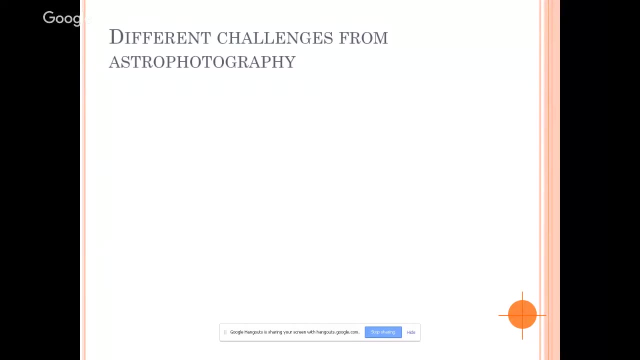 the standard now, um, and they are tremendous improvement over what was available. so it boils down to you have you know, minutes to seconds, to make just one measurement much easier, certainly within the, the amateurs ability. um, some of the different challenges that i see, uh, of course, the big one, i think, is, is you've got moving. 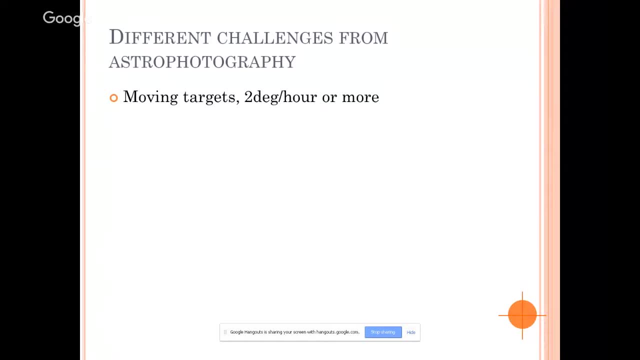 targets, uh, sometimes two degrees an hour, um, or more. when these objects come close to the earth, uh, that can be a real challenge. uh also the positions for the new objects, uh, are not all that well known, the, the orbits. when something is discovered, they kind of take a guess. a good. 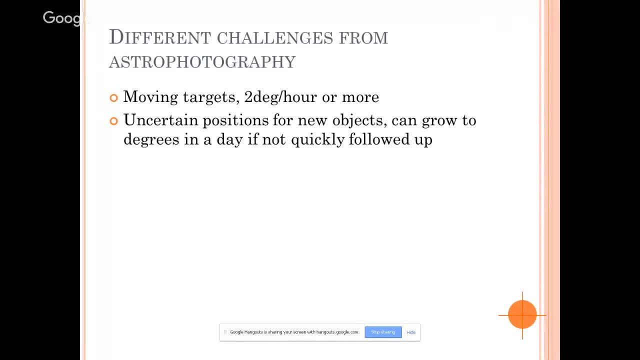 guess at the orbit, but if you don't get follow-up observations of that thing within hours, in some case, um, the the actual position can be off by degrees from where it really is. uh, so that can certainly be a challenge, and then these things vary in brightness. uh, the asteroids. 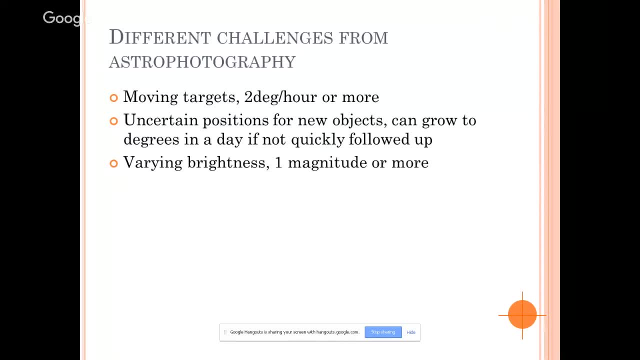 they rotate around and, uh, they're oddball shapes. so the brightness varies quite a bit. so sometimes it's brighter and fainter Comets. of course, when you're doing those comments pretty much do what they want. uh, you know, they can certainly be brighter or fainter than predicted. 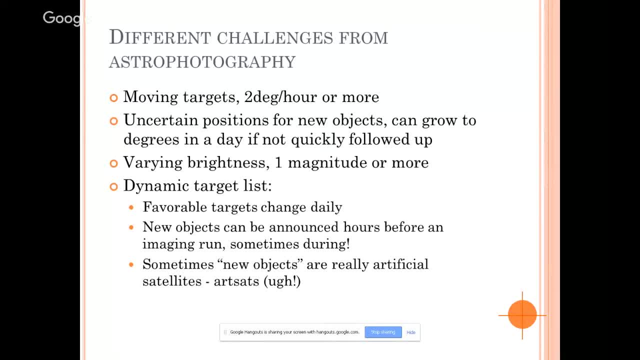 um, and I think you know there's a very dynamic. it's a very dynamic area there. the target lists are- they change daily really- uh, and new objects uh can be announced hours before an imaging run, sometimes during. I know, when I'm out taking images, I'm constantly. 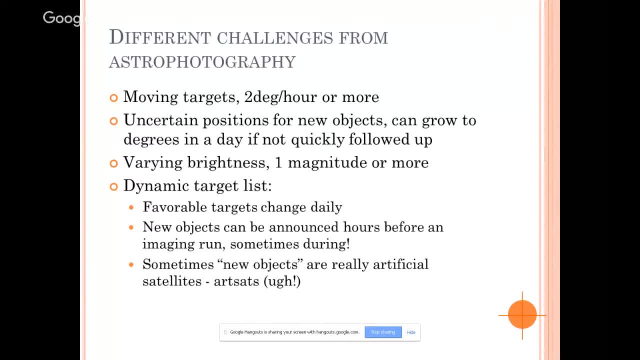 checking the, the website where new, new ones are announced, and, sure enough, several times one has been announced right in the middle of something, when I'm doing something, and I have to kind of switch gears, you know, on the fly, um, and of course, just to complicate things a little bit, sometimes new objects are really artificial satellites. uh, those 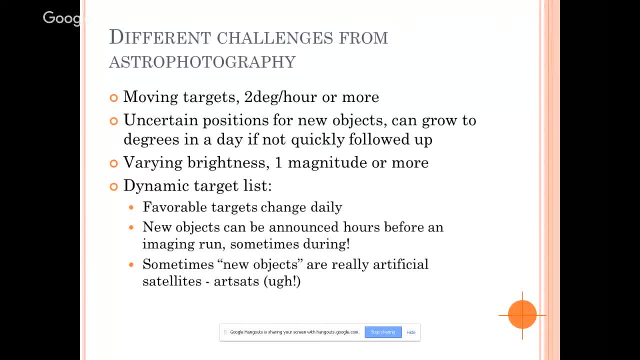 get in the mix a little bit. sometimes the, the big professional observatories, make a mistake and they announce: you know, a new object that's really a satellite. it doesn't happen very often, but it does, so that just complicates things a little bit. um so a little bit about the equipment and 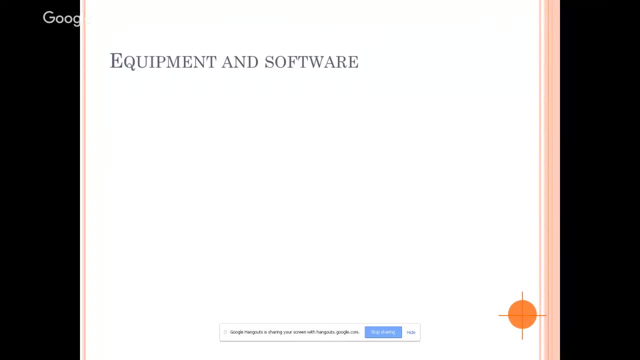 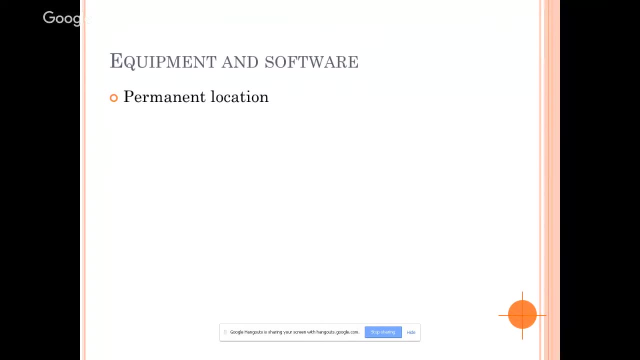 um, that's something that kind of the minor Planet Center, the place where you submit these observations insists on: all right, when we go through this, perhaps you know you'll see why that's really necessary. you also need sufficient image scale. um, you need a good enough image scale. 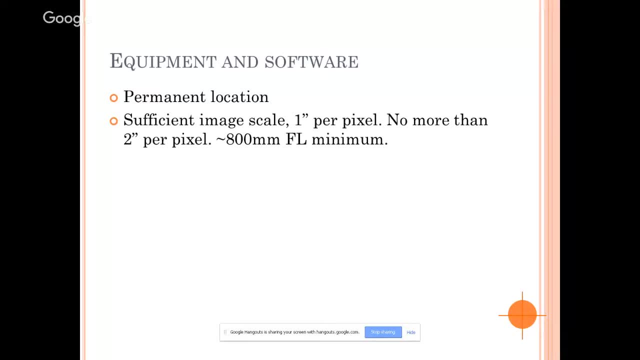 to get decent measurements and basically, uh, one arc second per pixel. uh, it's pretty good. you don't need to get anything uh greater than that or a finer resolution than that, but you don't want to get anything more than about two arc seconds per pixel and I quit. 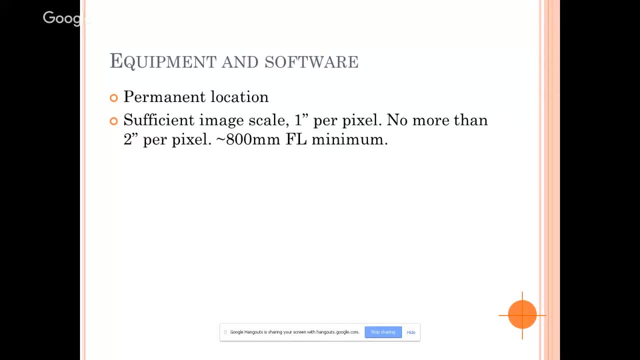 800 millimeter focal length minimum. I just kind of based that on the- uh, the pixel size of some of the common cameras that are out there today. uh, that's just a ballpark. um, you know, back in the day you needed longer focal length to be able to measure the positions on the glass plates to a sufficient. 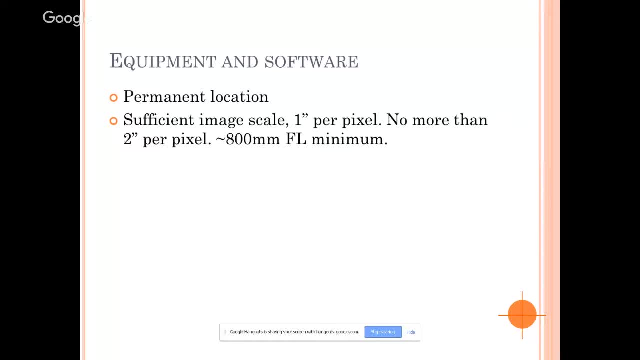 accuracy, But today 800 millimeter or more is probably sufficient. You also need a relatively decent field of view. This has also changed greatly As the star catalogs get better. you really don't need- and this is my recommendation- maybe more, at least 10 arc. 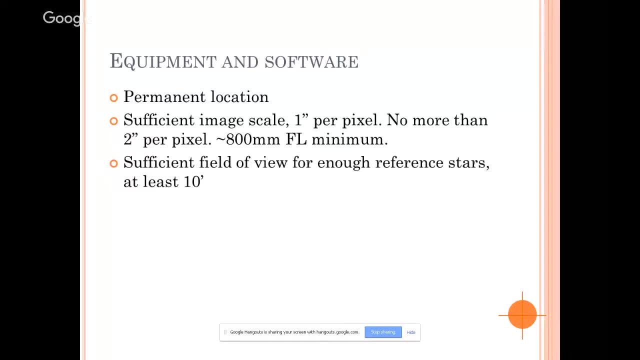 minutes is probably sufficient to get enough reference stars in the image so that you can get an accurate measurement over pretty much anywhere in the sky. Of course, larger the field of view the better, And also a high quantum efficiency CCD helps, And that's because you. 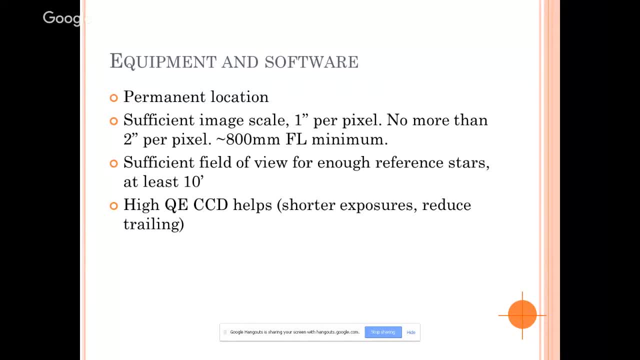 can get shorter exposures. That's kind of the bottom line here is: you want to get these things with the shortest possible exposure to reduce the trailing that they produce as they're moving Astrometrica software. you got to have it. if you're going to do this, It's really the only. 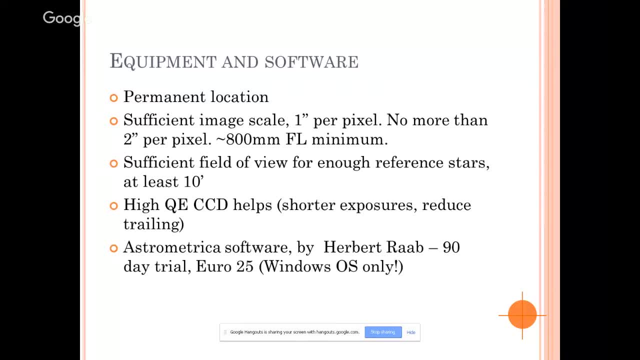 way to go. It is a nice package. It's only 25 bucks a euro, There's a 90-day trial And unfortunately it's only Windows, But you really have to have that. You also need to have some program that syncs your PC's time to. 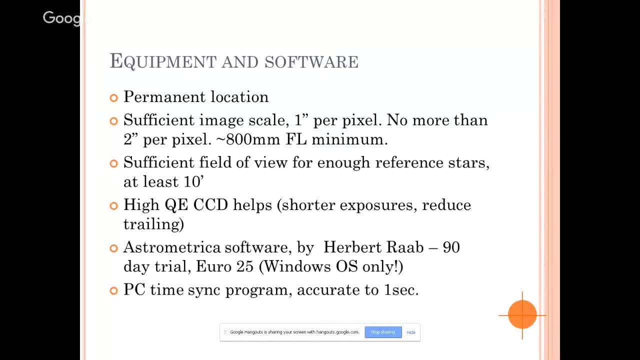 one-second accuracy. There are several freeware programs out there that do that, But when you take your images and you send in your measurements, they really require that the measurements be made to a second of time. accuracy. And, finally, you need some kind of post-processing. You don't. 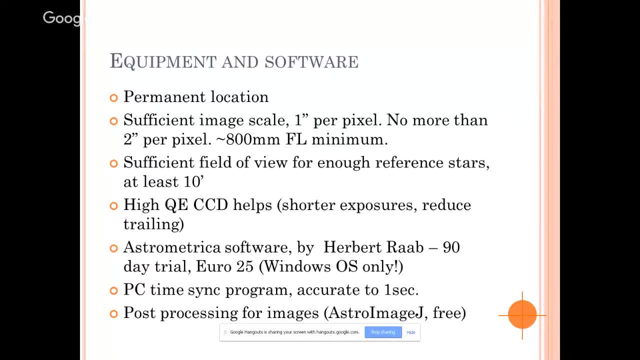 really do a lot of post-processing. You're going to have to have a lot of post-processing. You're going to have a lot of post-processing. I use a program called Ask for Image Day. I like it a lot. It's free. 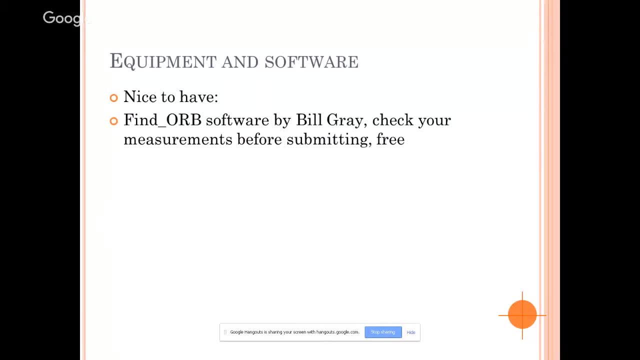 Some of the nice to have is a program called Find Orb And again links to all this stuff, all these programs and all the websites that I'm going to go through here. I've got them at the end of this presentation And I understand Adam's going to make this. 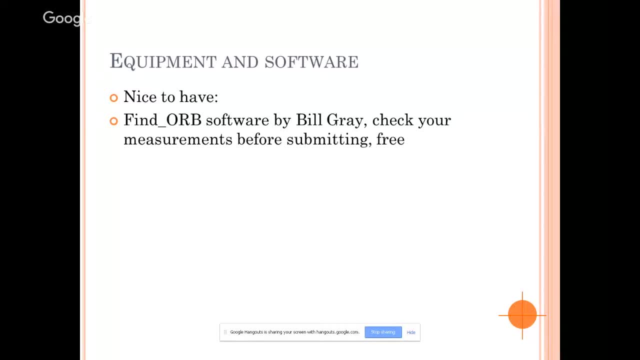 presentation available on YouTube. So that's another reason why I'm going through this quickly, Because you'll be able to download this and take a look at it at your leisure. This program lets you check your measurements before you submit them- Another helpful one that 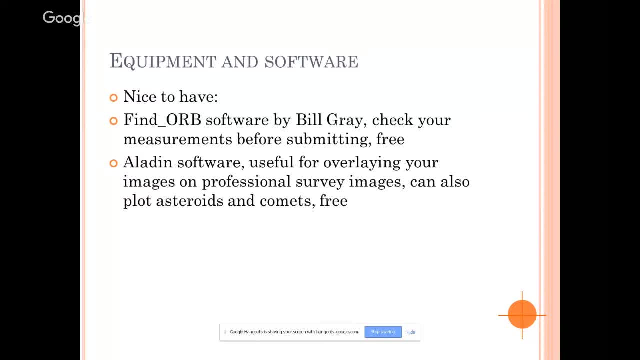 I've used is a program called Aladdin. I find it very useful for overlaying my images over survey images, to kind of see what I'm getting in my images. It can also plot asteroids and comets. And then the program I use is a program called Car2CL. I imagine probably a lot of you use that. 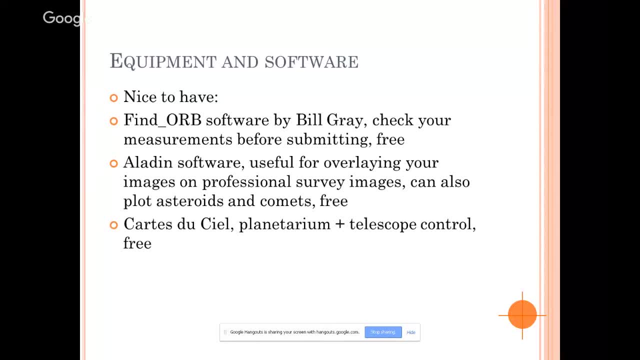 I like it quite a bit. I've gotten very comfortable with it. It controls the telescope. I use it to calculate the positions of these objects, And it's free. And there's another program that works with that, written by the same author. It's called CCDCL. It's in beta, But I use. 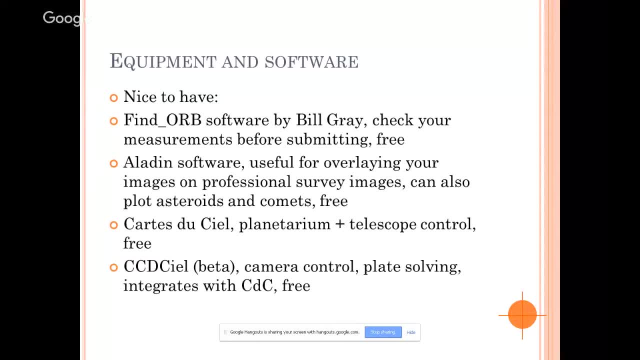 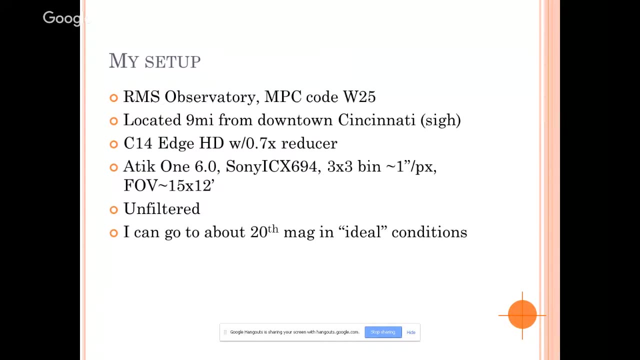 it for my camera control. It does plate solving, It integrates with Car2CL And it's free And it works pretty well. And again, I've got some demos in my screencast that actually show you how I go through this and how I use them. So my setup: Well, I've got a C14 Edge with a 0.7 degree. 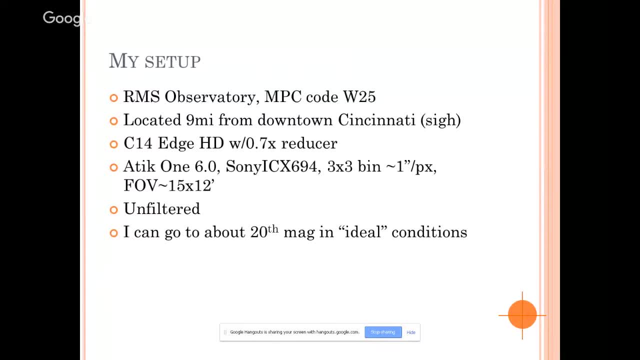 square on it And my camera has got a Sony sensor. At three by three binning I get about almost exactly one arc second per pixel And my field of view is about 15 by 12 arc minutes- No filters. I use it unfiltered And I can get to about 20th magnitude on a good night in quote. 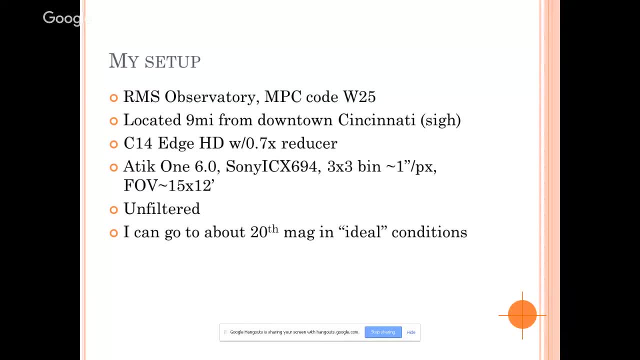 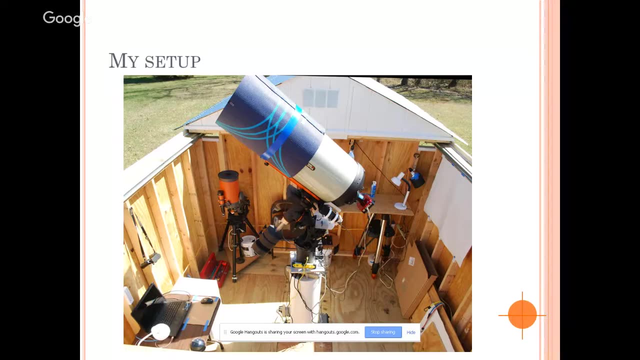 unquote ideal conditions because I am located nine miles from downtown Cincinnati, So I've got a fair amount of light pollution I've got to deal with. This is just a picture of my setup. I actually just built this observatory last fall. After being interested in astronomy for 45 years, I finally got around to building this thing in my 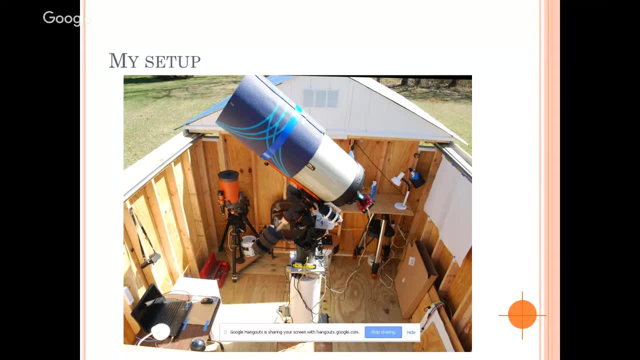 backyard: buying a new telescope, buying the camera. You can see my little C8 in the background there. It's just a 10 by 10 shed roll off roof. I know you guys like looking at gear, So here's my gear. 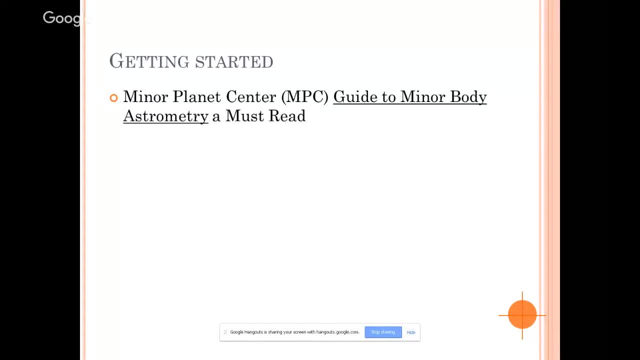 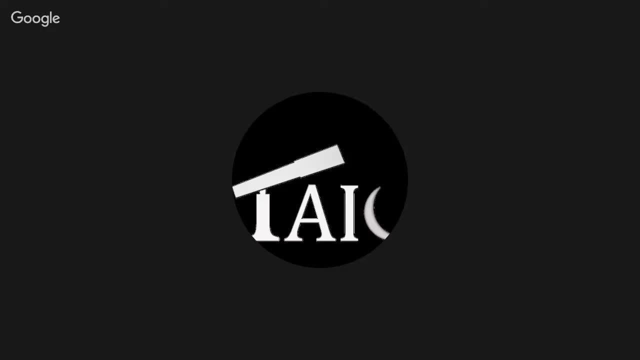 Before I get going in here, Adam, we got any questions popping up? You've answered the questions as they come. Of course, people are asking: what scope mount are you using? and you just answered it, So keep doing what you're doing. 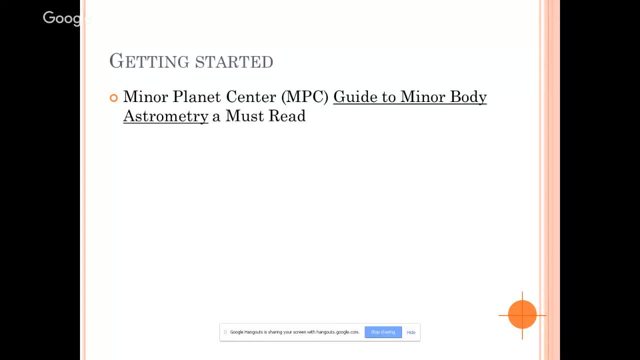 Great. So to get started, if I haven't scared you off by the end of this or put you to sleep, you really- I think the best place to start is this guide to minor body astronomy. This is really a must read, And if you want to go further, start with this, And I'll just leave that there. And again, there's a link to this at the end. 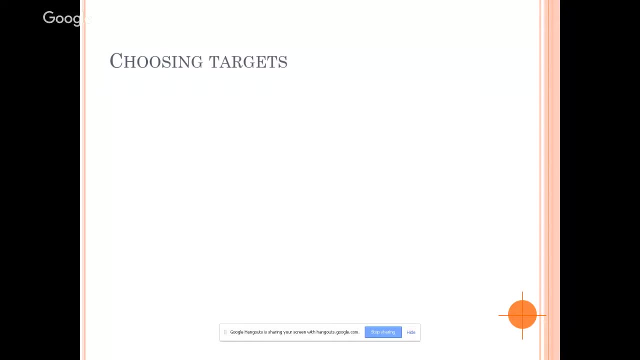 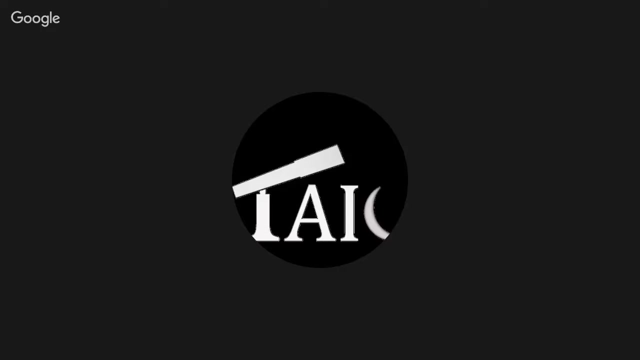 So, talking about choosing targets, How do I do it? Well, this is how kind of I do it. Of course, the greatest need is for targets with poor orbits. That's kind of the bottom line here, Basil, Yeah, Yeah. 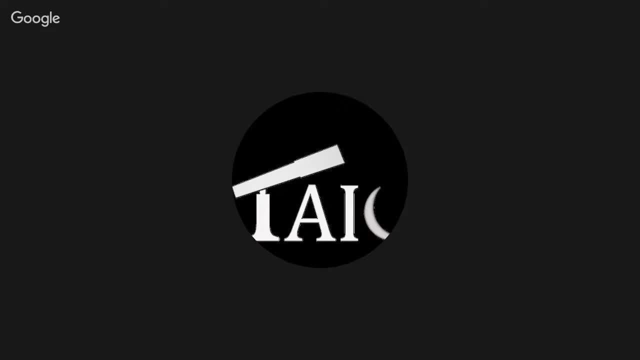 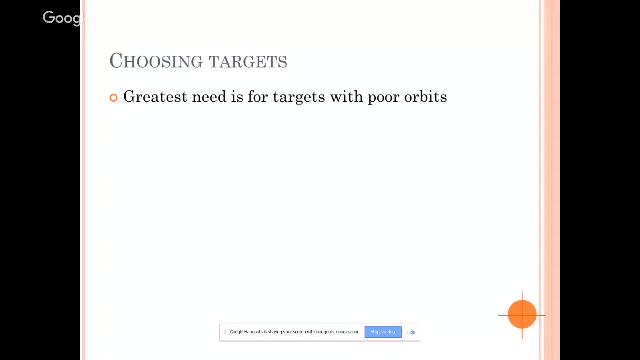 Yes, One question in regards to your observatory. I might as well ask now, Sure, What is your MPC observatory code? Ah, W25. Awesome, Thank you, Mm. hmm, So the ones with the poor orbits are the ones that you really want to try and focus on, And there are quite a number of those. So what I do is I start with the Minor Planet Center web pages, And there are several of them. 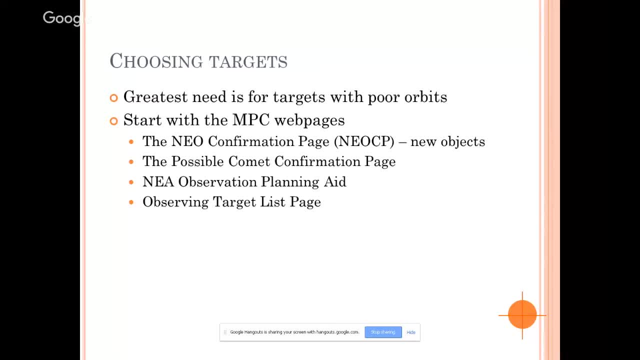 And I'm going to quickly go through them. I have some screen captures of them. The one that I refer to a lot is this NEO confirmation page. That's the one where all the new objects are announced. That's the one I check several times during the night. 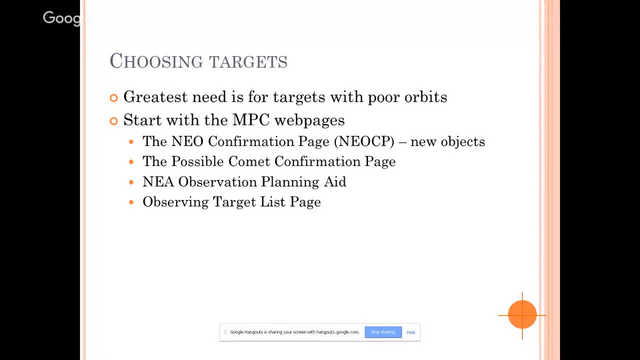 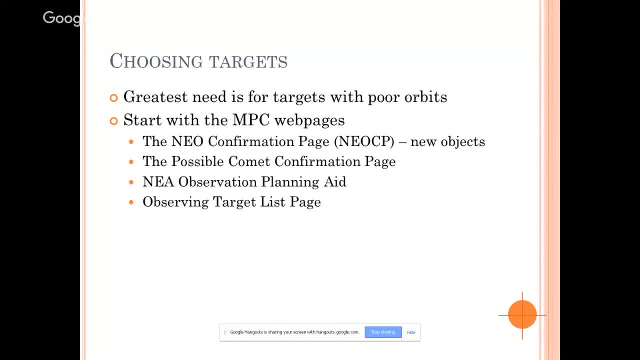 And then there's the one that I refer to a lot. Now, this is an actual a point that I and I looked at this development function of the NEO presentation manager, of all the other podcasts yet to have a platform where they can get to us. 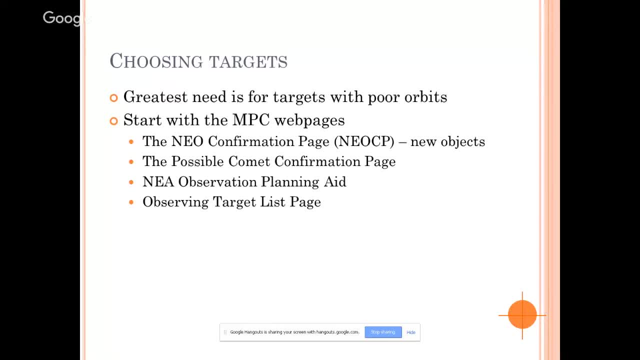 Simply, as you can see, mykeltag is now called this cptrell- теперь先设成用来设定几个文件. questa locator前采访呀, hebdicios自己提供和我广告. 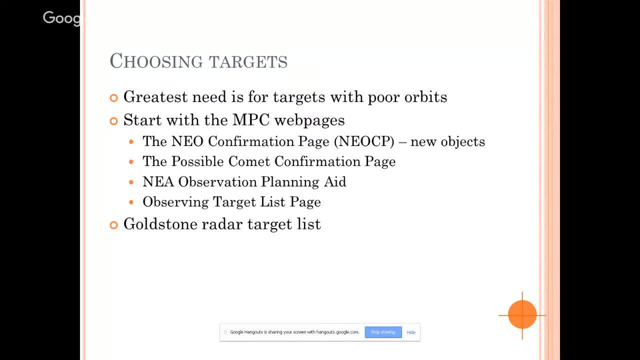 And if they look fuzzy then they move them to the other page. And then there's a couple of other ones. There's a planning aid and a target list page. that are the last one there. I used to get comet cometary objects. 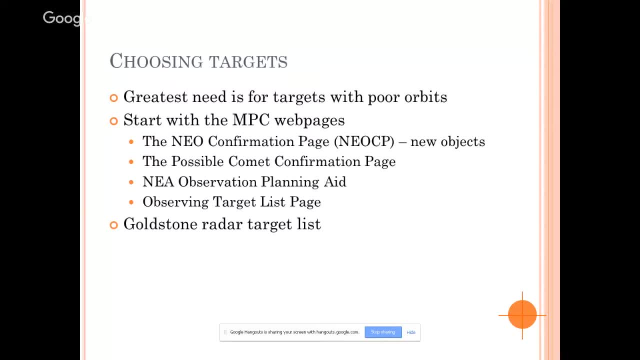 And then there's a couple of other ones. There's a planning aid and a target list page that are the last one there. I used to get comet cometary objects to image or target, and sometimes the ones on there can be different than the ones that the 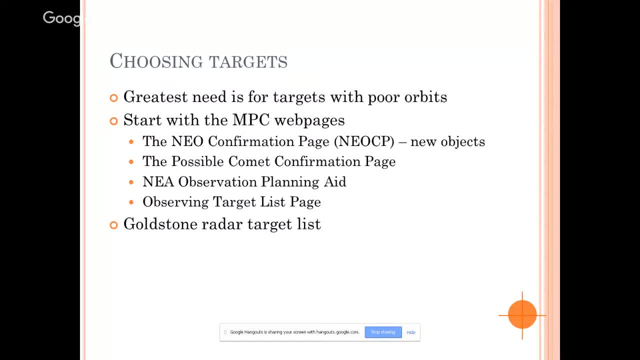 minor planet center, uh thinks you know need orbital refinement, um. and finally there's a. there's an esa. uh, there's a priority list there. it's very similar to the minor planet center. it's just kind of another place to check. um, i kind of use this as a kind of double check sometimes. 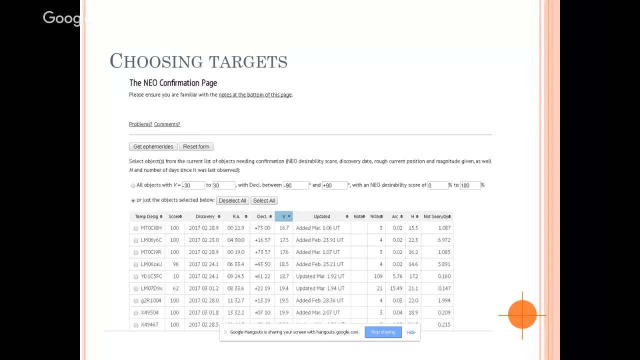 um, so here's the the uh neo confirmation page. uh, from the minor planet center. this is where the new objects come out and i'm not going to go into a lot here. uh, if you want to see kind of how i go through this, that's just in one of my screencasts, but you know, basically what i do is sort them by. 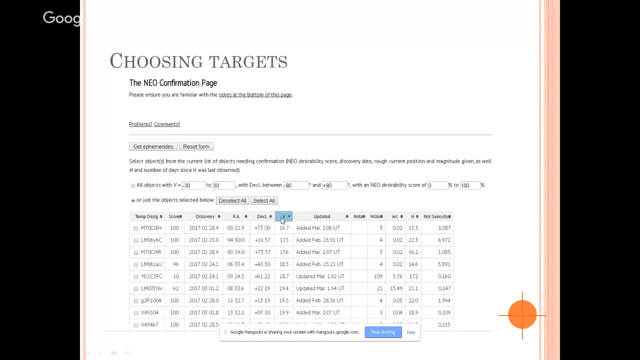 by magnitude, first to give me an idea of what i can get. and then i check the declinations to see if i can get them, uh, and then i get on the list here and i see, well, okay, how many observations have there been and how long has it been since they've been seen? and in this case, uh, you know these first one. 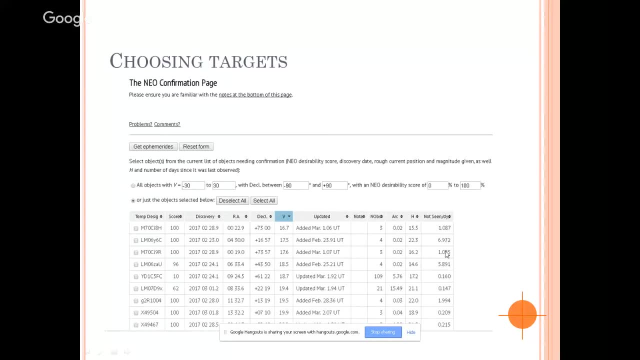 two, three, four objects, uh, having not been seen in this length of time, they're all probably lost. so all the bright ones here, and the fact that they're so bright and haven't been seen is a good indication that they are lost. so in this particular list, the first object that i would 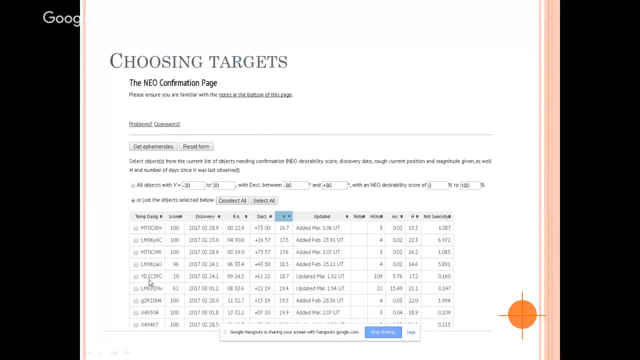 probably try for is this one here, this yd1c5 fc, uh 109 observations it's been recently seen. next one also, and then the rest of these are probably lost. so already you know these guys are gone um and you can set various constraints here about declination um. 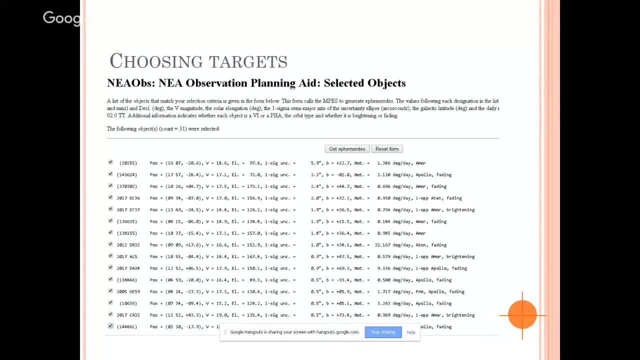 that this page is is a listing from the minor planet center where you can get objects. uh, there's a page before this where you fill out a form and you can set various parameters like declination and and minimum magnitude, uh, and some various other things, um, and i just go there. 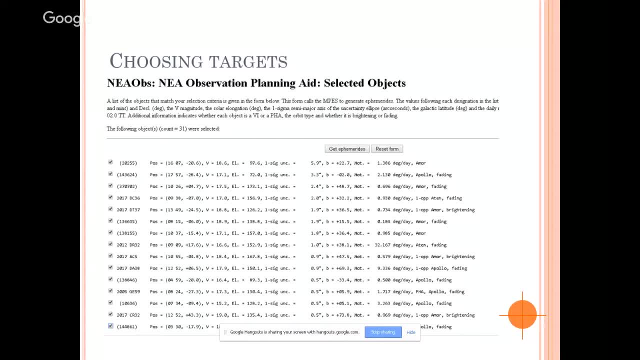 fill out the form and brings me here and it shows me. these are the objects that have preliminary designations, or numbered designations, meaning that their orbits are fairly secure. um, and some of these will not need further observation to refine their orbits. uh, you know, looking at this, this, i have them sorted by the error that they have in their 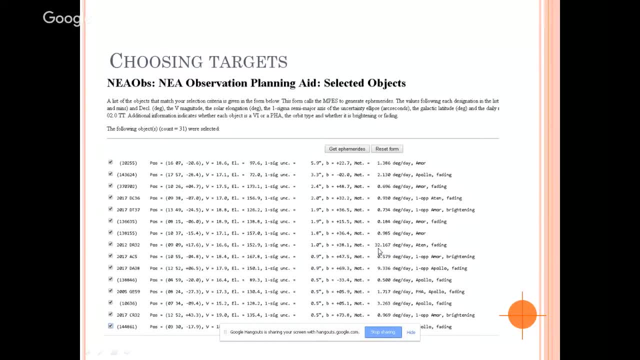 positions. uh, you can also see here. here's somebody that's moving it at 32 degrees a day. um, that's going to be one of those fast movers. uh, so this kind of helps me. you know plan uh for for some observations. um, what i do is i click on get ephemeris and that produces a list of objects. 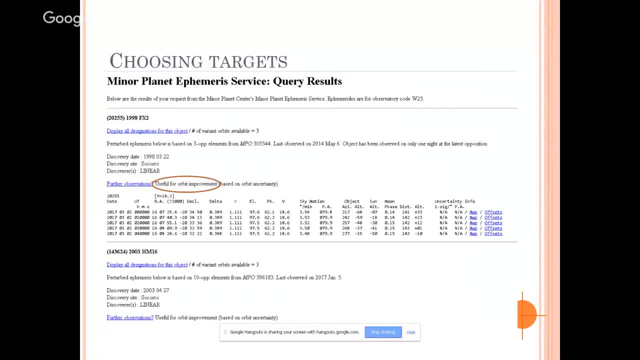 i just grab them all and i go through the list one by one and i look for this, this useful for orbit improvement. here's this first object on the list, and basically what i do is i create a text file of all of these objects that i want to target and i basically just copy and paste the name into the 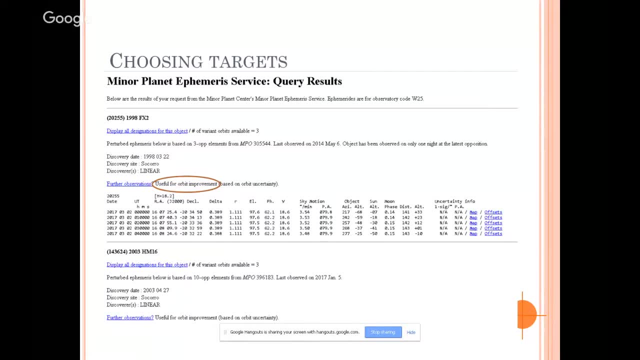 text file and i go through the list one by one and if i see useful for orbit improvement, i check some other things down here about how far away from the moon is it and things like that, of course. how bright is it? um, and i just go through the list one by one and if i see useful for orbit improvement, 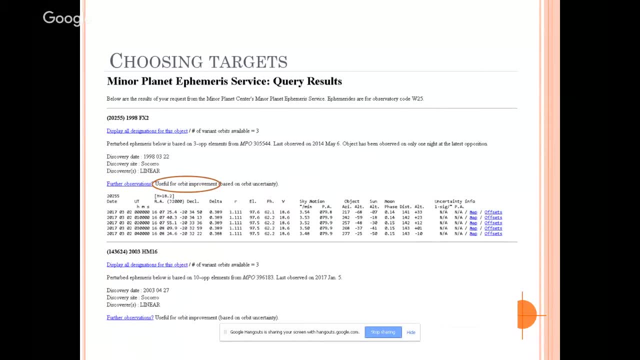 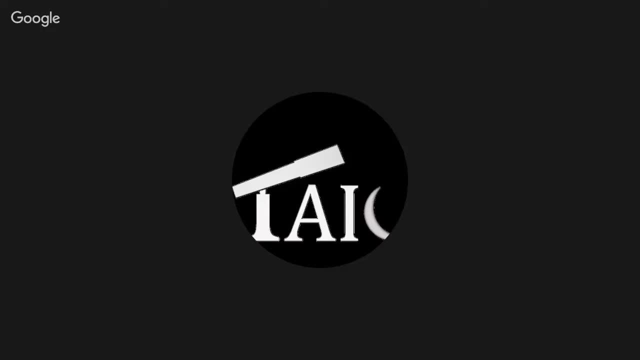 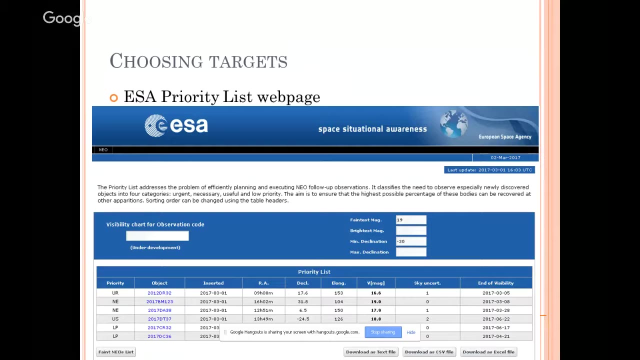 then i add it to my list, whether i get to it or not, as another issue: basil. one more, one more question. yes, do you do any measurements for the target asteroid project? uh, i don't think so. um, i believe i've. i know what the person is asking. 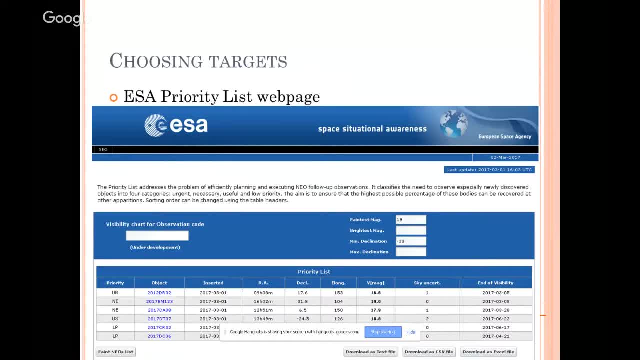 um, i've seen that and that is another kind of- uh, i guess, avenue to to go, if you want to, you know, get a list of objects, uh, to target. i think they might be interested in sending spacecraft to those, more so than refining their orbits. uh, i think that's what it. that was uh. 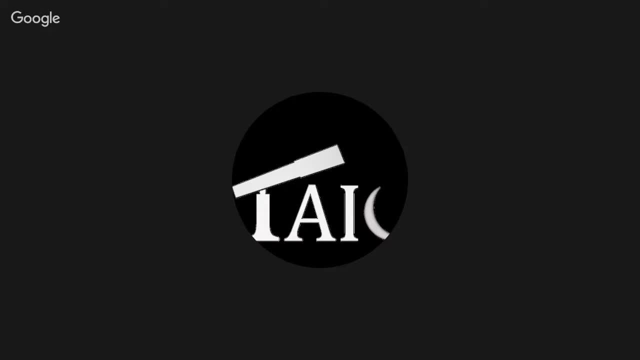 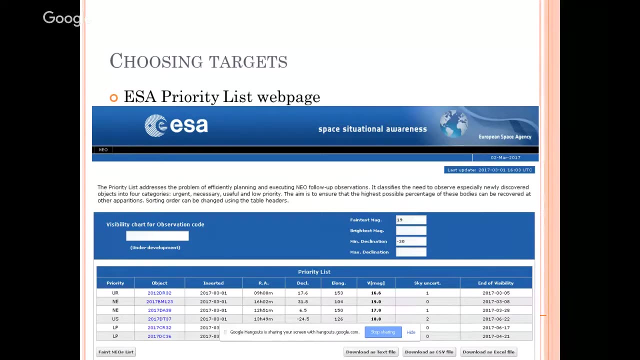 for the flyby study of venue. yes, i was commenting on, so that sounds right. yes, yep. no, i've never, i've not gotten involved with that. um, i don't think they're really planning any future missions to asteroids, uh, so i don't know how active that is these days. 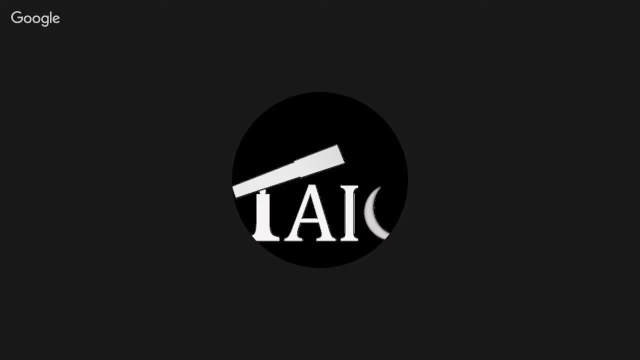 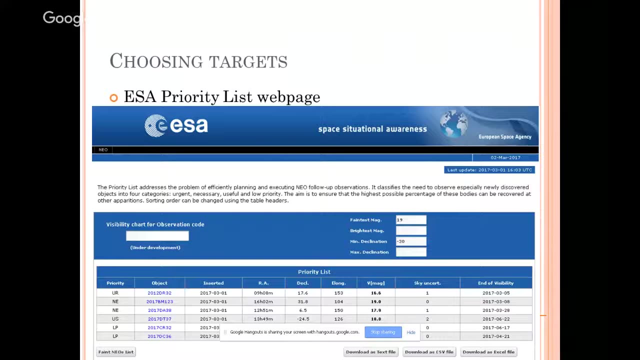 okay, and can i ask one question? um you your uh from a particular slide. now it disappeared on me, but uh you uh had said earlier, your goal is in general, to refine the measurements, or the error. i should say so, unlike i think it was two slides before it showed. 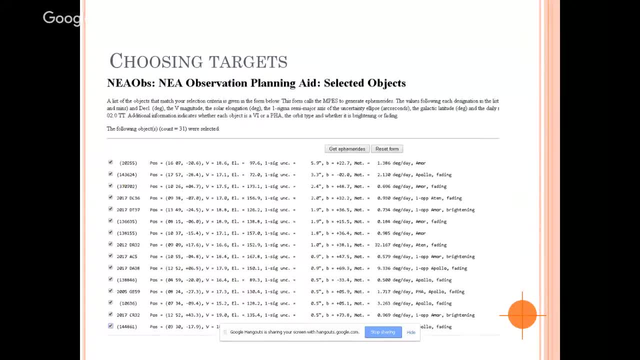 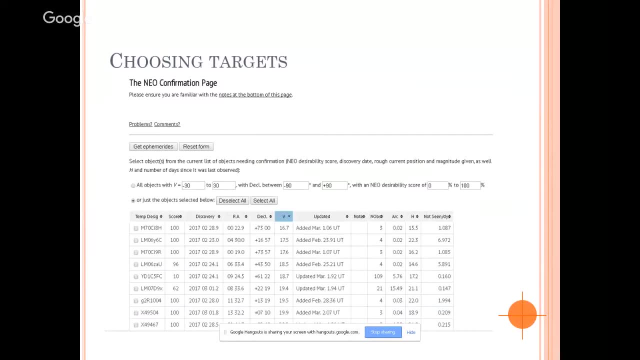 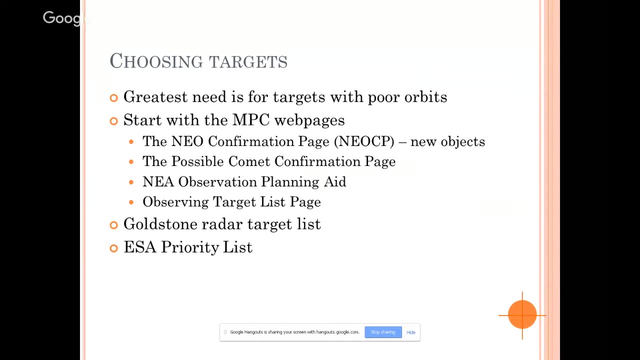 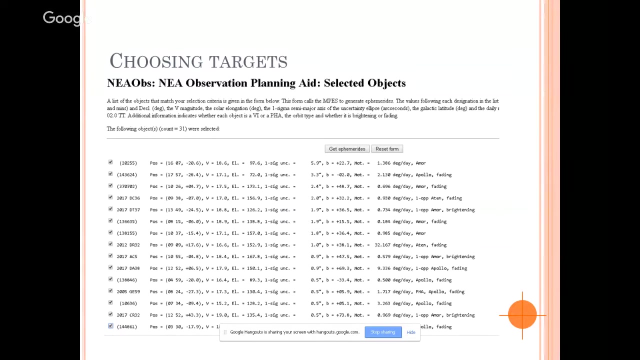 in. uh, what did it say, man? Maybe one more slide back, if you don't mind. Where did I see it? No, it must have been – I thought I saw something that said error or positioning error, And your goal is really to refine that positioning error, right? 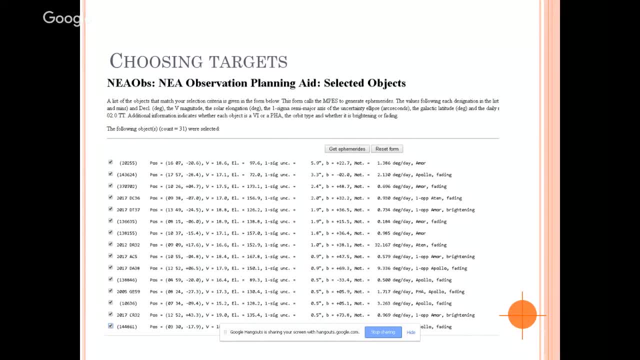 Yes, I mean that's the goal for the Minor Planet Center is to pin down these orbits better And, in this case, to reduce this error that you see here in this column. That's kind of the goal here for the Minor Planet Center is to better keep track of these things. 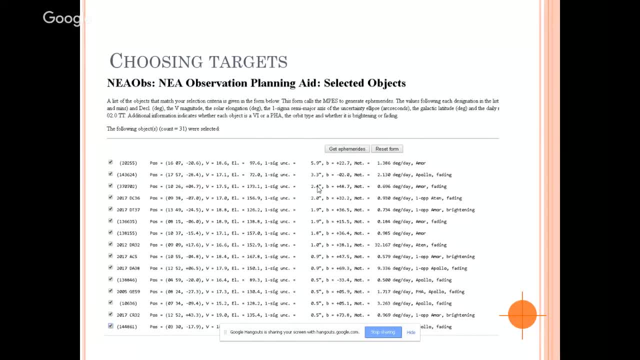 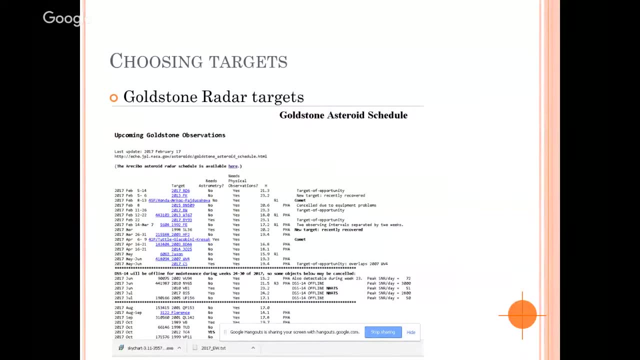 Okay, That's my question. Thank you, Sure. Sure. This is a grab from the – This is the Goldstone Asteroid Schedule, And the column here that we would be interested in is the one that says: need astrometry question mark. 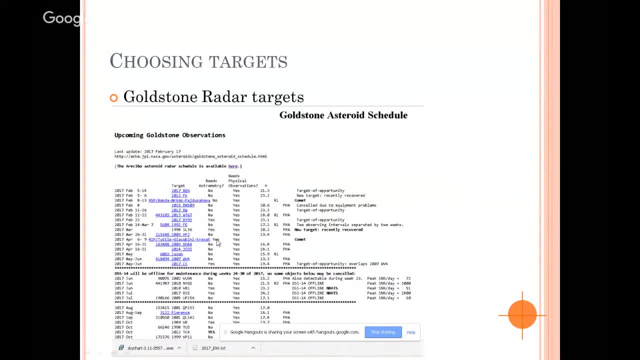 And you can go down here and you can see here's a comet that they're looking for astrometry on, And they go pretty far out into the future here. I think they even go into 2018.. Of course, this list changes. as you know, near-Earth objects get discovered. 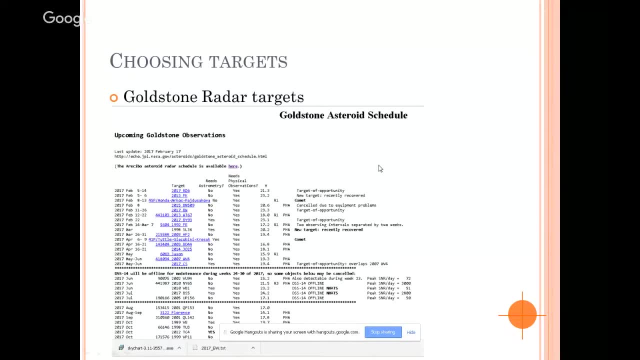 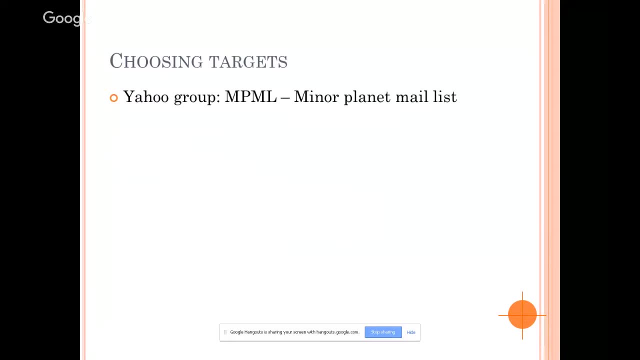 But this can be another source to help Get objects for your target. And finally, there's a Yahoo group that is a good one to subscribe to the MPML. A lot of professionals hang out in there. Sometimes I hear about new things there before anywhere else, or things that kind of fly under the radar. 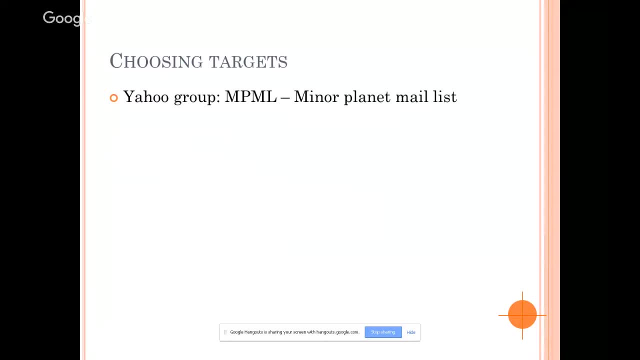 No pun intended, So that's a good one to subscribe to. Okay, That's pretty much it for choosing targets. Again, I got a lot more kind of – I go through those websites in more detail on some of the screencasts. 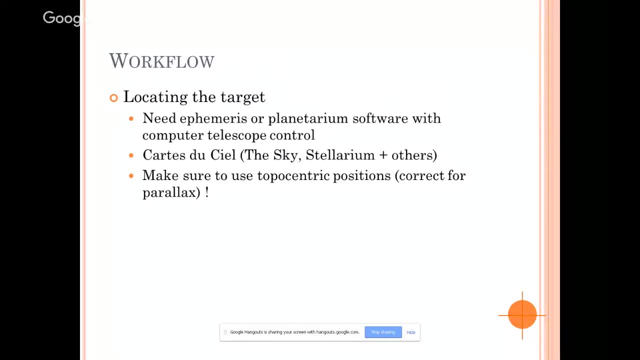 On to the workflow. Well, the first thing you want to obviously do is locate this target, And in order to do that, you need some type of ephemeris for this target, or today, it's going to be a planetarium program with some type of computer control. 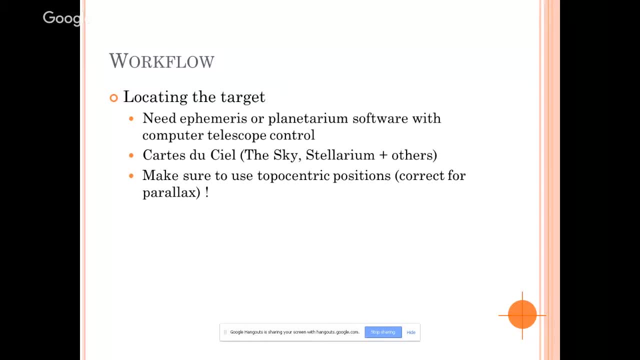 I said I use CartusCL. The Sky does this, Stellarium does this. there are others that do this Because I use CartusCL. I'm going to talk about that one a little bit. The important thing to remember is, whatever one you're using, you need to make sure you have topocentric positions set wherever that gets set. 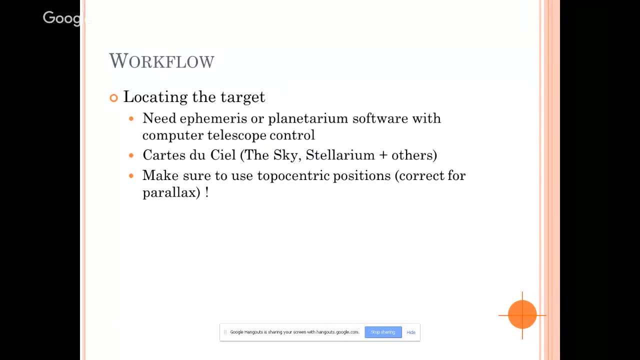 You have to correct for parallax. Is these things – if these things – is this a parallel? No, it's not. It's a parallel. That's the way it's supposed to be. So, that's the way it's supposed to be. 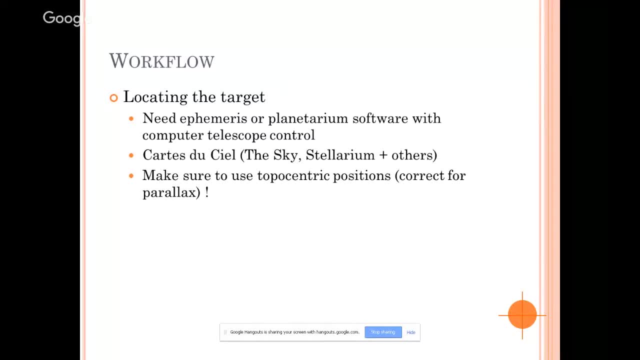 That's the way it's supposed to be. So that's the way it's supposed to be. So that's the way it's supposed to be. So that's the way it's supposed to be. these things come close to the Earth. you're you're positioned to be off by a degree or more if you're not correcting for parallax. 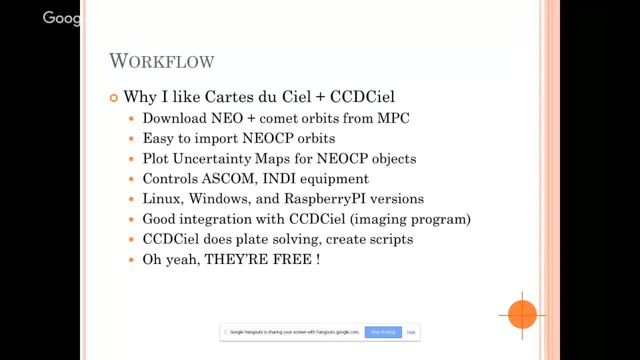 That is super important. A little bit, I guess, of a commercial for CART2CL- although I don't get anything from this in CCDCL, but one of the things I really like about this program. it does a lot of stuff, but for what we're talking about, you can download the comet and NEO orbits directly from the Minor Planet Center. 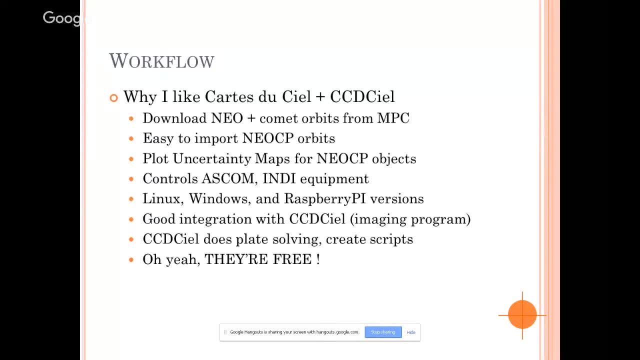 and it's easy to import the NEOCP orbits. Those are the new objects. Getting those orbits into CART2CL is a little. you have to go through a little bit of a process, which I talk about in one of the screencasts. 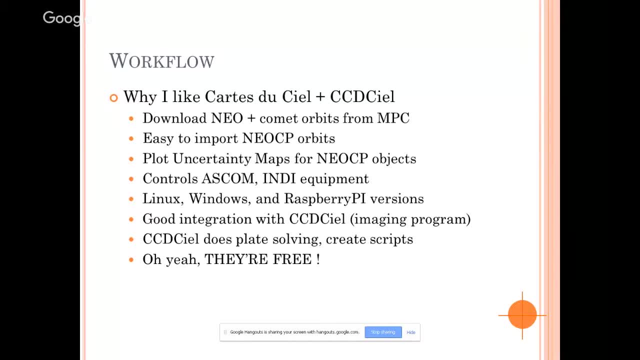 but it's pretty easy. It's easy to do. I don't know if- and some of you if- someone out there knows the sky, which I think is also an excellent program and I know does a good job, and I know a lot of people use it to target asteroids and comets. 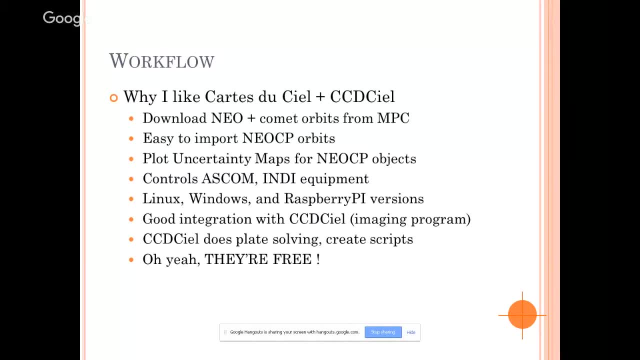 but I don't know the sky and I don't know if the sky can grab the NEOCP orbits or if there's an easy way to get those in there. So if someone out there is the sky guru and has done this, I would love to hear from you. 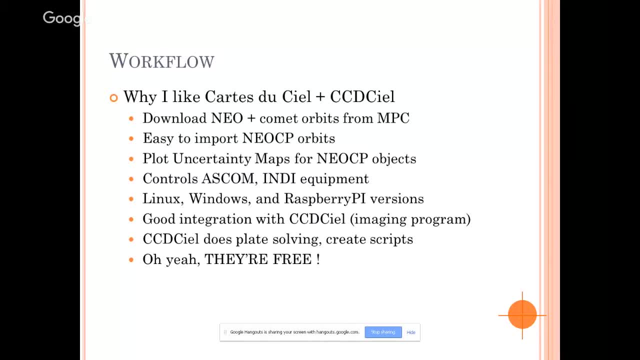 I would love to hear from you. I would love to hear about that. You can also plot something called uncertainty maps in CART2CL, which we're not going to talk about. It controls ASCOM and India equipment. There's a Linux, Windows and Raspberry Pi version. 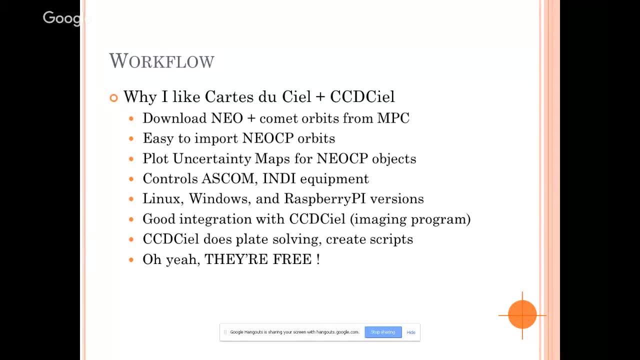 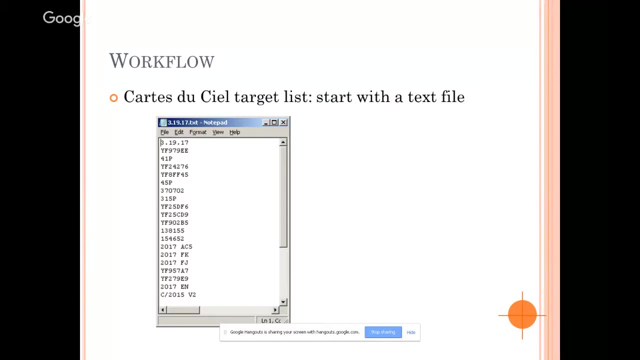 It has good integration with the imaging program written by the same author. CCDCL does plate solving and you can create scripts and run scripts and of course perhaps one of the best things is they're free. So here's kind of remember. I said we create, I create a text file first. 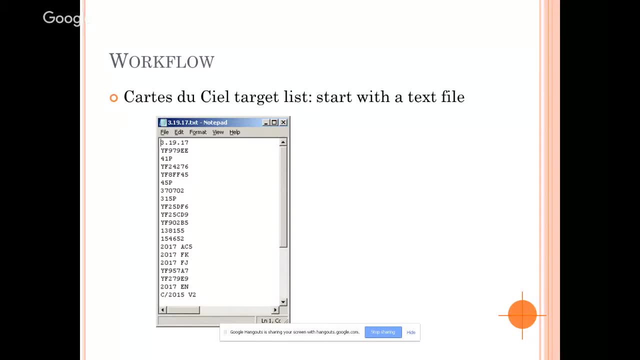 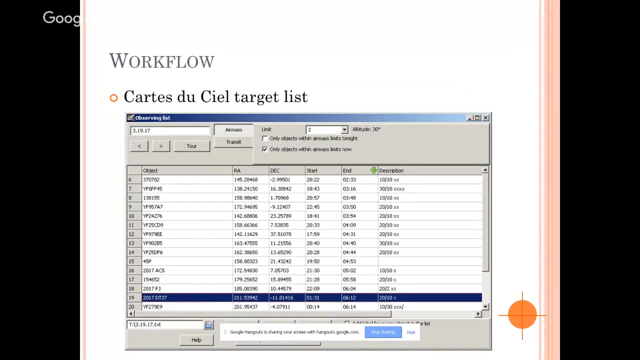 Well, here's a sample text file that I've copied and pasted all these targets for tonight or through the night of the 19th of March, and this is what I'm going to bring into CART2CL. When I load it into CART2CL it gets you get something like this on its observing list page: 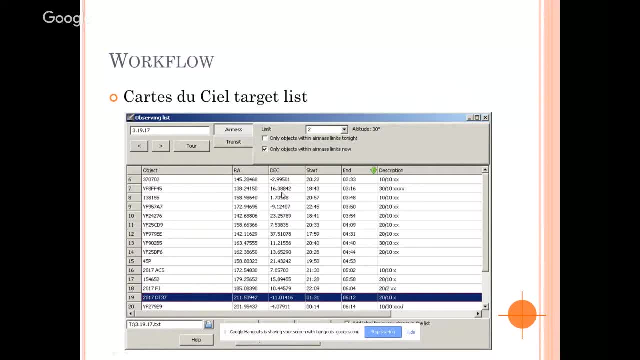 and I'm not going to go through a lot of this stuff, but I think you know you get the idea of what's going on here. You know I've got it sorted to show me only objects that are above 30 degrees altitude. 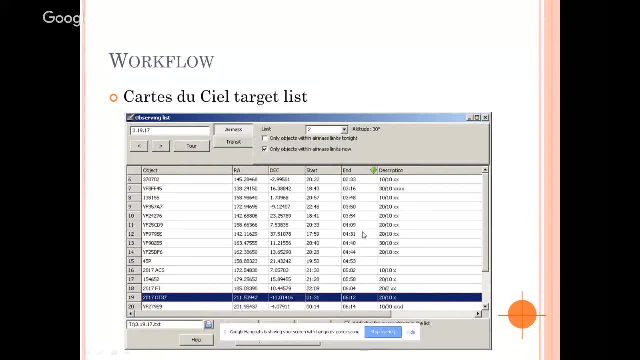 so I just kind of go down the list here and start imaging, and what I've found very helpful is over here in this description column I record a couple of things. I record first the number of subs or the number of exposures I've taken and the time for those. 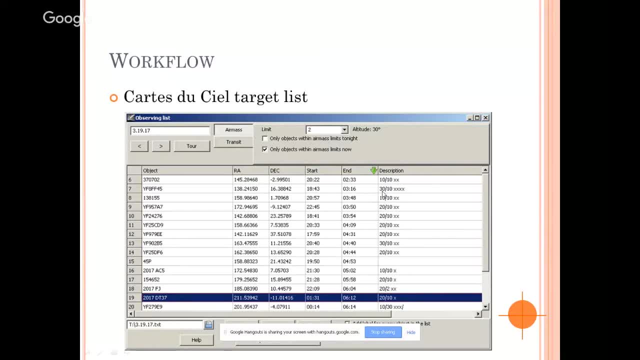 So this would be, you know, 10 exposures at 10 seconds, 30 exposures at 10 seconds. here's 20 exposures at 2 seconds. This one must have been moving really quickly, and then I put a little X down here to indicate. 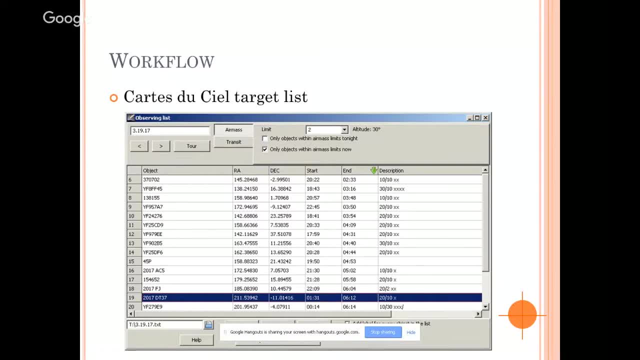 that I've completed one set of observations. When I talk a little bit later about submitting these, the Minor Planet Center insists that you have at least two observations per night per object. so the ones with the little two X's are ready, assuming I got them. 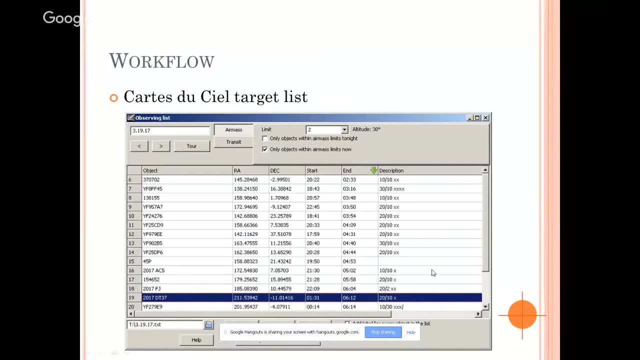 Here's one where I did four sets of observations. Here's a couple where I've only got one set and I need to come back and do these. so you know, as I get going through these and it gets late at night I cannot remember how many subs. 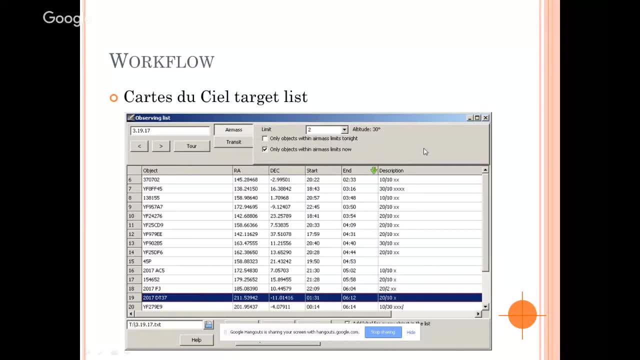 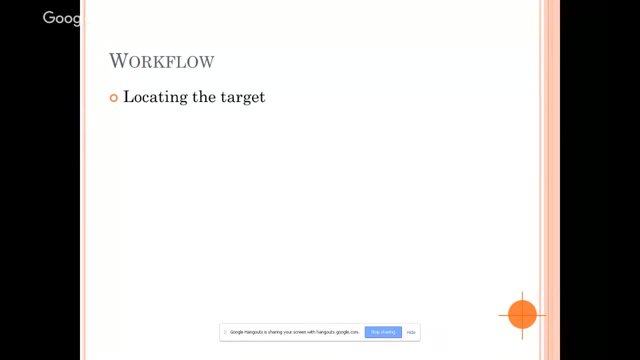 and how long? and is this my first set or my second or third? So I find recording this type of information someplace is really almost essential. So here's kind of how the workflow glows and I think you kind of know how this goes. 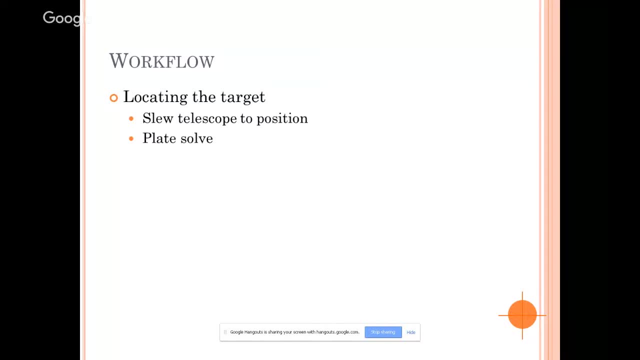 You locate, you slew the telescope to the position, you do a plate solve, you sync the telescope, then you do a repeat slew. if your telescope isn't pointed sufficiently well, Then you do another plate solve and hopefully by then your telescope is pointing exactly. 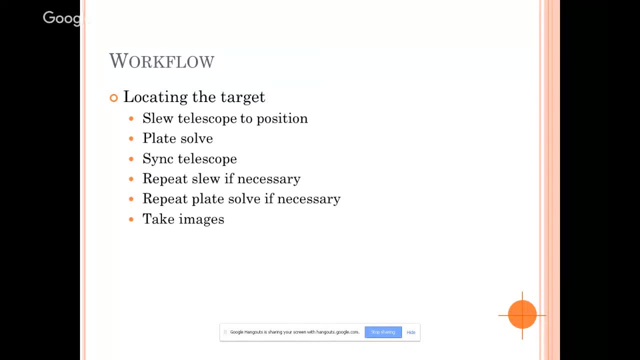 where you want it to be. Of course, if you have one of those expensive mounts that points exactly where you want it whenever you move it, that's great. I don't have one of those and you take your images, except if the thing is moving fast. 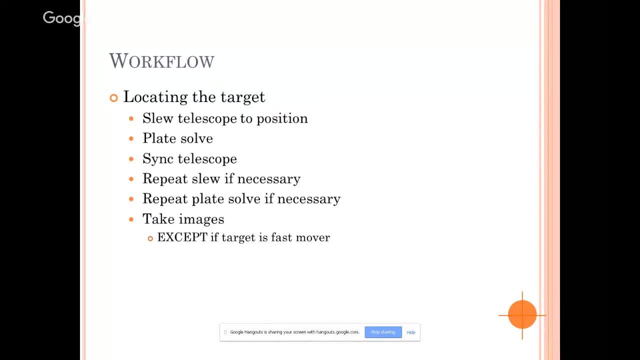 Here's kind of what happens to me when I try and target a fast mover. So here's this object moving in this direction And I tell my telescope: OK, do an initial slew and center the object in the frame, And you think that's what you get. 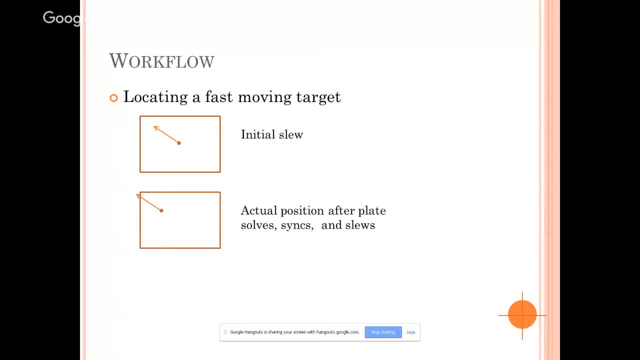 Well, by the time it's gotten there and you've done the plate solve and you've done, in my case, another slew to fine-tune the position, the object has moved pretty close to the edge of the field. So I've got to come back here and do a little fine-tuning and manually move. 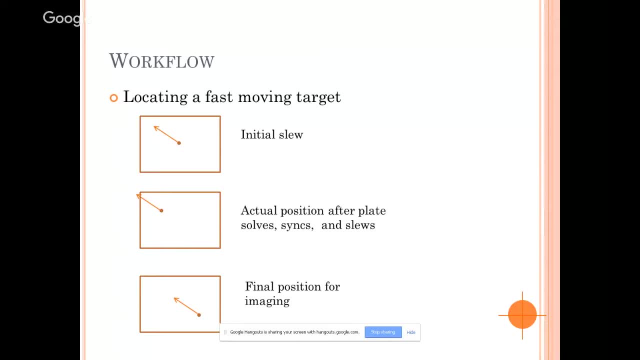 So I'm going to move the frame so that the object is somewhere down near the other corner, so that it's going to move through the field of view as I'm taking my images. So this is kind of where you're chasing things around the sky. 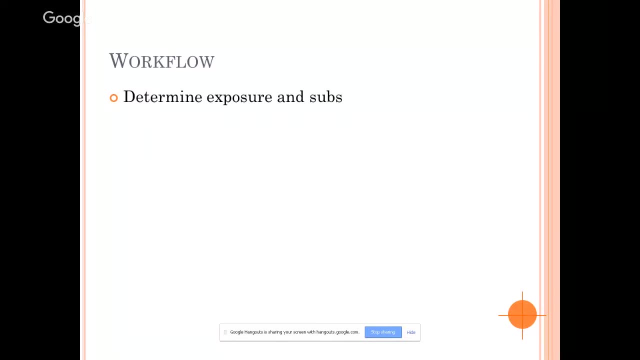 The next thing I need to do is determine: OK, how many subs am I going to take and what's the exposure going to be? Basically, the bottom line here is: you don't want the target to trail too much, So there is a lot to do. 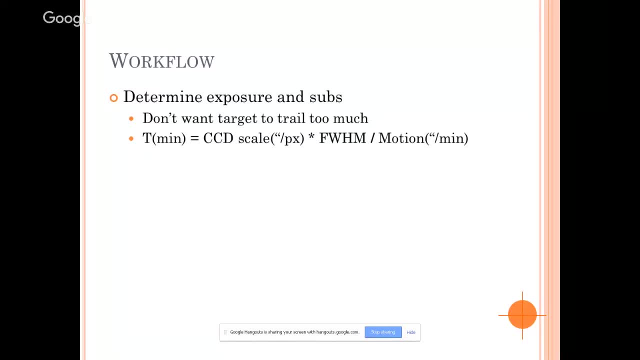 There is a formula that I found- This is the only formula I've got tonight- And it relates the maximum length of time in minutes to your CCD scale and your full width and maximum of your typical seeing and your star images and the motion. So I have an example. 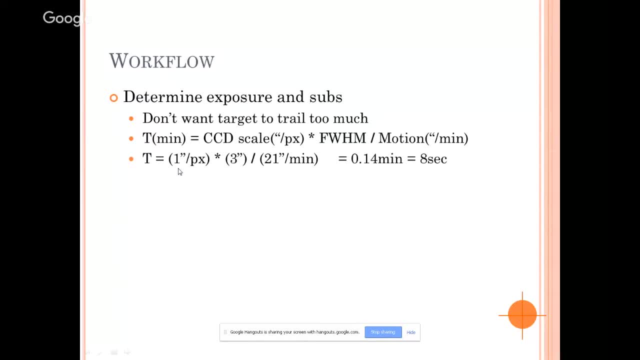 In my case, my image scale is 1 arc second per pixel. My good seeing is around 3 arc seconds. So that's FWHM, that's 3.. And let's say the object is moving at 21 arc seconds per minute, which is pretty good. 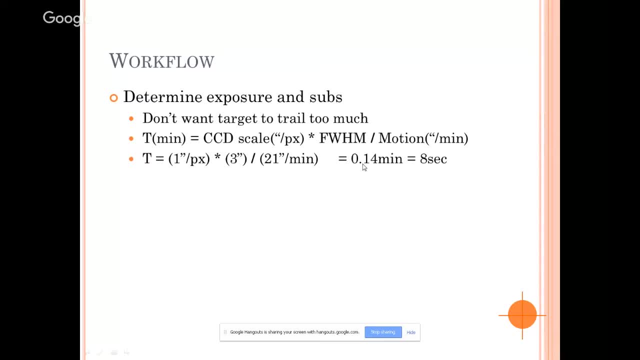 You run through the numbers, my exposure time would be .14 minutes or 8 seconds, Anything longer than that, and the star or the asteroid is going to trail noticeably and it could you know, you know, stop, Be problematic for the measurement. So in this case I would probably do five second exposures. 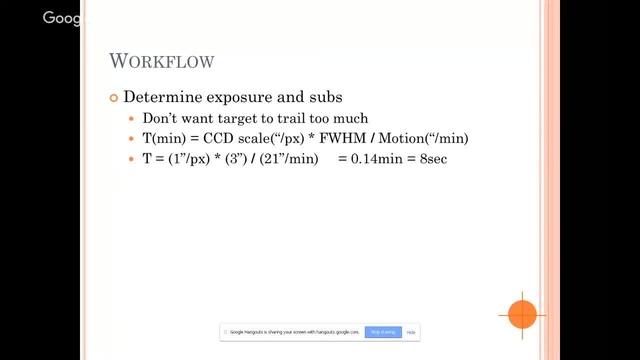 Okay, so how faint is this thing? and and how many exposures do I need To get it? How many five second exposures, again, keeping in mind shortest exposure possible? Well, I need to adjust the number of subs to reach the desired magnitude, and there's. 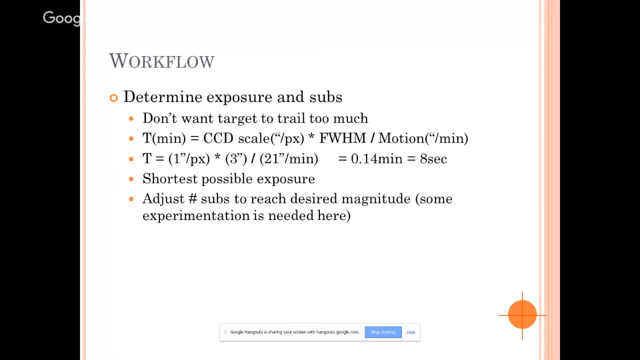 You need just to do some experimentation here. I Know that there are formulas to calculate exposure time And I started looking into that and just kind of threw up my hands what I did. Here's my. here's some, some typical examples from my setup. You know, the shortest ones maybe two seconds, longest ones maybe 30 seconds. 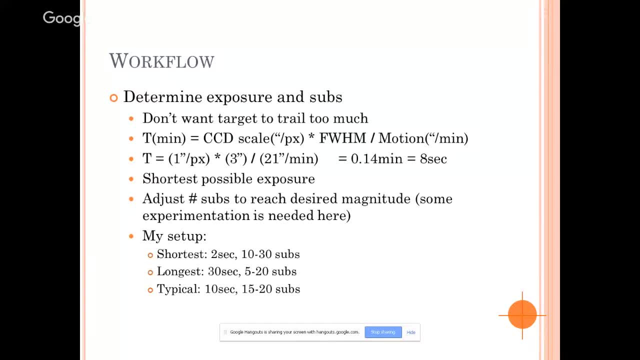 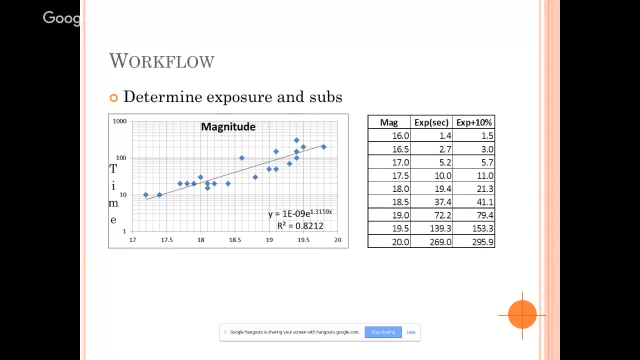 Typically I do 10 seconds, 15 to 20 subs- And then I wanted to get a little bit better handle on just how long I need to go. so I did this- and this is kind of an empirical Attack on that question of how long do I need to expose. and basically what I did is I went through some of my recent measurements. 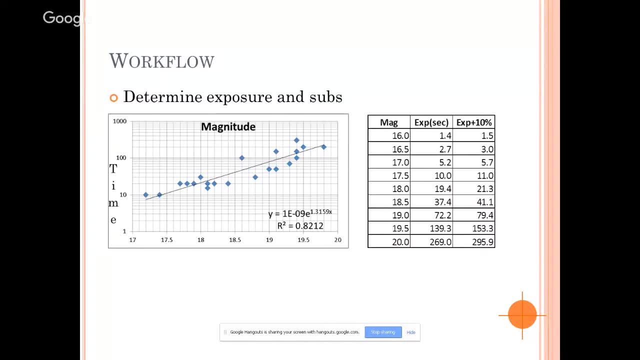 plotted the magnitude of the object Which is down here and the time it took in seconds over here- and this is logarithmic over here. And I did this in Excel And I said, well, let's try and fit a line through it And I got an okay correlation. Here's this wacky formula And I'm guessing some of this. 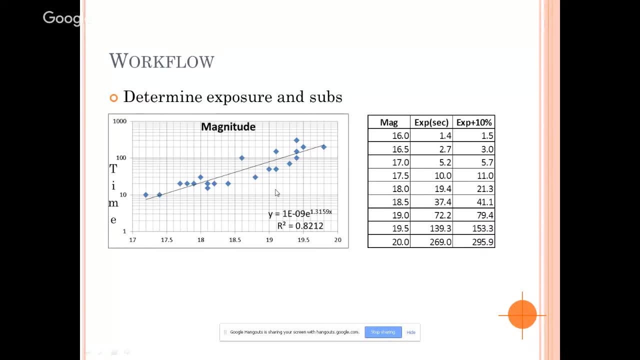 you know, these were measurements that were taken over many weeks, some lower in the sky, So you're talking about different air masses. Sometimes the moon was up. I wasn't really too concerned about that. I just wanted to see if I could do this, And I came up with this table over. 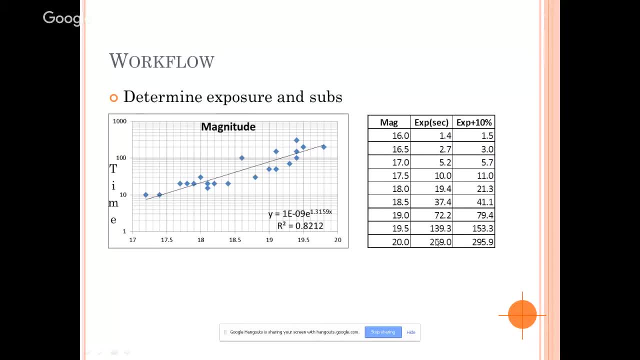 here. If here's a magnitude, here's roughly the length of time I need to go in order to get to that magnitude. And again, this just gets me in a ballpark. You know, I have to take in consideration, you know what's the condition like tonight and is the moon up and things like that. But 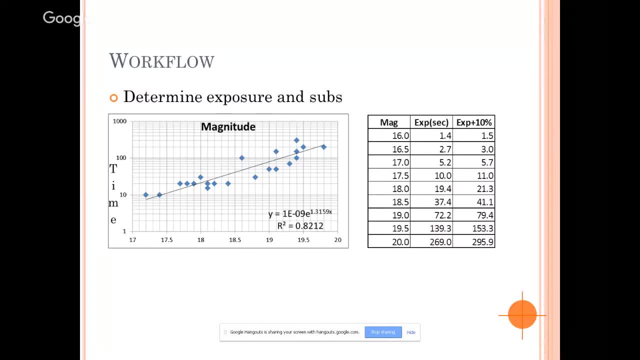 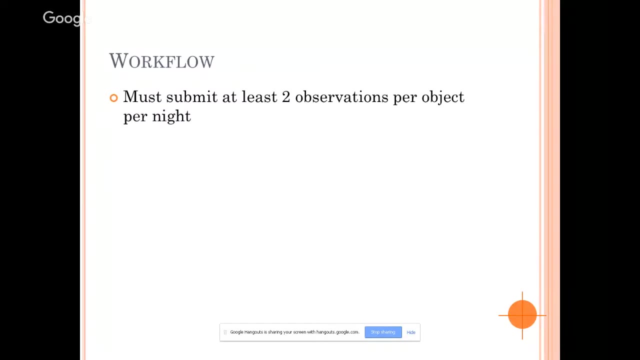 this may be helpful to do something like this for yourself. You do need to kind of have an idea of how long of an exposure do you need to get to whatever magnitude you're trying to get to. So yes, Does Cart2CL do the plate solve, sync, repoint etc. automatically? 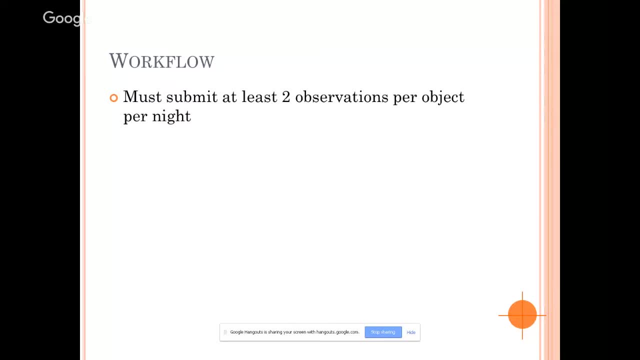 Cart2CL does not do that. Okay, It's CCDCL, the imaging package. Oh, okay, From Patrick, That's the one that does that, And it does it with astrometrynet And you need to have a local. 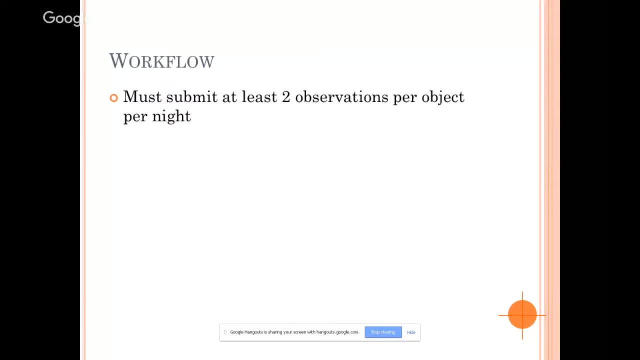 install of astrometrynet. So you need to download that. I downloaded all the index files, which took a while and took up some disk space, but I find it works the best, And you need to get astrometrynet running locally, which can be a little bit of a task but it's not too. 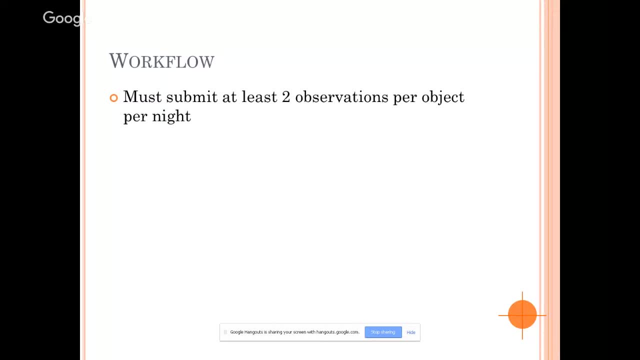 difficult if you go through all the directions and just play with it for a while. Okay, And I might have missed this, but you're not doing that after each frame. How does the program have a track on the asteroid, as opposed to just moving an RA? 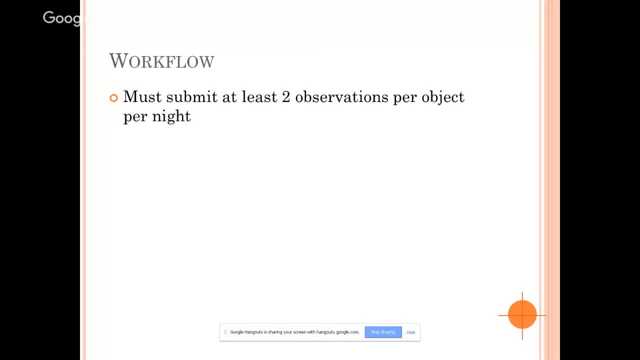 Okay, I am not tracking on the asteroid's motion. Okay, So you just let it drift through the frame. That's the whole idea behind taking the shortest exposure so that this thing doesn't trail. Okay, I don't have one of those mounts that tracks on asteroids. You can probably use that. I don't. 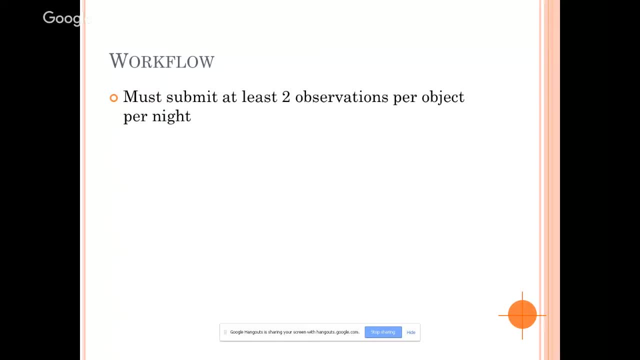 know how astrometrica would respond to tracks? Okay, Okay, It will do the trick when it does it's trailed star images, when it tries to find matches, and does it's plate solving in astrometrica, which we're going to talk about here. 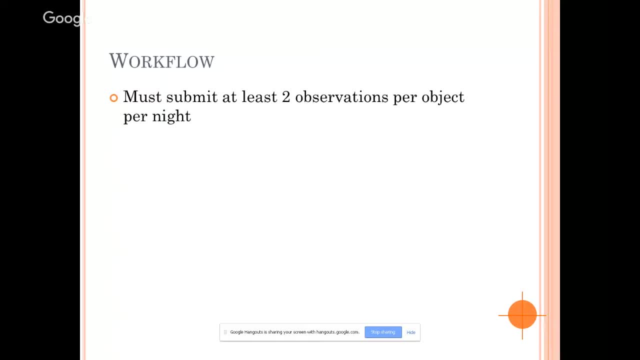 Okay, Does that help? That helps? yes, So I talked about you need to submit two observations per night. Yes, At least. So you need to kind of figure out what's the wait time between your first set and second set. you want the object to clearly move. to make sure that you have identified this. 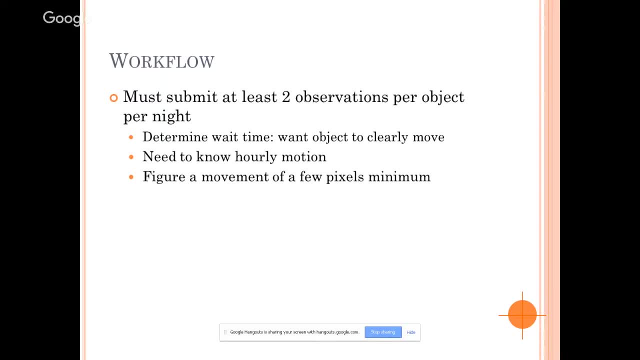 so you need to know the hourly motion, you need to figure out the movement of a few pixels. now, when i say you need to do this, you don't really need to do that. what i typically do is wait five minutes, and that's how long i wait between taking my first and second set. 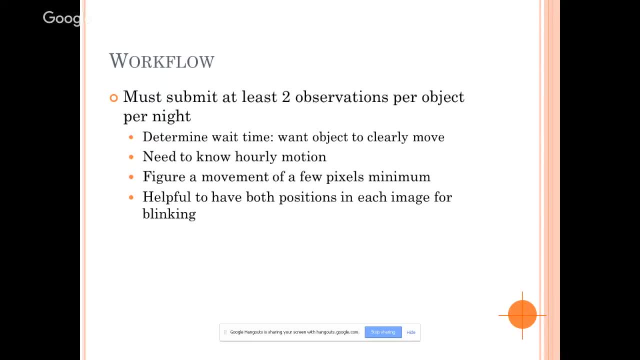 of images. sometimes i wait 10 minutes, but usually it's five to ten minutes. um, what i found helpful is that, however long the delay is between your first and second set, it's useful to have: uh, the first set and the second set have as many stars in common. 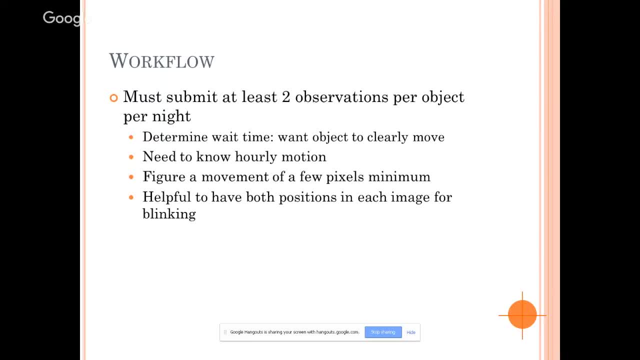 uh, in both of them. that way, when you blink them- which i'll show in just a minute, um, things that are moving between the two images will stand out easier. i hope i explained that well. um, i kind of go through that exact same process in one of the 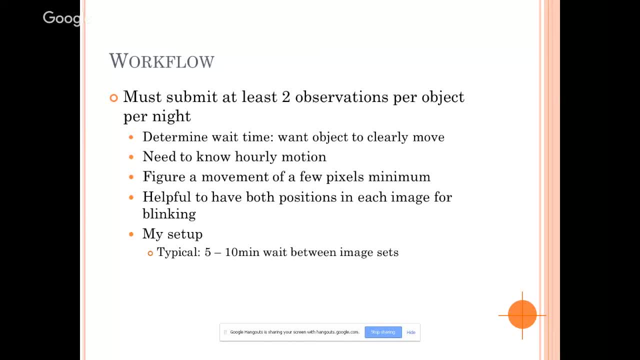 screencasts, but i just find it helpful to have both images reflect the same star field. that's not always possible, um, so typically i said five to ten minutes between the image sets. uh, that works well. um, just a couple notes while you, while i'm doing the imaging. uh, they could be pretty much unguided. 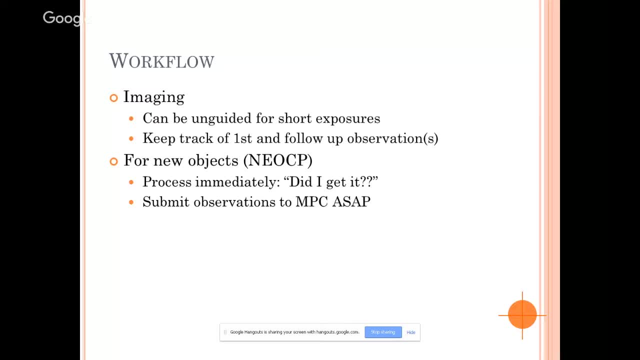 because you're you know you're talking 5, 10, 20, 30 second exposures. most i ever do are 30 seconds. um, sometimes i'll go a little longer, but rarely, and you need to keep track of this first. and what are the individual activities that you would for our sort of a有一été? fit. i'm just calling them often the percent. um, after the turn i put it up for our census. but i'm trying to replicate what this is. you sent me a link to motion. if i were to compare it in six years or seven years, i'd probably get many more. 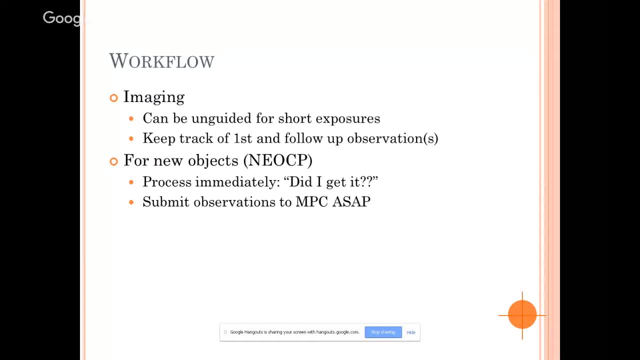 uh, someone to convert. if it's just exploreawords, bless me to submit those observations like that night, because that will help other observatories keep track of this object. so you know, astronomers over in europe, they, they get positions and then they, you know, shut down for the evening. and uh, observatories over here in the east coast, uh, 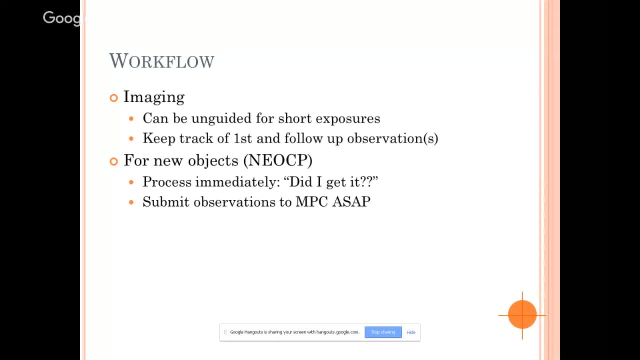 start up and then observatories in the west and observatories out in hawaii and then around the globe, really. so keeping track of these new objects is kind of a global effort, ideally. um, for post processing, you just do a standard calibration bias, dark and flat, that's it. 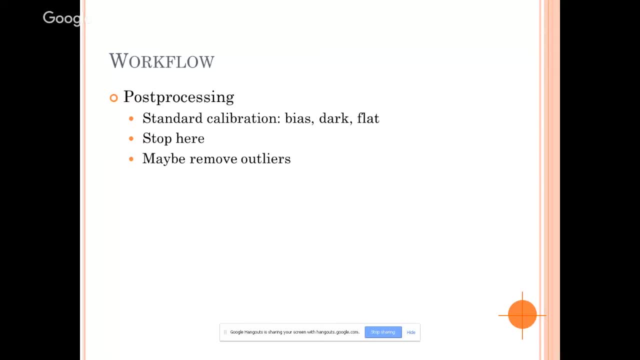 don't do anything else occasionally. i found it helpful to remove outliers. it can help see some of the faint stuff better, but really simple post processing. um, i want to talk a little bit about astrometrica, the software that you gotta have to do the measurements, uh, basically, you, you do a track and stack, uh, if you need to, unless you can. 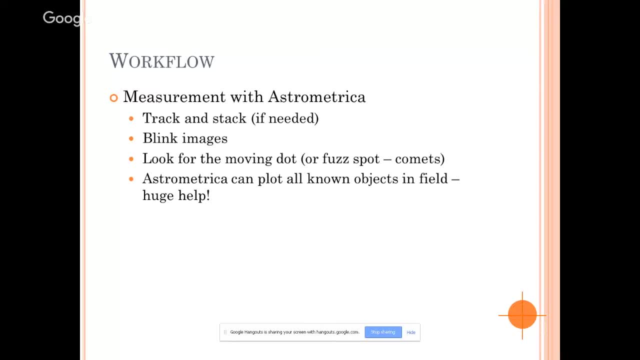 get your object in one image. usually everything i do is track and stack and then you blink the images and you look for the moving dot or the moving fuzz spot. and there's some neat things that astrometrica can do. one of them is that it will plot all the known objects in whatever particular field of view. that 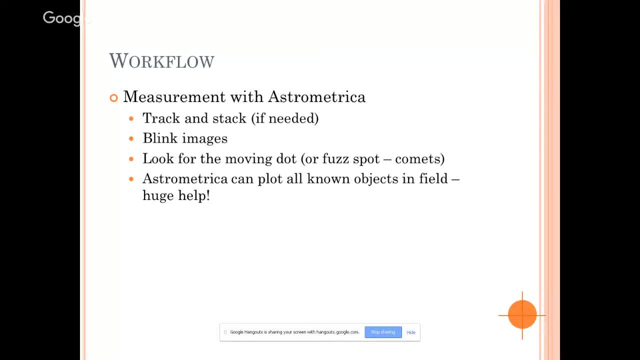 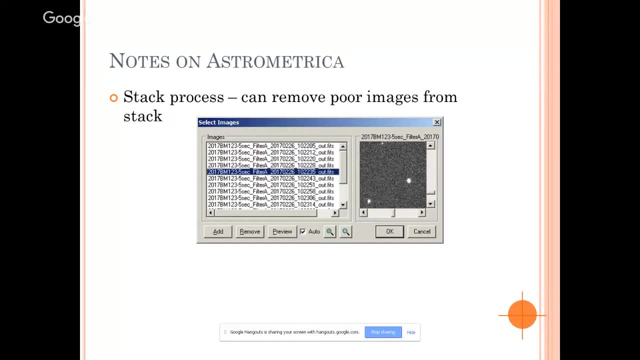 you're looking at and it will draw a little box for all the things that are there and that can be a huge help in identifying things. uh, so just a couple notes on astrometrica. uh, here is, uh, the, uh, the screen where you load in all your 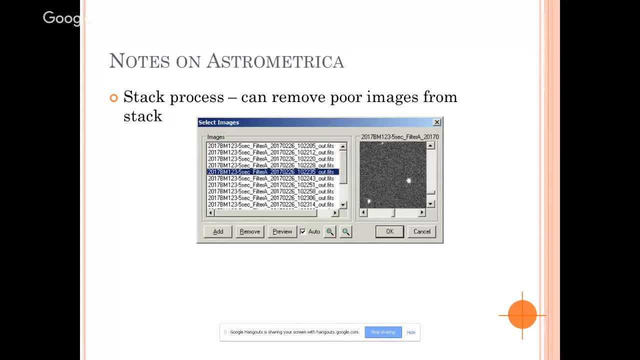 images, uh, and you can see, here is my list of images, uh, and you can go through these one at a time and you can see a small section of them over here. um, and if any of these stars don't look good- maybe a gust of wind or something move your scope. uh, you can remove them from the stack. 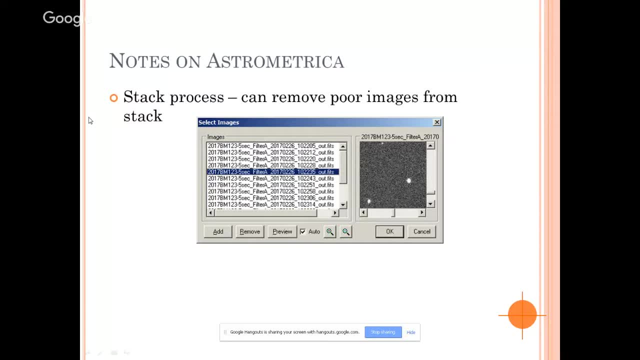 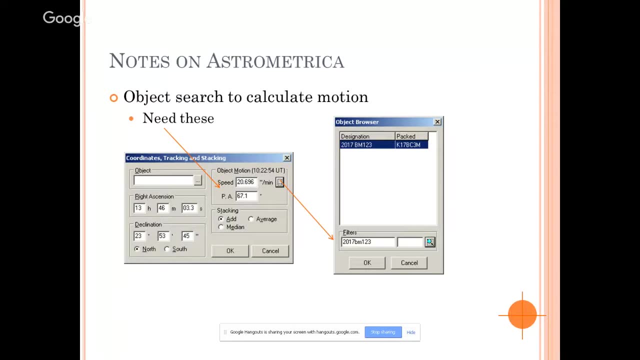 um, so that's, that's a little bit of information about astrometrica, so that's a nice, nice feature. uh, after you've loaded them in, you need to tell astrometrica how do you want to stack these things? you need to tell, you need to tell it the the motion. 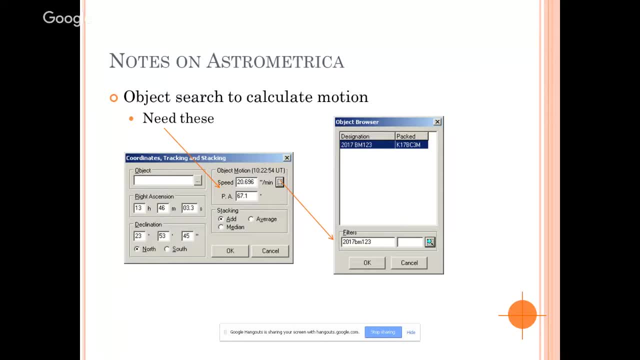 of the asteroid at that particular date and time. um, astrometrica makes that real easy. uh, what you do is you click on the little button here and you type in the target, you do a search and it goes through the entire list of hundreds of thousands of asteroids and comets and finds a. 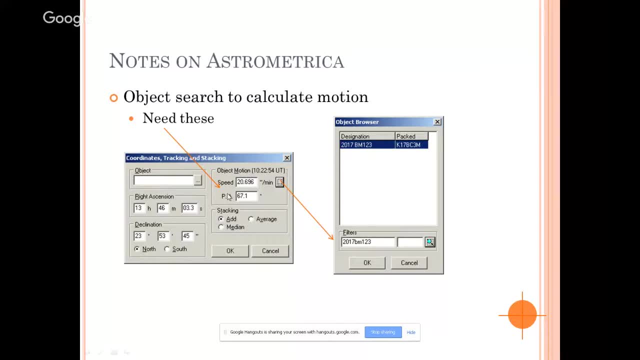 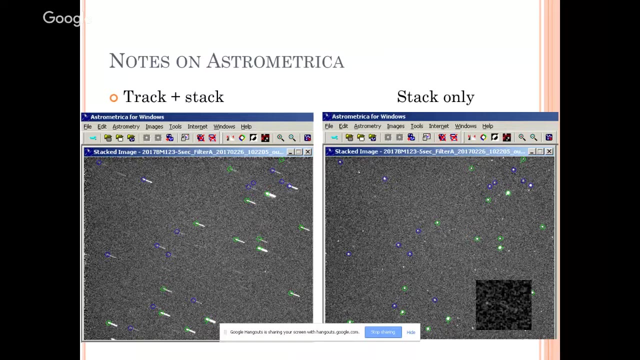 match, select this match and it automatically populates the the motion fields here. this is going to tell astro astrometrica how to stack these things. um, here's an example of a track and stack image. and just to stack, uh, you can see there's a little dot right here. that's the object in the track and stack this. 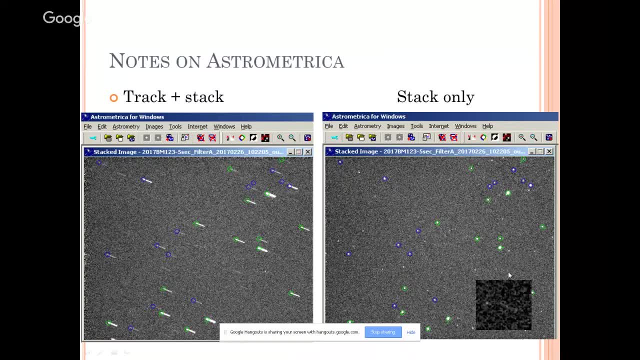 is just a stack and the object is right. here is a streak. um, probably can't see it. i don't even know if you can see the one that i tried to enhance down here. um, you know you, you obviously don't want to have, you don't want to measure a streak, you want to measure the position of a dot. 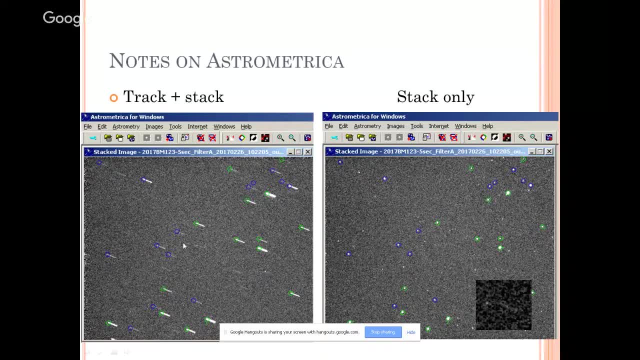 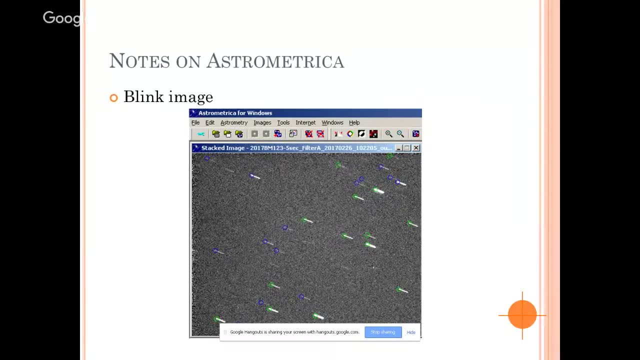 that's what i asked. that's the way astrometrica works works. The green circles reflect the reference stars that it's using, And I think I have an example of a blank And I don't know if this is going to work, So let me know if you. 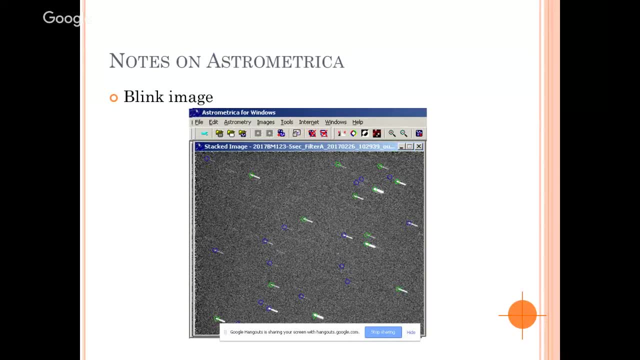 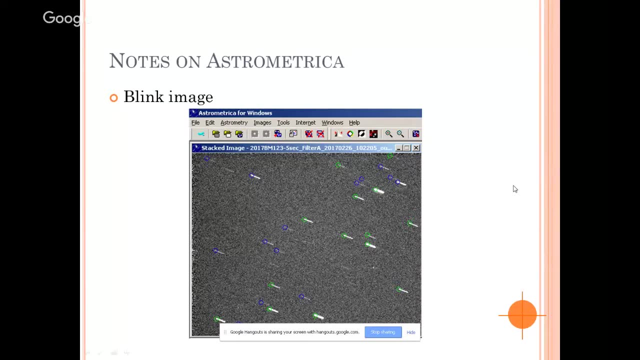 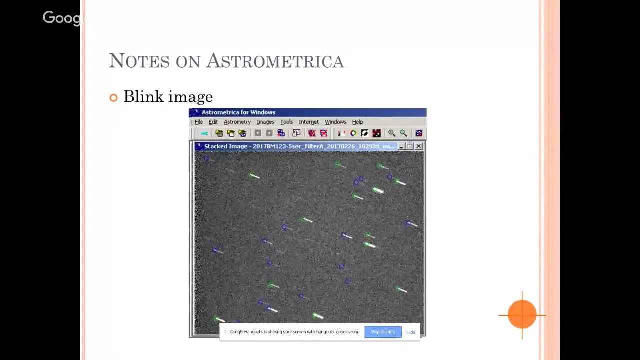 see the little dot move here. I'm just going to flash back and forth. The dot is right here and then it's somewhere up here as I go back and forth. Oops There, If you see it, great, It's a moving dot. If you don't see it, no big deal. But that's what you look. 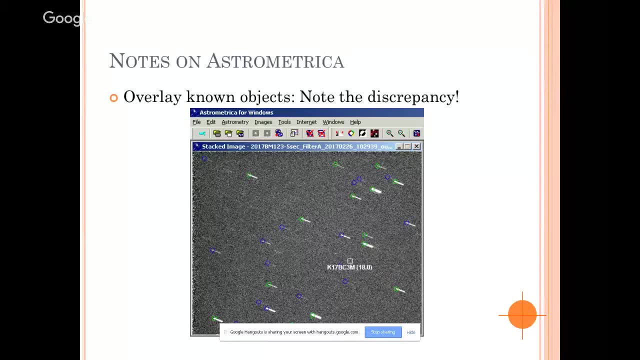 for I think we can see it. Okay, great, And I mentioned Astrometrica has the ability to plot the positions of everything that's in that field of view, whether it's an asteroid or a planet, So I've told it to do that here. Here is where the orbit says the object should be, And here 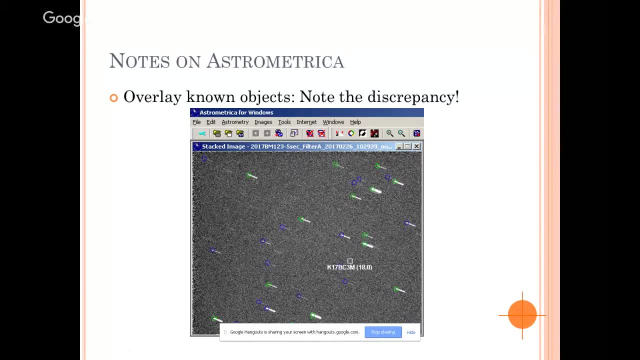 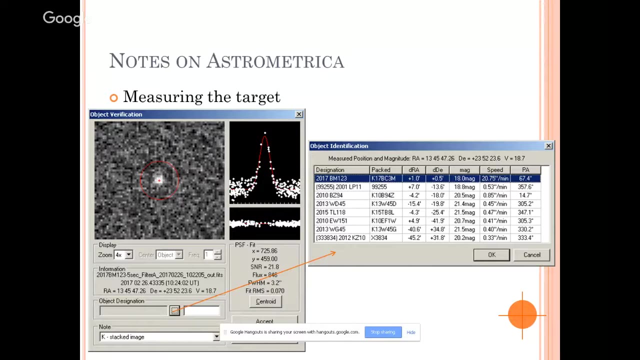 is where the object actually is at that specific moment in time. So you can see there's a discrepancy here. So this is certainly an object that needs some refinement in its orbit. A little bit on how to measure the target: You basically click on the dot And then you. 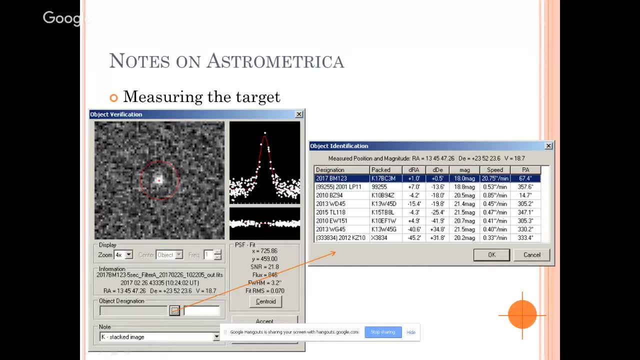 have the point distribution And it shows you how the light distribution relates to a point spread function. here Looks good. It shows you some other information here. Now you need to identify this object. So you click on that little identification button down here and it will again go through the position you specified And it will show you. 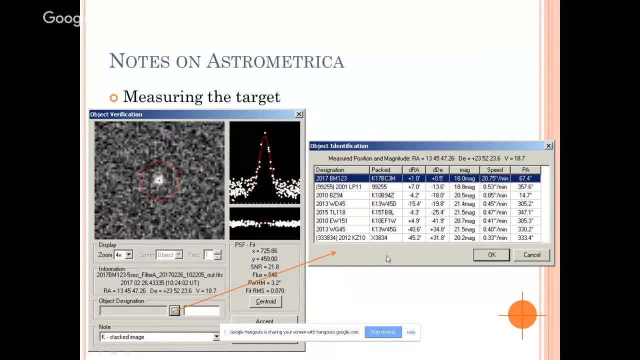 a list of all the objects that are close to that. This is a huge document, A magnet, And it's going to show you exactly where that object here is. huge help, um, it's amazing that i can go through this so fast. uh, and it shows you. you know the the? 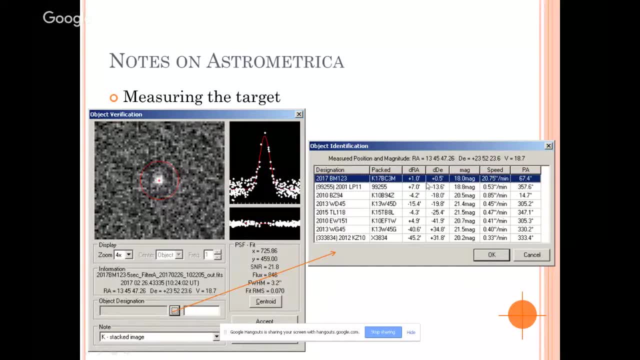 probable object that's closest. in fact, this is the one we're looking for. it shows you the the difference between its actual, the measured position minus its actual positions. these are observed minus calculated. uh, so it's a little bit off. um, so you would click ok and that would. 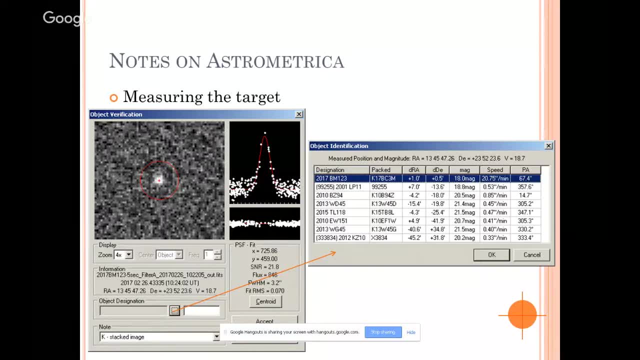 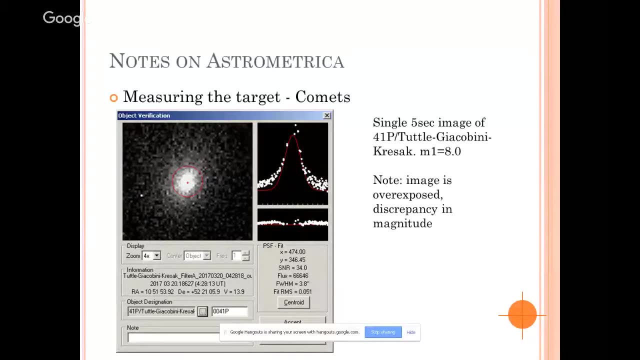 be your first measurement. do it again for the second set of images. um, i wanted to note here something about comments. i haven't been talking much about them, uh, but this works for comets. the problem with comets is you don't have a nice little point source to uh to deal with. you got 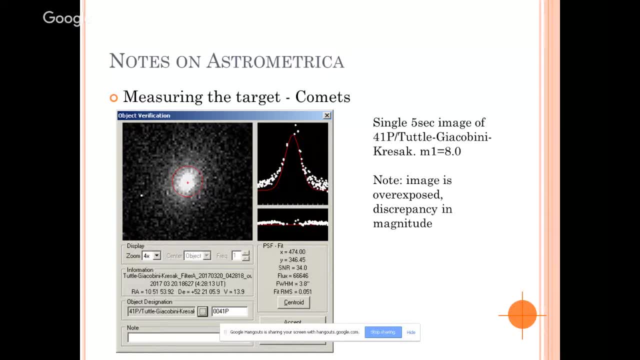 a fuzz ball and astrometrica will will try to find the center of that. uh, that's that fuzz, but it's not going to be the center of that. uh, that's that fuzz, but it's going to be the center of that. uh, that's that fuzz, but it's going to be the center of that. uh, that's that fuzz. 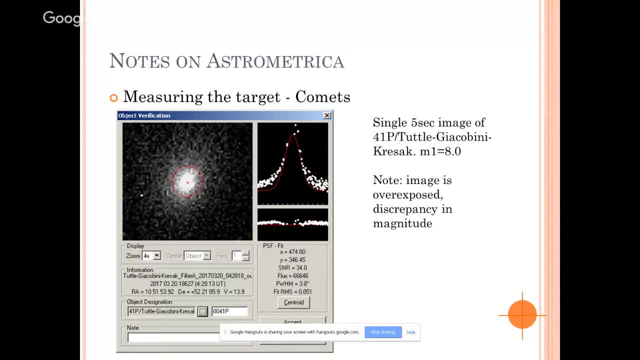 spot, but it you know, it's not. it's not as accurate, uh, and basically what i'm showing here. this is a single five second uh image of uh comet 41p and it's overexposed. um, i probably should have tried for maybe a one second or even a half a second exposure here. 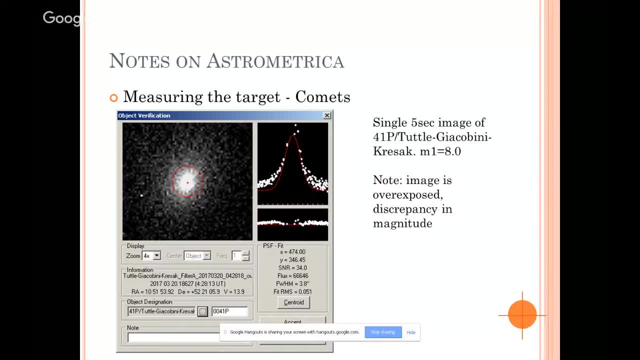 it's just overexposed. it probably still can give me a good measurement and i'll probably submit it, but it's it is overexposed. uh, another thing i should point out is this magnitude. this program is saying that this thing is at magnitude 13.9. however, in reality it's probably closer to 8.0. 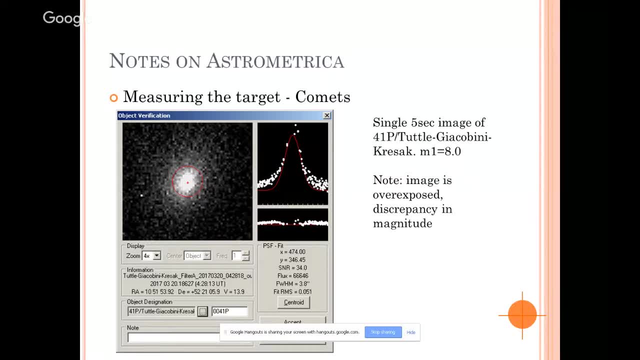 the way astrometrica calculates magnitudes, uh, for asteroids works pretty well. the way it does it for comets, uh, is a little different. uh, the method in the math is the same, it's just the results you get. uh, because it's a diffuse object, um are a little wacko. uh, they're, they're much fainter than they. 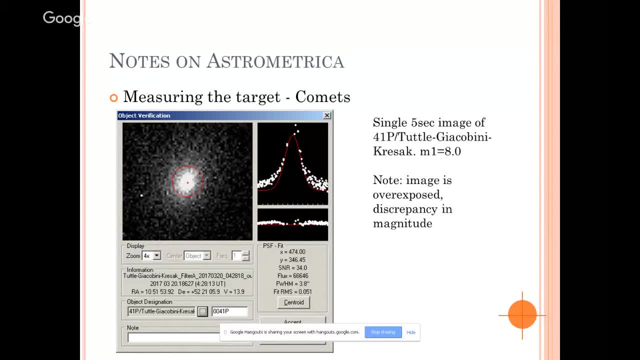 are in reality, um, and it has to do with the way the magnitude is calculated and the fact that the background it's assuming here really isn't the background it's, it's the extended part of the coma, so that grossly skews these, these magnitudes um. 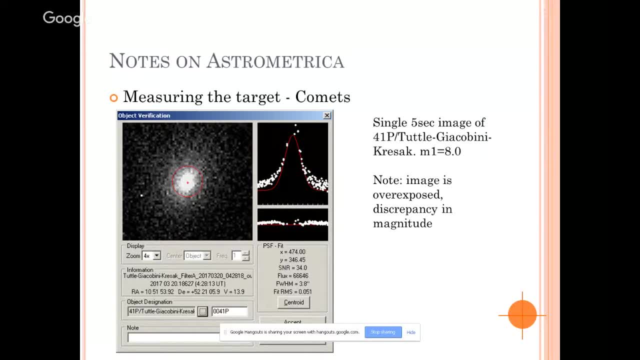 which you know, the minor planet center is aware of and they're not too concerned about comet magnitudes, uh, other sites that collect those uh measurements strictly for magnitude purposes. visual estimates, um, maybe you don't want to use the ones astrometric gives you because those 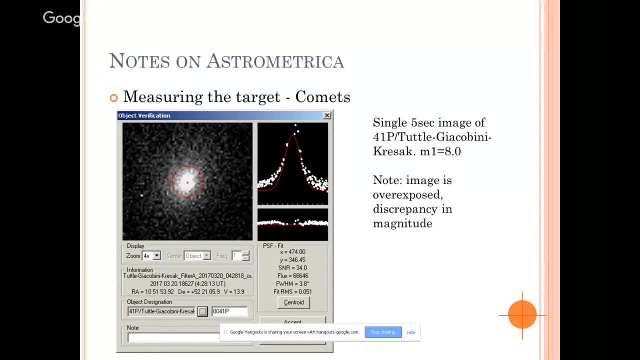 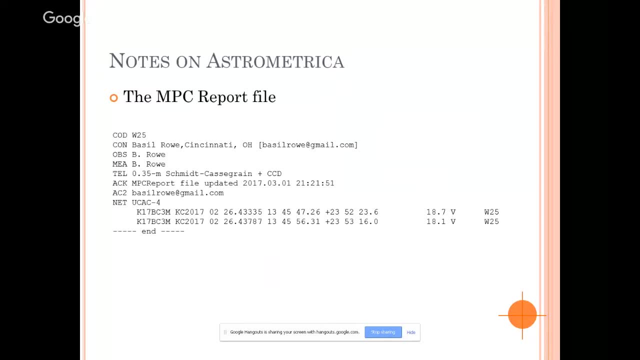 don't really reflect the visual magnitude. uh, so here's the report file. it's generated, um, and this has to be a very specific format, um, and things have to be in certain columns and they have to be laid out in a certain way. you know, basically you can see. here's the name, the date, 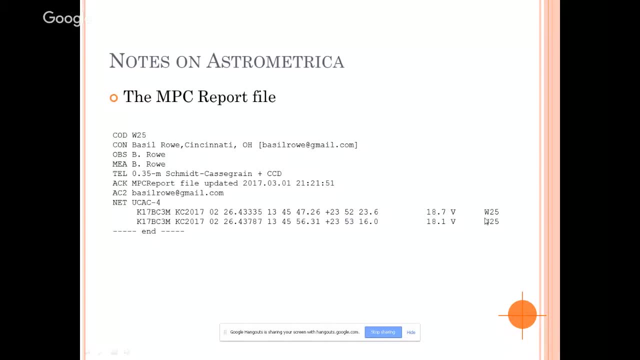 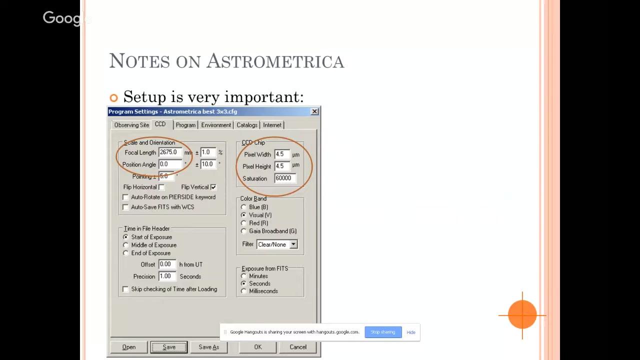 the time. uh, right, ascension, declination, magnitude, and and my observatory code. so this is what you would send off to the minor planet center. um, astrometrica does that automatically. i'll show you that in just a second. just a couple other notes about astrometrica, the setup of the program. uh, if you decide to, you know, go with this and. 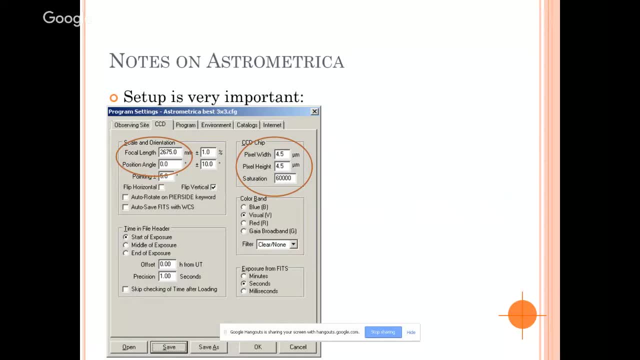 explore it further. you need to get astrometrica set up properly and there's good documentation and help file on how to do this. but things like the focal length, uh, and the position angle of your camera, um, those are important, obviously. the pixel size and your saturation limit, those are very. 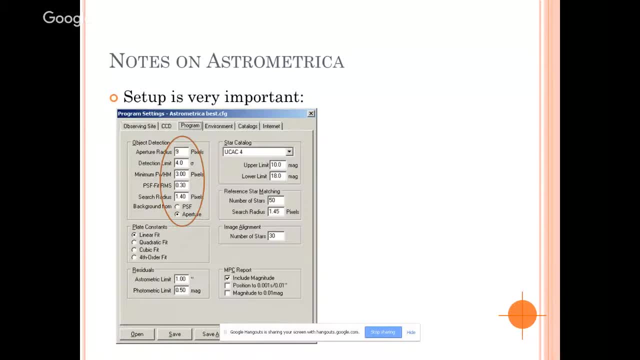 important. um, a couple of other things in this, in this program tab, uh, things like everything in here. you have to spend a little bit of time reading the the documentation to figure out what you need to put in there. um, you just can't accept the default values that it comes with. 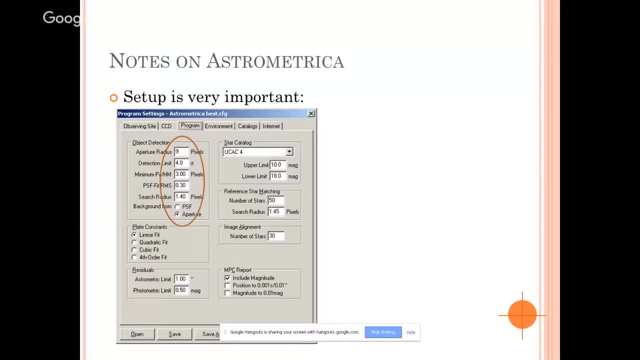 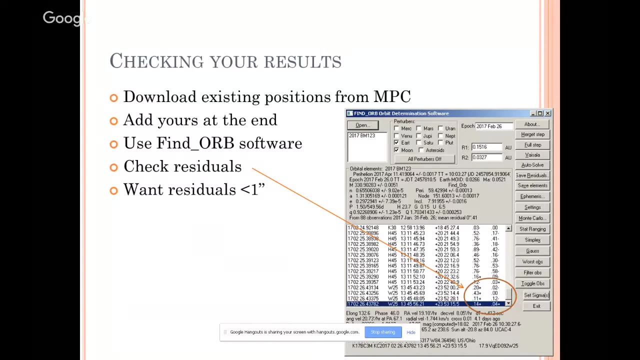 so there's a little bit of work involved in setting up astrometrica, but once you get it set up, as long as you don't change anything on your system, your setup, your scope, then you're good to go. um, so you've made your measurements, uh, you're ready to submit them to the minor planet. 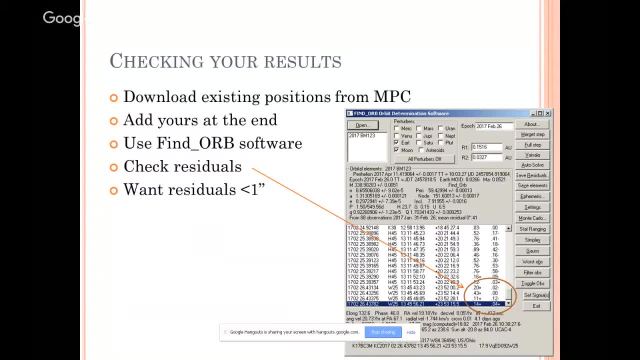 center. but you're wondering, you know, how good are these, uh, and do i really want to send them off? i certainly was that way, uh, when i was getting started, i basically wanted to check everything before i sent it off, which is probably not a bad idea, uh. so there's a program called find orb where 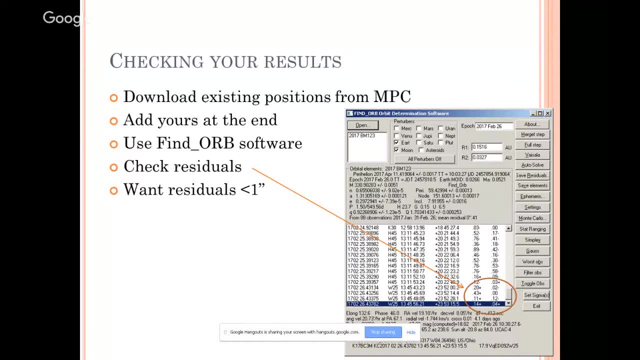 you can uh tag your measurements on the end of other observatories measurements and i have a specific screencast that shows you how i do that. but basically it's a text file that you grab from the minor planet center that has all of the existing positional measurements. 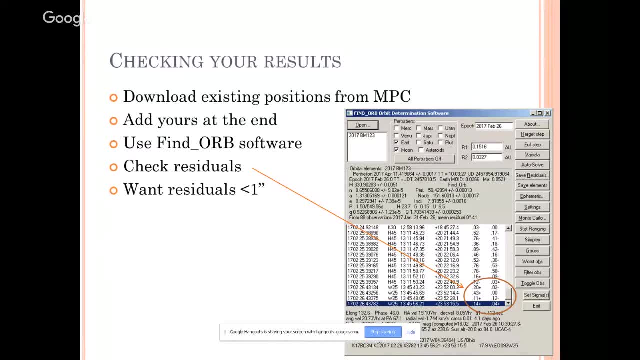 you open that up in notepad and you stick your measurements from the report here. just copy and paste those two measurements to the end here and find org will process all the measurements. and what you want to check are these last two columns, which are the residuals, uh, the observed minus the calculated, and which are shooting for. 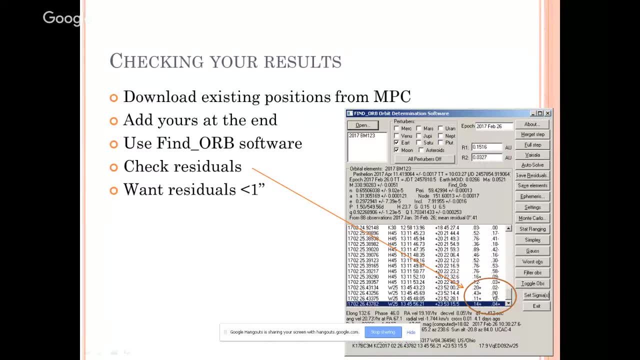 something less than one arc second, and in this case you can see i happen to do acceptable. so these are good measurements that i would send off. i know i was checking everything before i sent them in, uh, because i just i didn't you know really not what i was doing and i just wanted to be sure that i was submitting useful data. 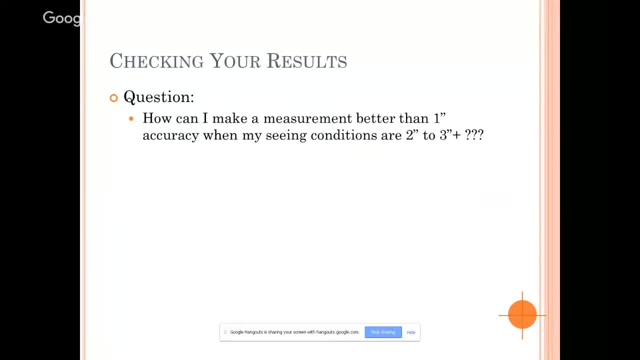 um, so you may be asking a question: how can i make a measurement better than one arc second accuracy when my seeing conditions are two to three arc seconds? that's a very good question and my simple answer is: it's the math- uh, the centroid calculations, and the math used in plate. 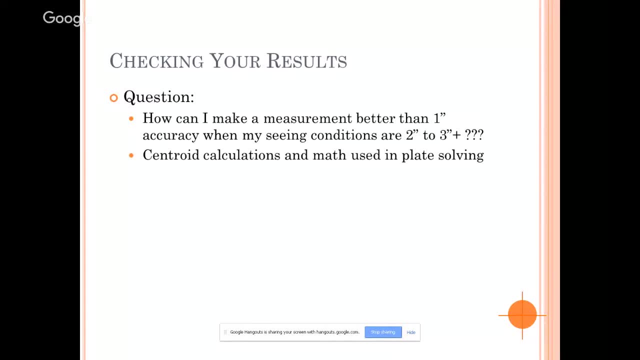 modeling that that runs on, that runs behind the scene in astrometrica, uh, just makes that happen. and that's the extent of the answer that i'm going to give to that question. but it's a good question and and basically, astrometrica and the math make it work. 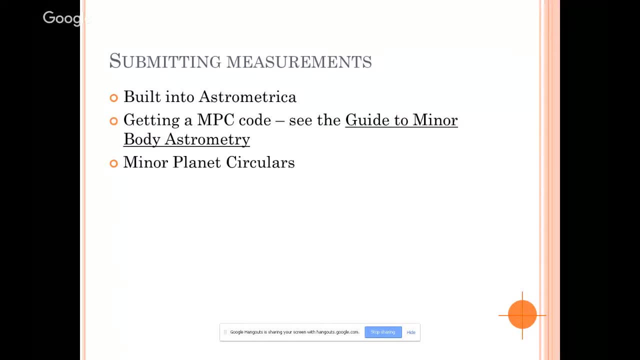 um, so finally here submitting measurements, uh, that that file, the astrometrica, creates. uh, there's a feature built into it. um, basically, you set up a smtp email server that you can use and you just send those out. that way, you can copy and paste those measurements into an email and send them off. just make sure you use. 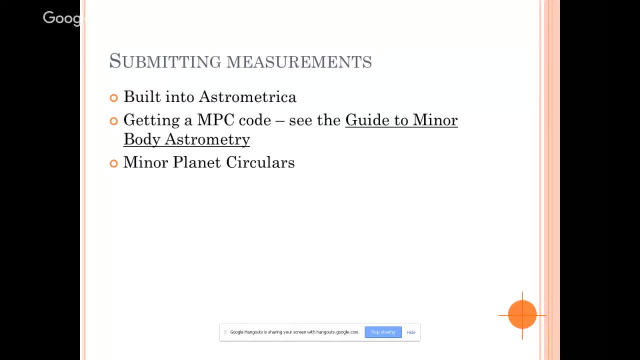 plain text, they don't want html. um, getting a minor planet center code, an npc code? uh, i just refer you to the guide to the minor models under body astrometry they. they lay it all out in there as to how you can get a code for your observatory. uh and finally, your measurements. uh will appear. 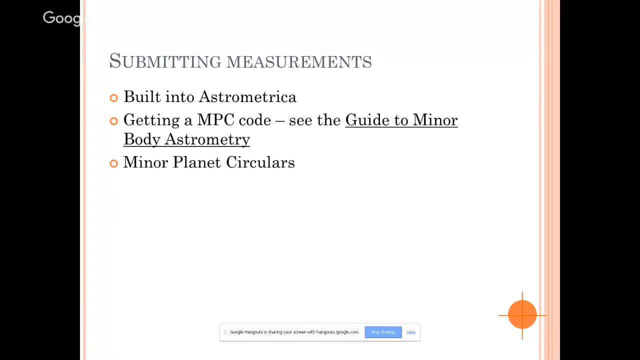 in publication in uh, the minor planet circulars. uh, those come out around every full moon. uh, they are quite voluminous. uh, thousands and thousands and thousands of measurements uh get published every month by the, by the minor planet center. um, it is quite a herculean task that they go through. 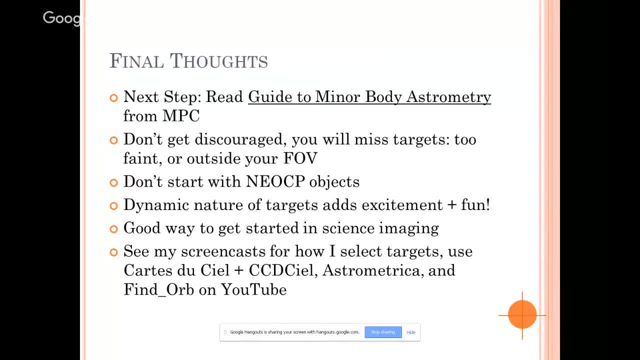 um. so my final thoughts: uh, if you want to go further with this, i i suggest the next step: just read that guide to minor body astrometry. i know i've said that several times. um, don't just don't get discouraged. uh, you will miss targets. um, i've missed many uh, either too. 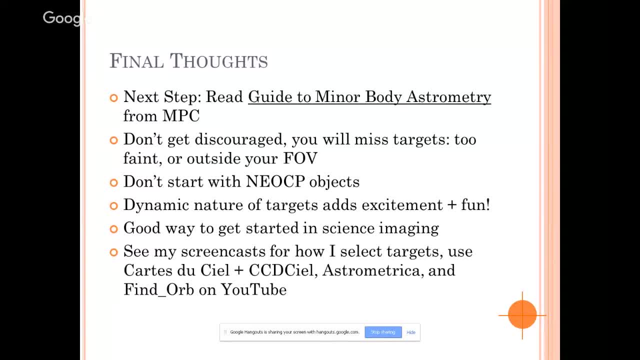 faint or outside my field of view. the position was off. uh, it just is the nature of of the beast. i suggest not starting with the? uh, the new objects, the neocp objects, um, those objects, uh, while they are probably the most valuable to get measurements on, uh, i suggest don't. 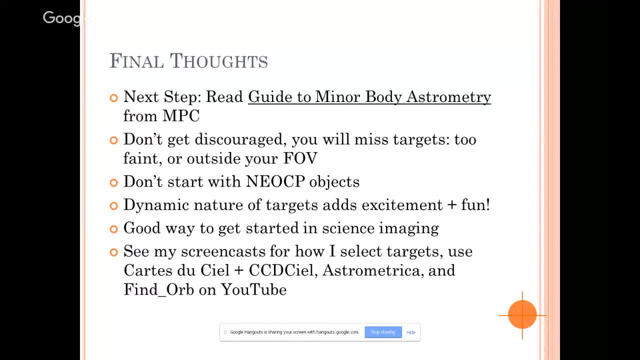 start with those, start with something a little easier that has a known orbit. uh, that's, that's bright enough, uh, just, i think it would be less frustrating getting started with those, uh, and i certainly i didn't when i was getting started. uh, the dynamic nature of this, i think just. 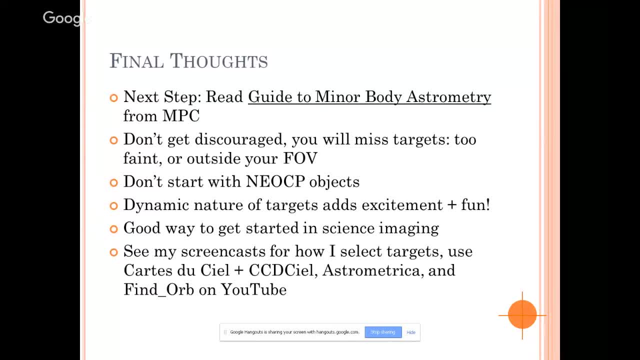 adds a lot of excitement and fun. uh, you really. you know, once i get started at night, i'm going until the clouds come in or until i can't take it anymore. it's a very dynamic, very dynamic thing. it's a good way to get started and i'll see you next time. 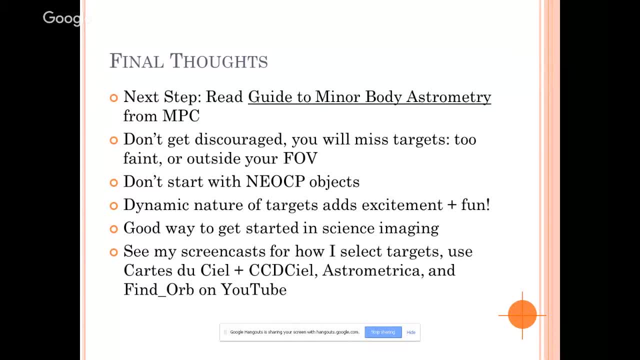 some science imaging. there's- there's definitely some possibilities for school projects. um, if you're a teacher, uh, there's a lot of stuff to chew on here if you wanna. you wanna get into that? uh. and finally, uh, if you do wanna go further, i really suggest you take a look at my screencasts. 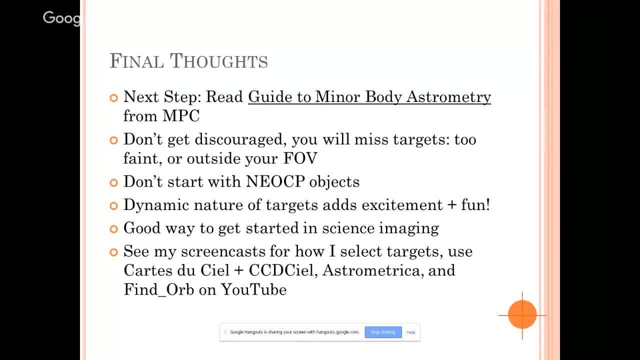 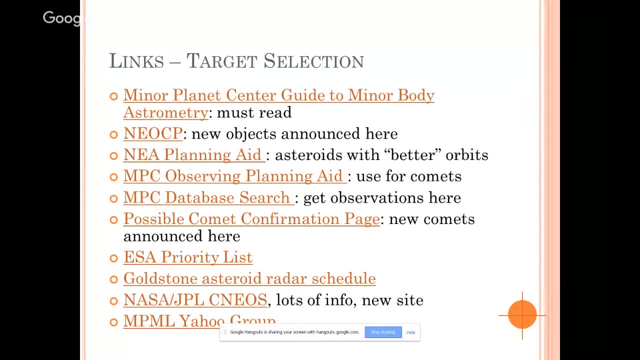 um, they're, they're not polished, they're not slick, they just are kind of. here's how i do it and i hope it will be of use, uh, some of it for you. uh, and there's links to that. in fact, these last couple of pages i'm not gonna really spend time on there's just i've got a whole bunch of links here. 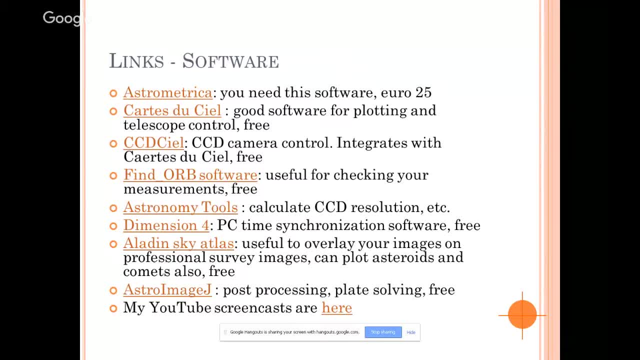 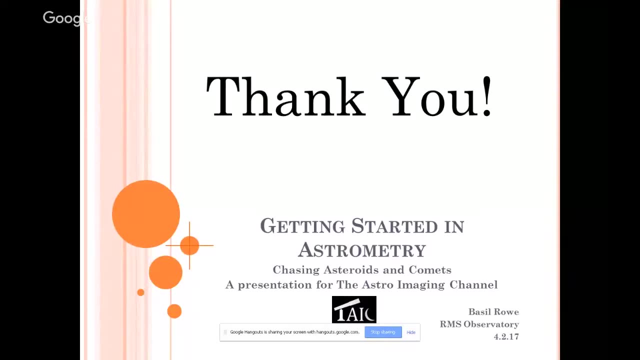 for target selection and for software that i've talked about. they're all in here and this whole presentation, i understand adam is going to make it available, if you care to download it and take a look at it later. yep, it's already posted on youtube, so, uh, if you visit, if you visit this video on youtube. 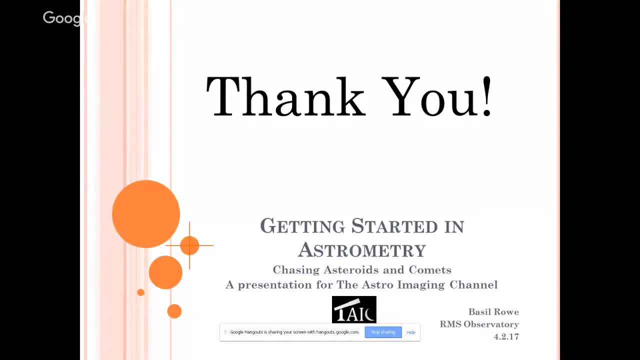 it'll be in the description. awesome, thank you, adam. that's it. thank you, i made another hour. yes, uh, a few questions popped up. i was kind of um, uh, trying to sort through them, uh, but um, questions and comments, i should say, uh, dennis wilde said he had managed to. 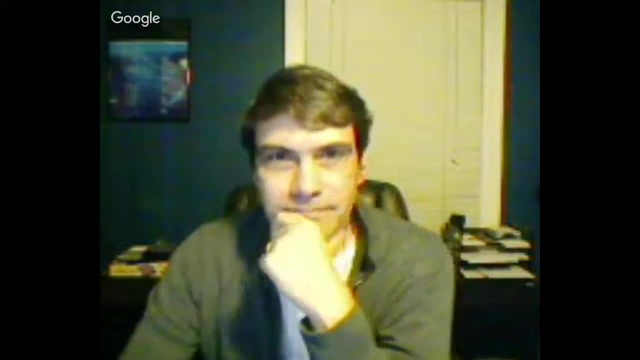 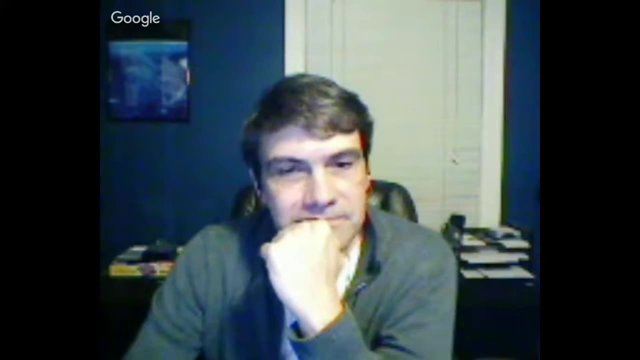 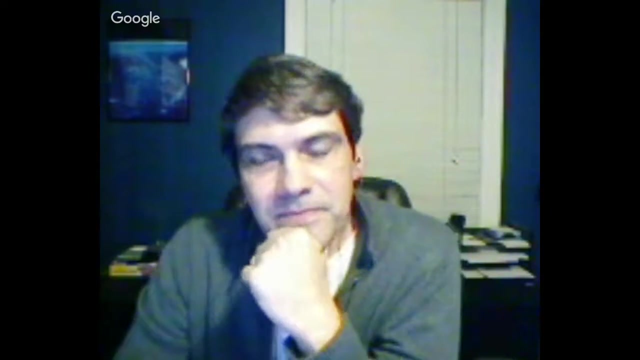 track on the asteroid with the mx plus because of his small aperture scope, but the residuals from the astro astrometrica measurements were large. so, um, you're doing it probably a better way than i was thinking by not tracking on the actual asteroid. okay, that's good to know. 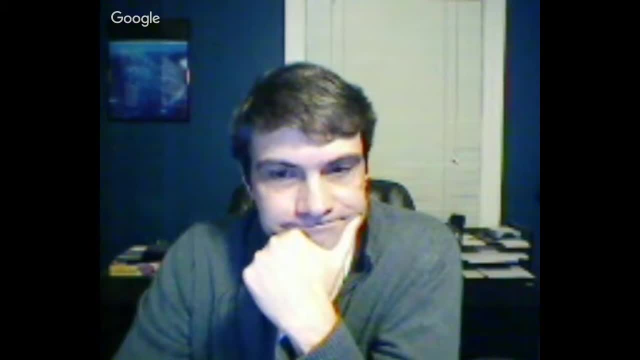 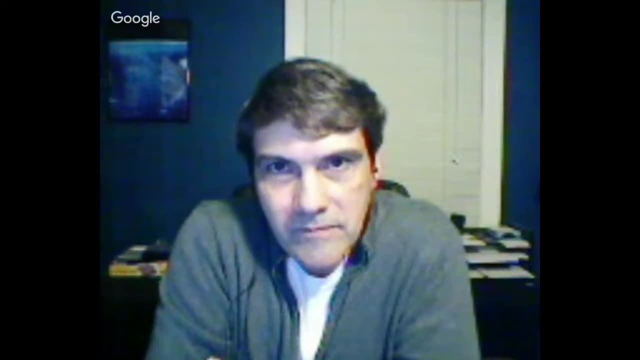 and and alex then went on to kind of reiterate um that, uh, yeah you're, you're fixing the stars in the, not the asteroid, so you get better measurements of the stars, uh, and still get that relative movement. i should say. um. dennis wilde commented he thought mpc. 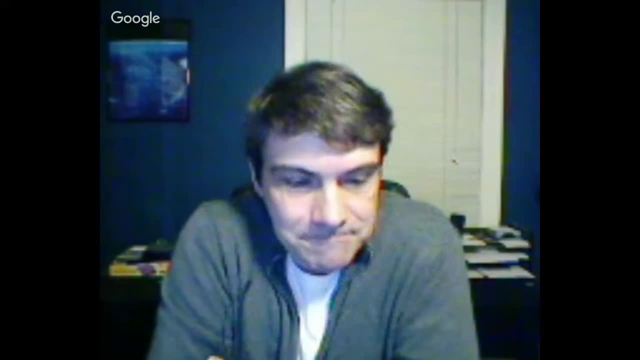 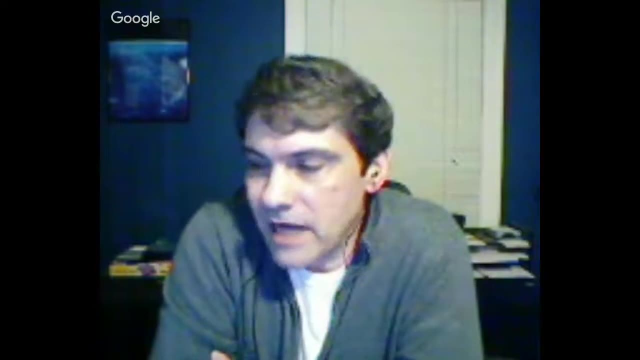 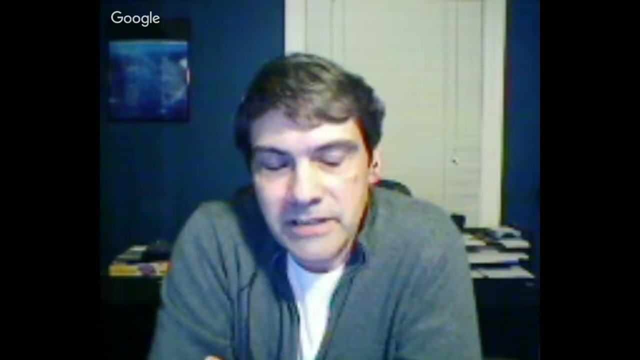 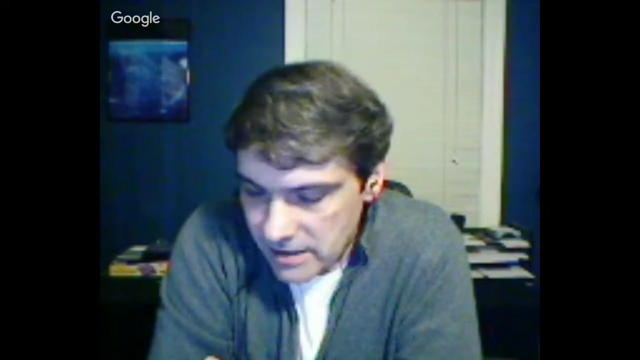 wanted 20 to 30 minutes between exposures. uh, can you speak to that? yes, uh, i do remember reading that in some of the older documentation, uh, some of the books about, uh. you know what the minor planet center prefers, um, however, if you go and look at one of their websites, uh, that uh shows the current. 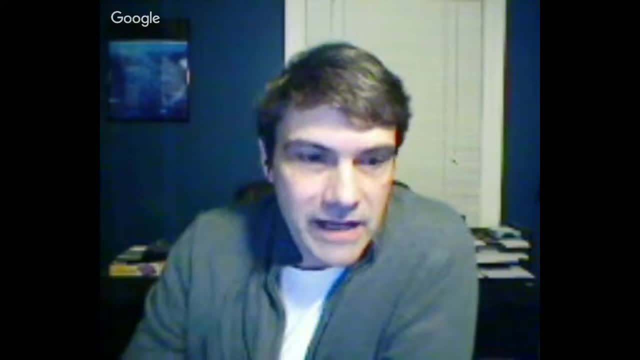 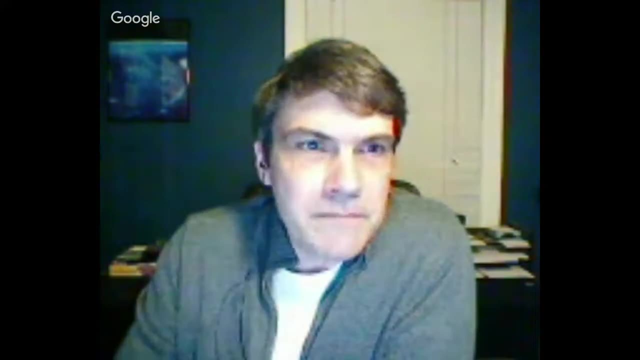 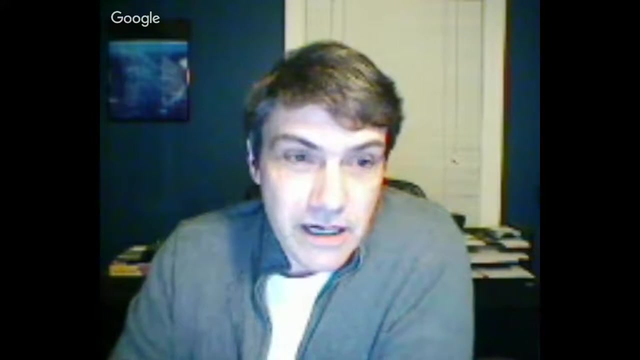 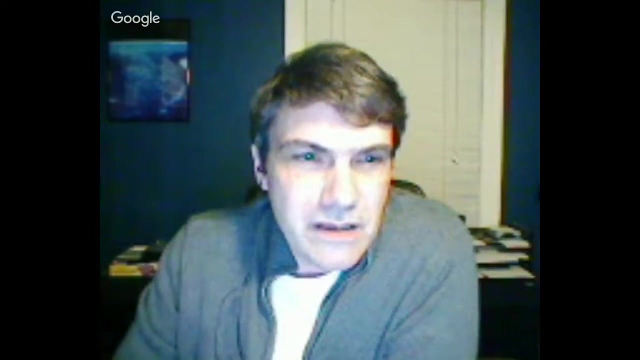 activity, um, tonight in fact maybe i can bring that up- uh, you look at what other people are doing, and some people- i mean i'm talking professional observatories- uh, they're waiting five minutes between observations, um, and that seems to be the norm today and i think in the documentation, um, that that document that i talk about, um. 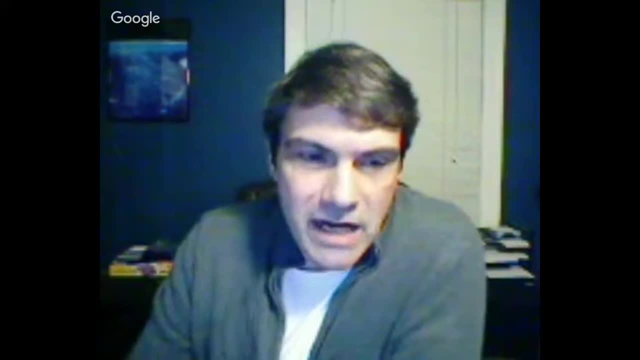 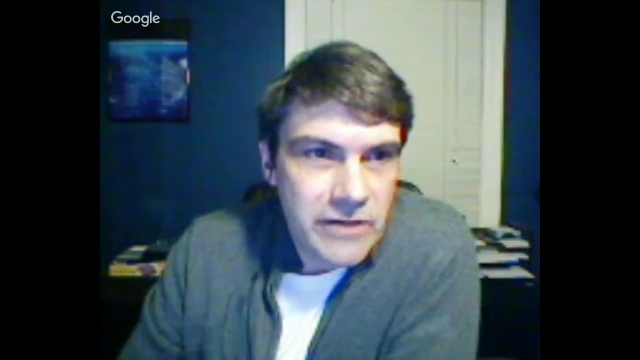 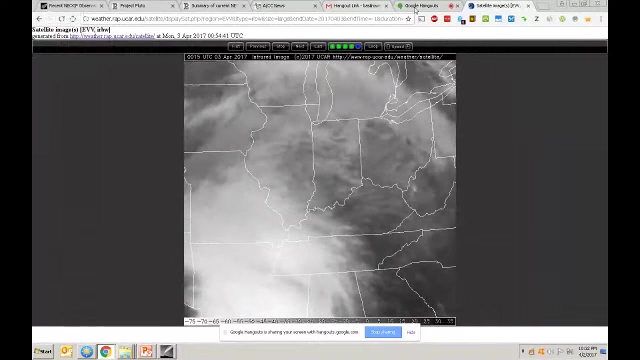 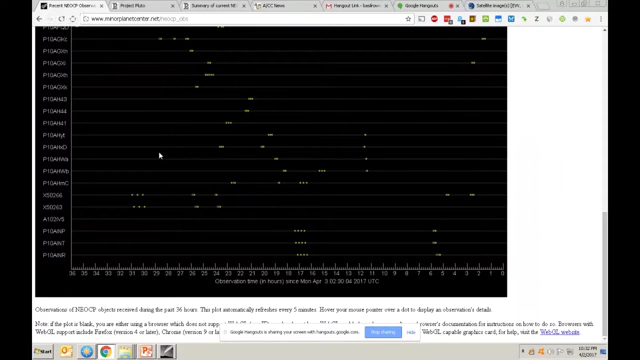 they, they don't. i think they specify a shorter wait time is acceptable. um, let's see if i can share my screen here again. yeah, oops, not the satellite, did i just zap my? oh, it's back here. uh, here's uh a listing of what's. 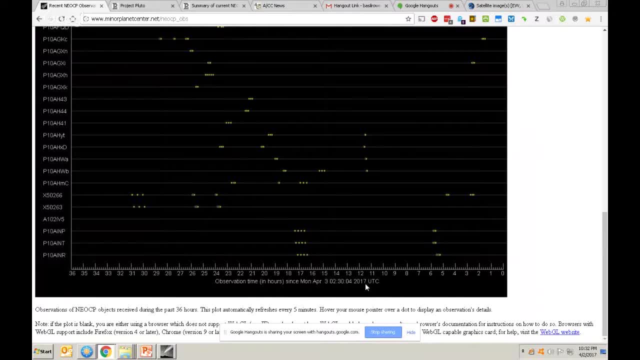 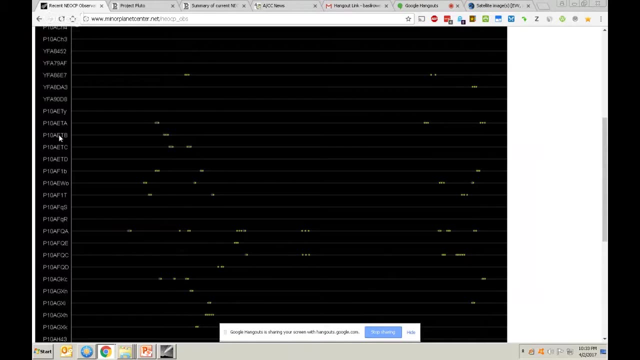 going on right now, uh, along the bottom here, here's, here's uh the tonight, right now, and then an hour ago, two hours ago, and here are all these new objects. is all the new object page. all the new objects are on here and you can see what. 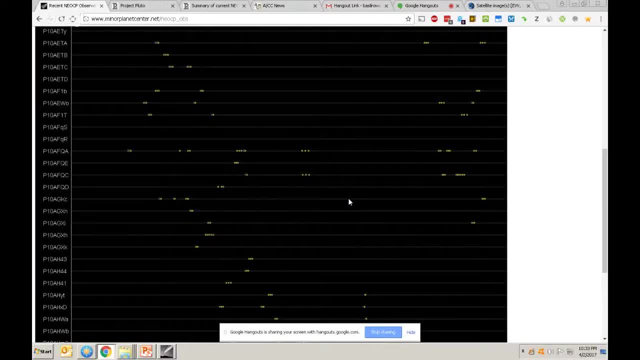 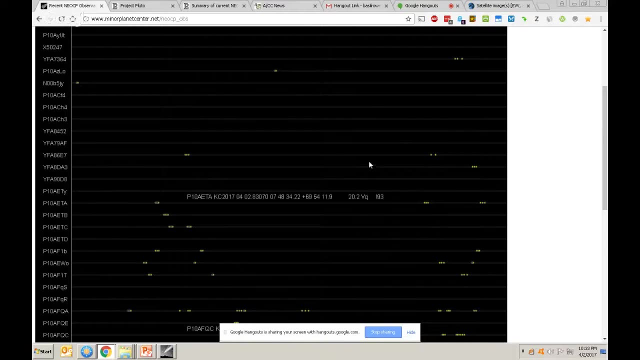 everybody's doing um, and if you look at these measurements you know this is probably about five minutes in between these two. uh, some of these are just a few minutes in between each. so, uh, i kind of assumed that you know, because everybody else is doing it, it's okay. 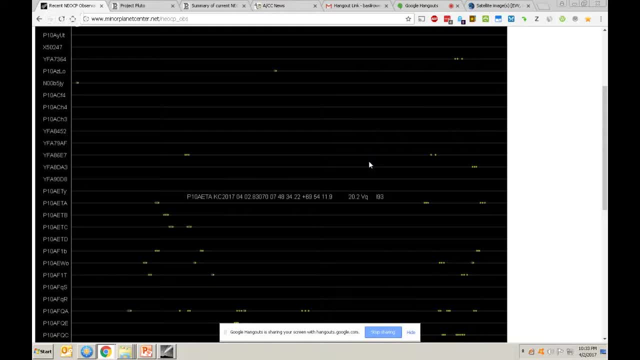 um, i do remember reading that they preferred, you know, 15 or 20 minutes, i think. uh, they relaxed that substantially. uh, i have tried submitting observations that were too close together and i got a bounce back from their automated system saying, nope, these are too close together and we're not going to take them. so there is some type of check in their automated. 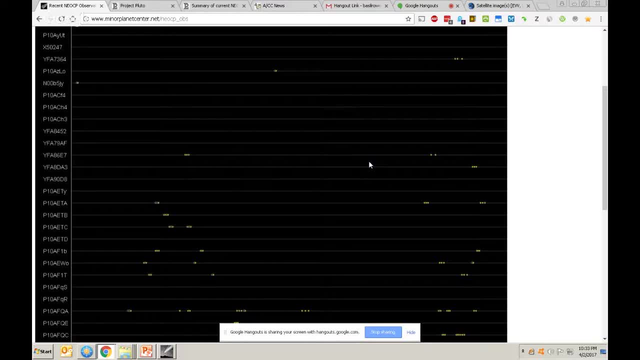 system. but i think they relaxed these because of the overwhelming number of things they have to deal with these, these new objects, objects that you know, in order for for them to just get the measurements, they had to relax those constraints quite substantially to, you know four or five. 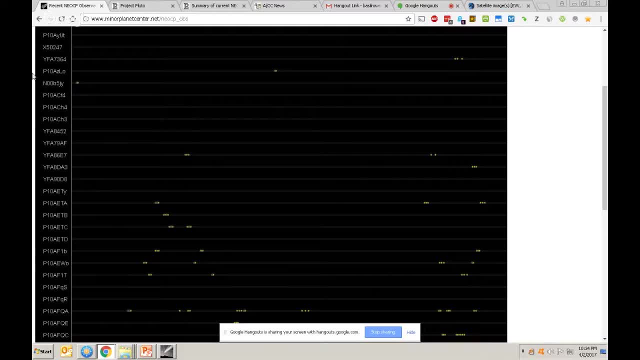 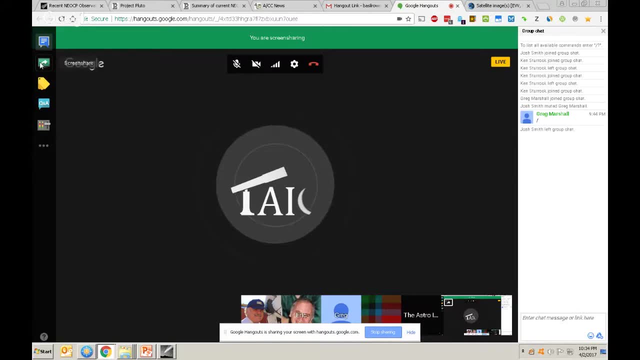 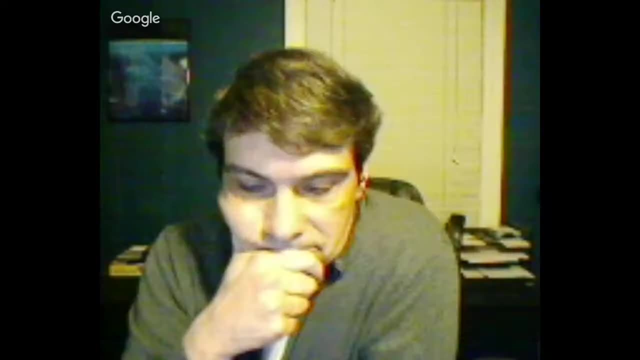 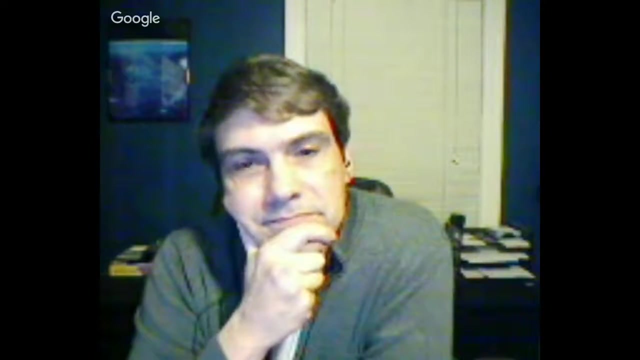 minutes to my guess gotcha Dennis wild, also commenting: setup is critical. I think you're speaking about that also in that particular program, which is which the name of its. escaping me and I think I'm the same note. he said he couldn't get the email to work, which I think you're automatically emailing. 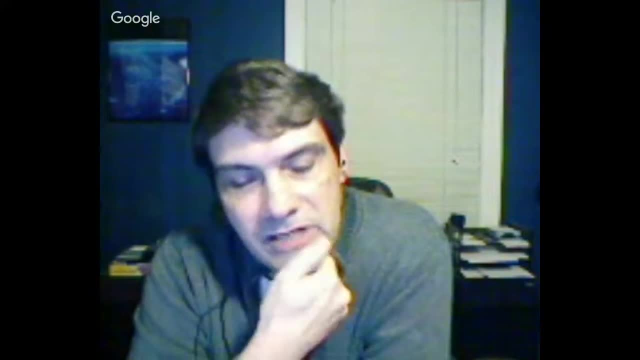 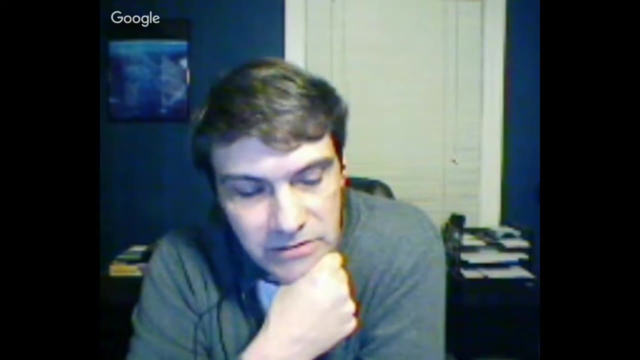 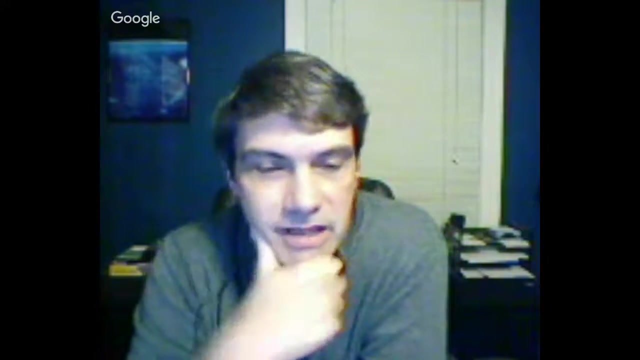 the data out. yes, oh yeah, there is a. there is a place where astrometrica can automatically send those observations out, and you do have to set up an SMTP server and tell it. when I tried using Google, which is my email it- it couldn't connect to the. Google SMTP server to send email, so I just switched it to my ISPs email server and that worked fine. I think it's a security thing to prevent spam. a lot of email servers like Gmail and Yahoo don't accept emails without extraordinary authentication. you know, I think it's a security thing to prevent spam. a lot of email servers like Gmail and Yahoo don't accept emails without extraordinary authentication. 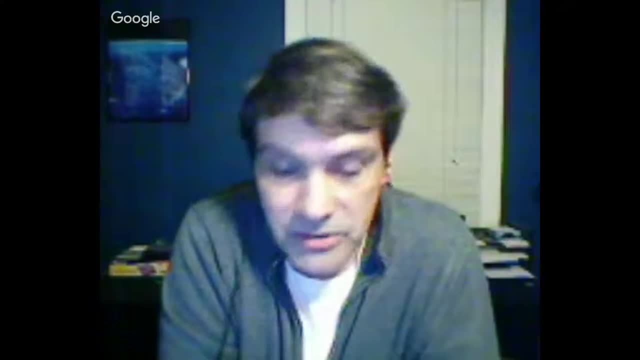 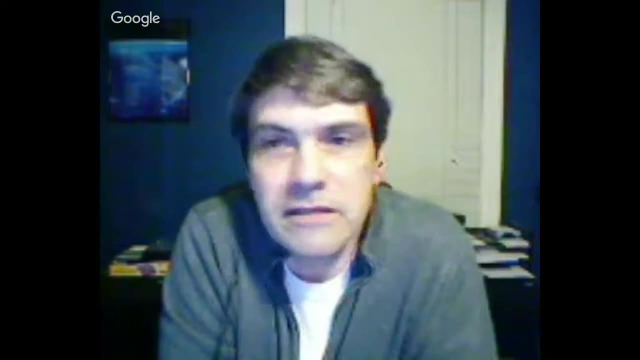 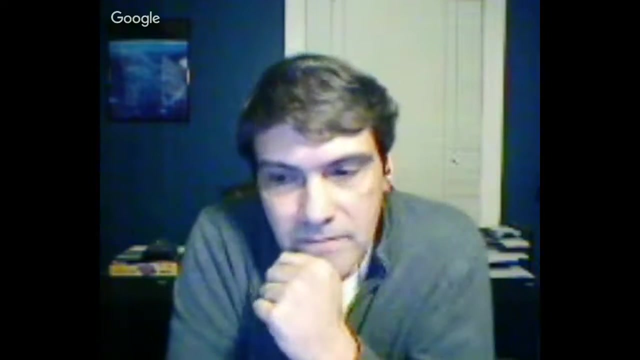 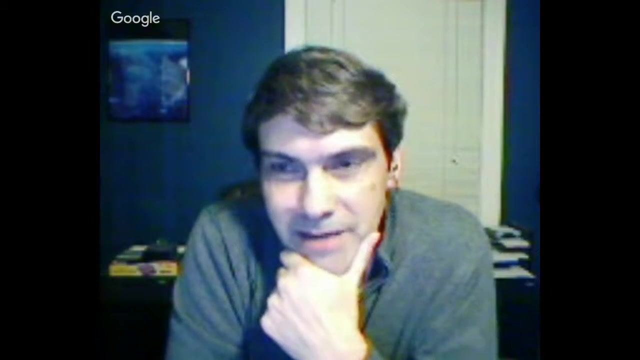 which astrometrica doesn't do. worst-case scenario: you can just copy and paste that data into a regular email- just make sure it's plain text- and send it off great. does the MPC give any feedback on your measurements? um, they will tell you if they're too close together. you get an automatic email you. 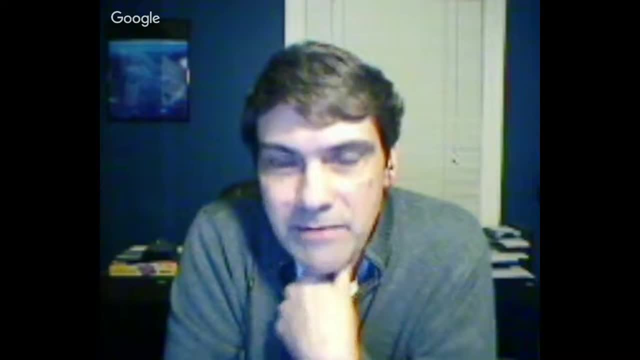 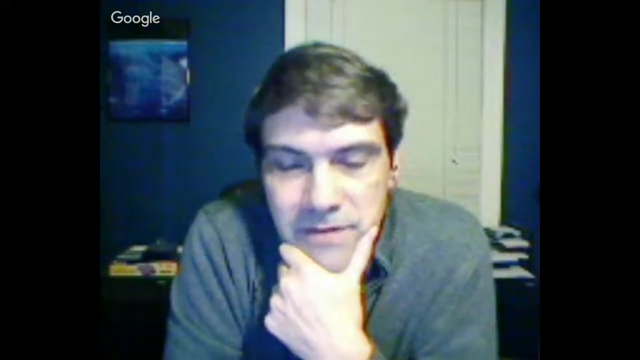 get an automatic email every time you submit something and usually it's just an acknowledgement saying we got your measurements. here's how many we we read and what you sent. you know 20, 20 measurements or whatever, and we're gonna process them if it's one of those new. 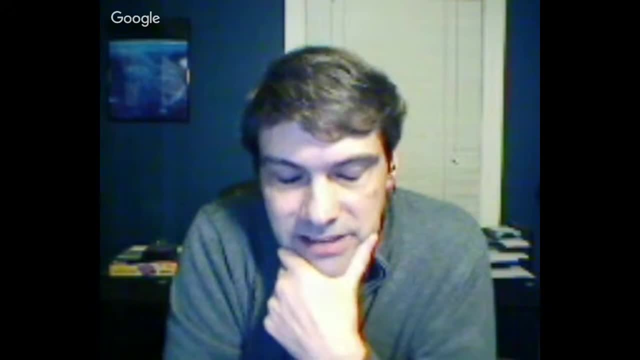 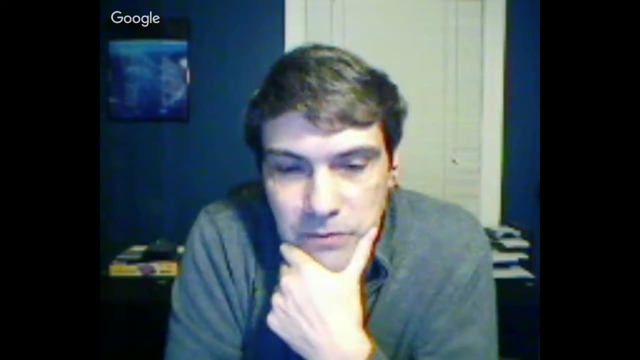 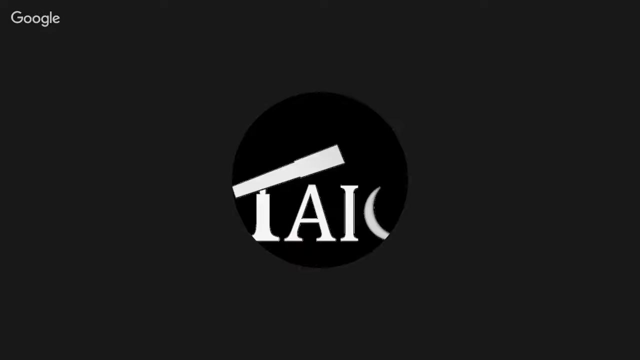 objects it. will you get another separate email that says possible any OCP candidate identified and we'll stick it in the list as one of tonight's measurements. As for any personal thank yous for doing this, no, You do get your stuff published in the Minor Planet Circulars. 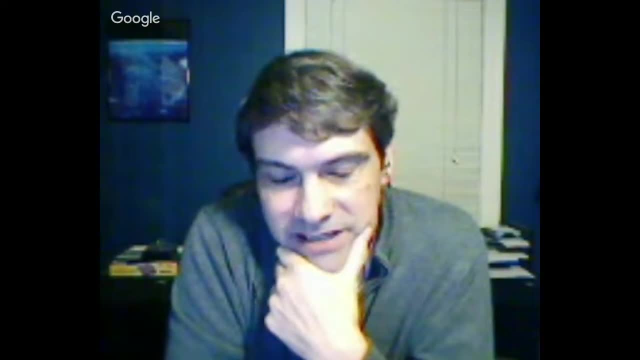 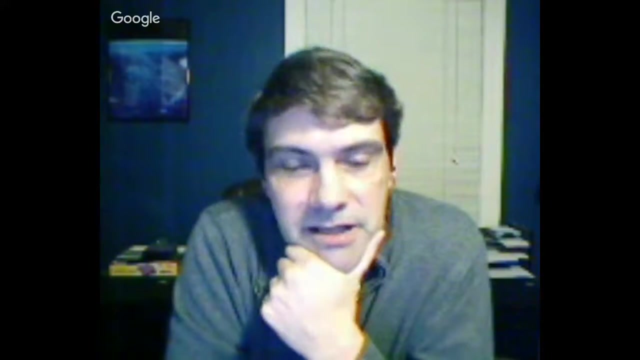 If you get in on one of these new objects and you submit measurements for one of those NEOCP objects, if that object gets enough measurements to receive what's called a preliminary designation, then that gets published, kind of as it happens. So one day you know an object will disappear off the NEOCP page. 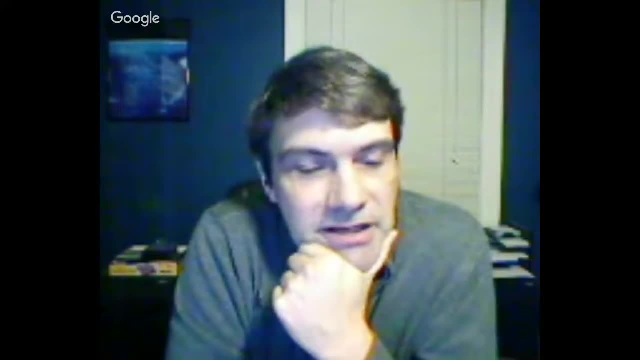 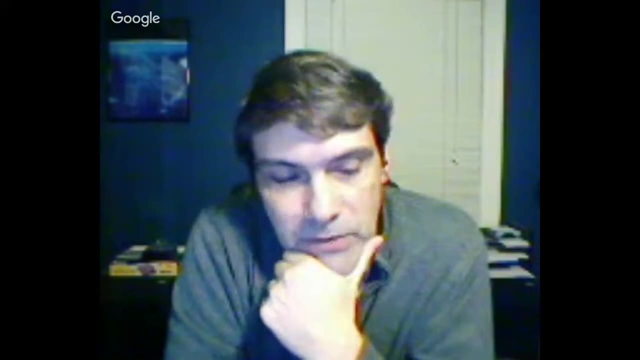 and it will receive an official designation and you'll get your name listed in that And you also get to see the residuals. That's kind of what I check is. every month I go in and look for myself, I look at my stuff that I submitted and check the residuals. 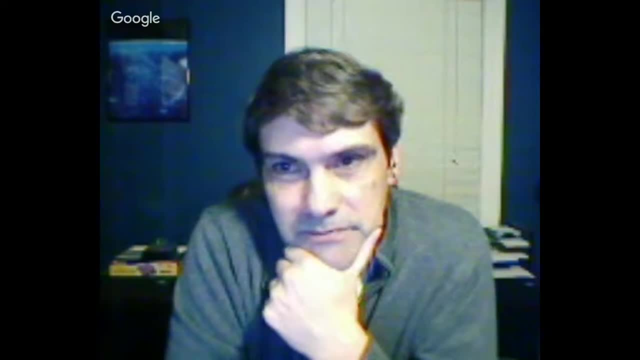 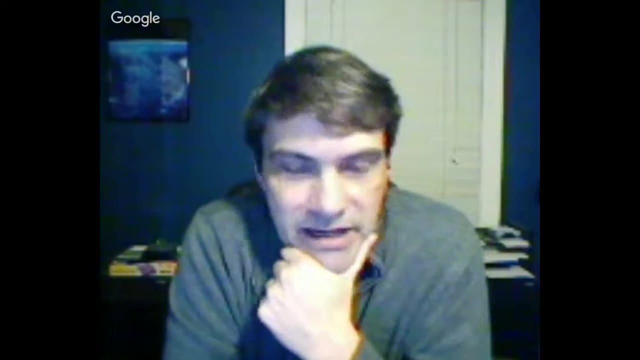 that they're coming up with, just to make sure that I'm, you know, doing a reasonably good job And if there's something that isn't good, it'll be notified. You'll kind of get a little call out in the listing there. 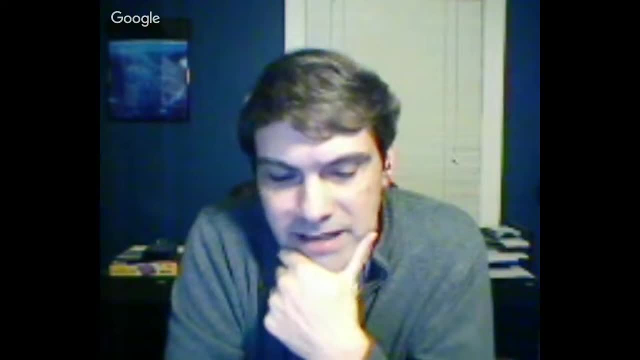 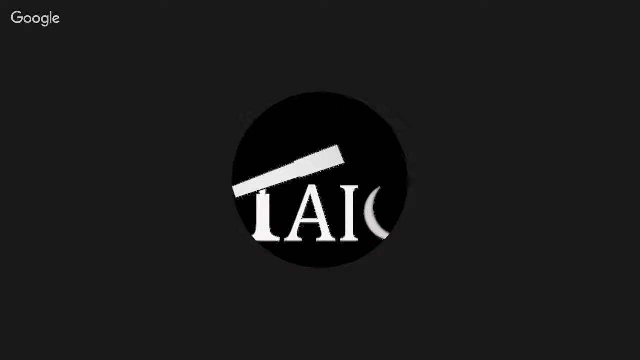 of your stuff and I go back and check and see: well, why didn't this one? you know, why did I do such a bad job on this one? Another good question from Dennis Wilde: Have you found any new objects? No, no. 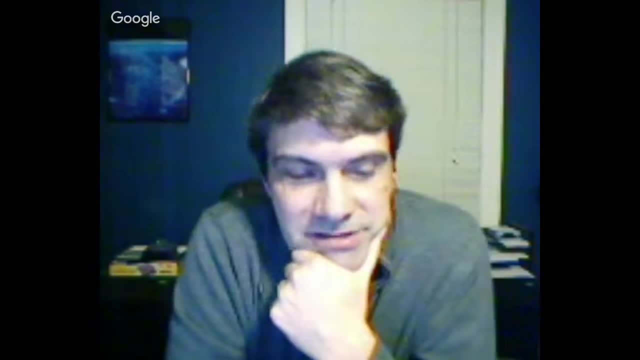 I'm afraid the days of amateurs discovering asteroids are pretty much long gone. Those robotic surveys that exist are just catching them left and right, And when something like the LSST goes online, you can forget it. Amateurs are just, you know. I think there was an article. 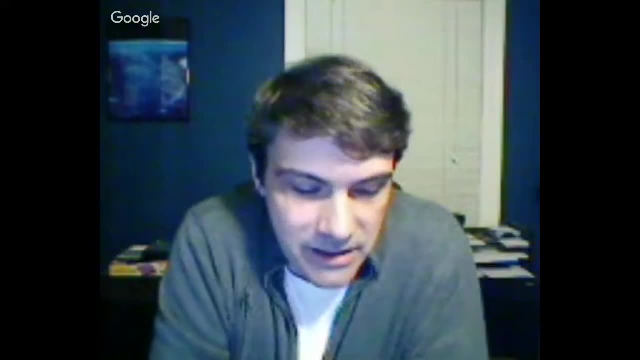 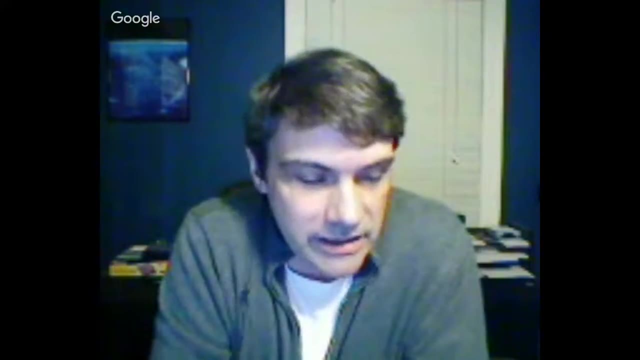 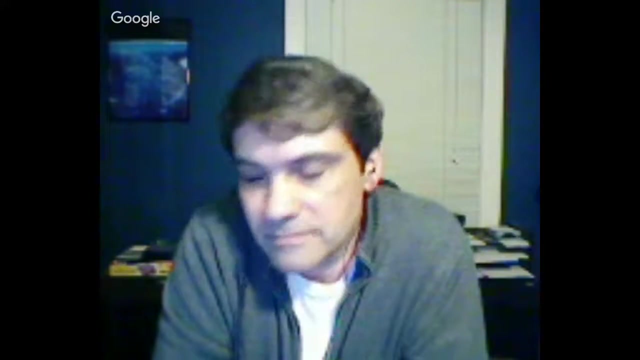 in Sky and Scope, or something recently about the days of amateurs discovering comets, are pretty much gone, And it's because of these automated surveys that just pick them up before anything else. Yep, But that doesn't negate the need for follow-up, Right, right. 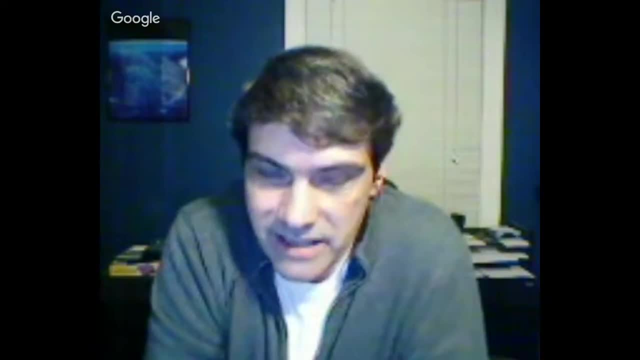 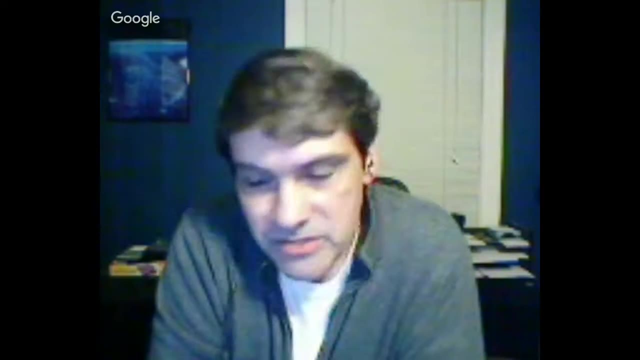 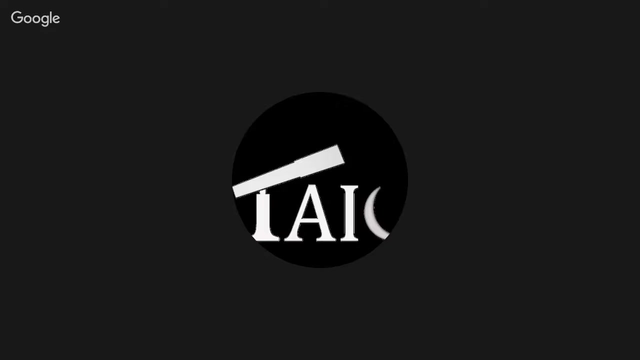 They're finding so many of these things that they leave all- pretty much all- the follow-up work to amateurs And smaller observatories. So there's a huge need for follow-up work. Steve Segarian's got a good question And now I know you mentioned earlier. 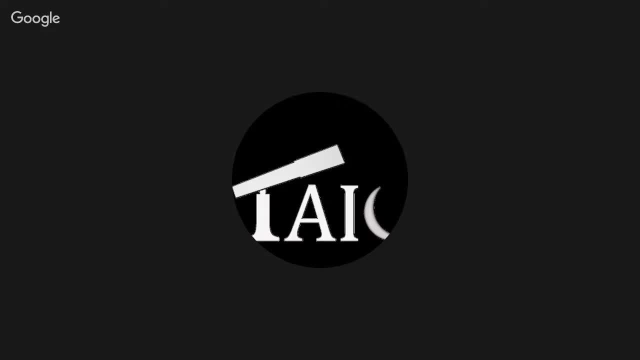 that MPC requires a permanent observatory. But his question is: can any of this be done offline and then do your observations at a dark site without internet connection? I think is the way I'd phrase it, So like do the prep work and the targeting and whatnot offline. 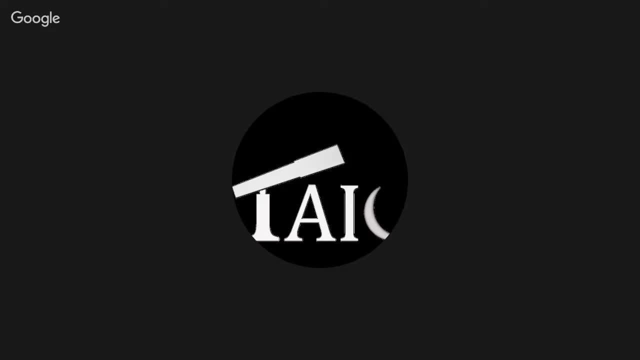 And then at a dark site, do it. Yeah, Dennis Wilde's saying you need accurate time, But that you might be able to manage that Accurate to one second. I don't. yeah, yeah, You know the thing is, you know. 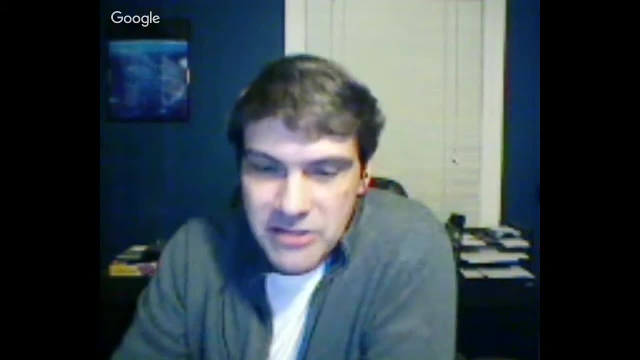 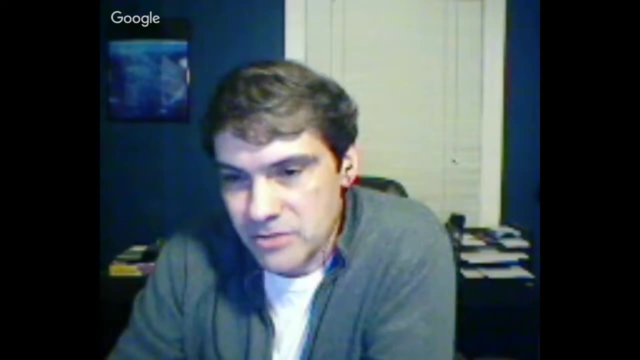 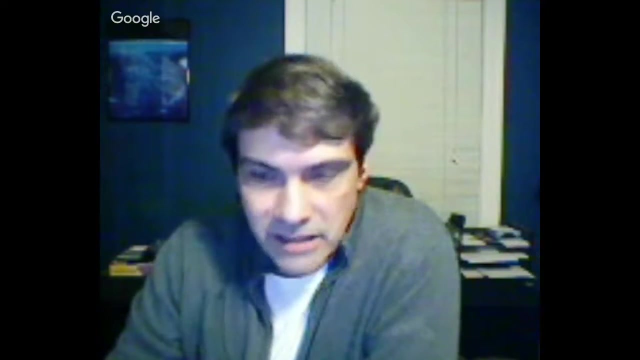 the thing is that the Minor Planet Center, when you submit your observations, those are topocentric positions specific to my observatory in my backyard, And the Minor Planet Center, I believe, just first converts those to geocentric positions and then uses those for the orbital calculations. 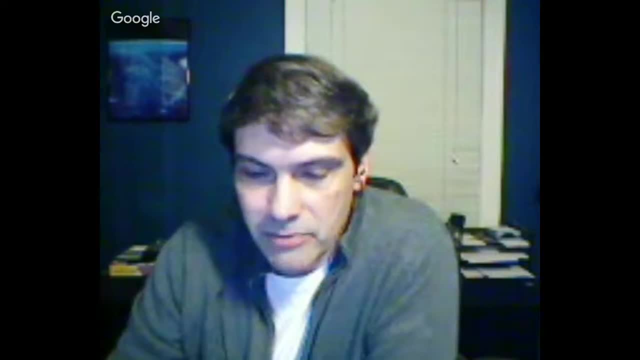 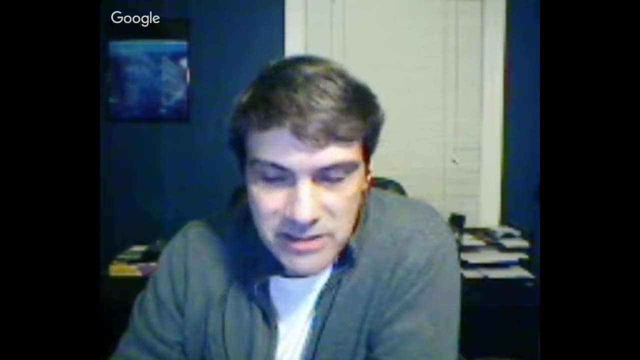 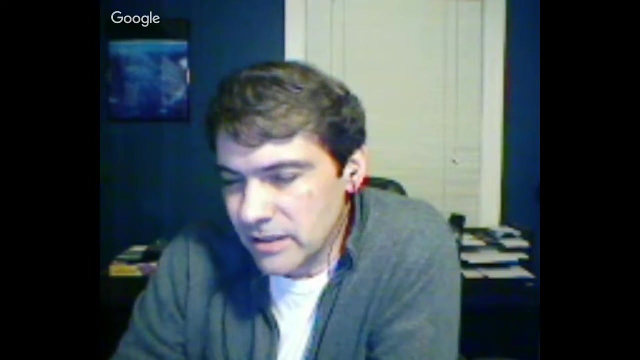 So that's kind of, I think, one of the reasons why they insist on a permanent location. they need to know the latitude and the longitude and the altitude of where these measurements are coming from. I think there is a way to include that in the header file. 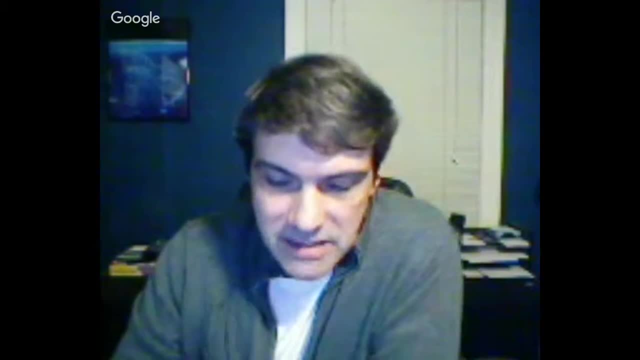 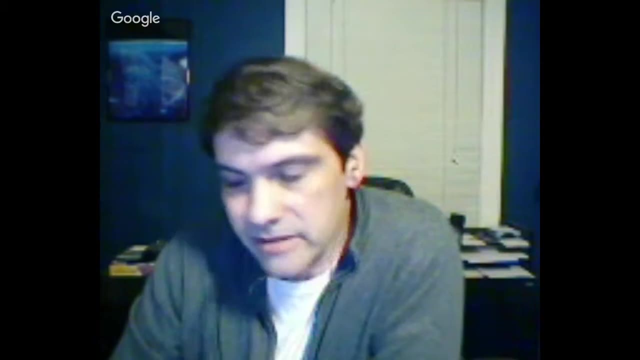 If you don't have an MPC code, you know there's a whole process of how to submit these before you get your MPC code And you need to include that info in the header that you send off. And again, that's all laid out in that document. 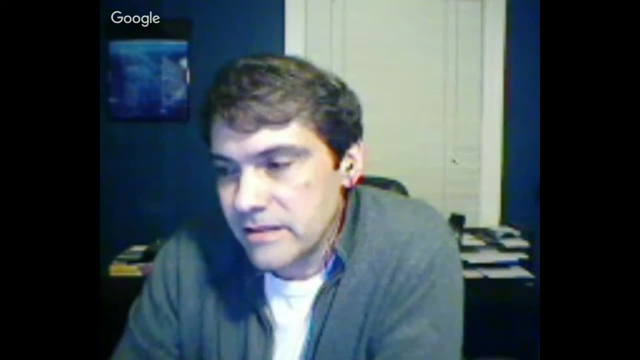 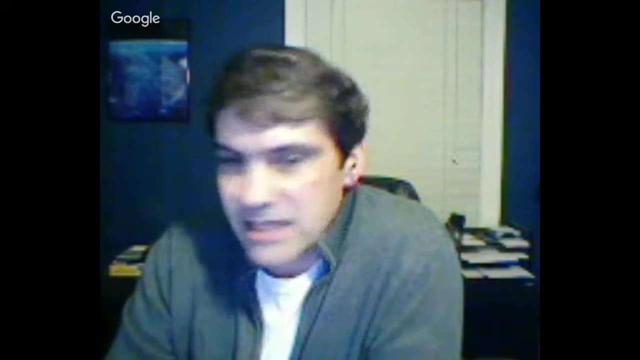 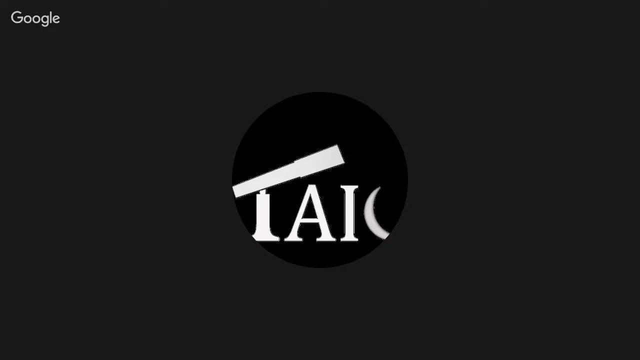 getting started. But as for seriously doing this from anything but a permanent location, I think it's going to be more problematic than anything else. Gotcha Yeah, for I mean I can think of some ways to overcome it If you have cell phone reception. 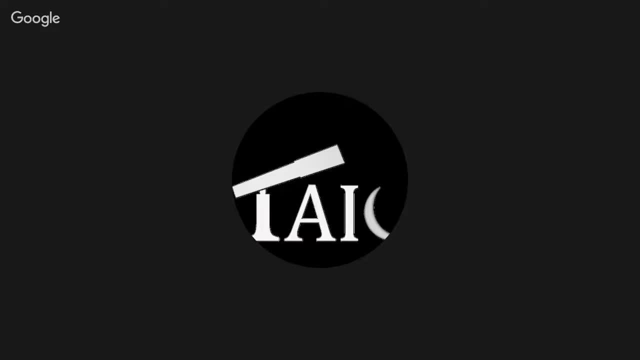 you can set your cell phone up as a hotspot, but that's still not going to give you that accurate longitude, latitude, altitude that you want to have and have it repeatable and know exactly where you are. So you might introduce more error into the data then. 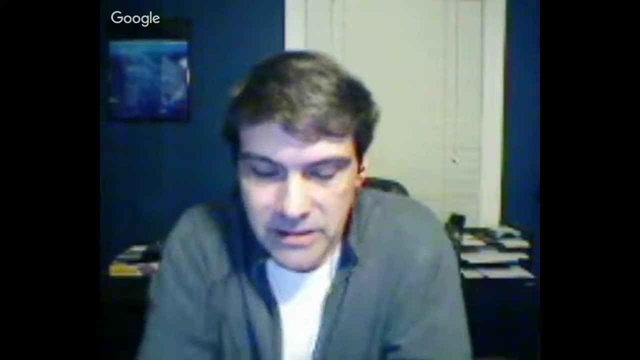 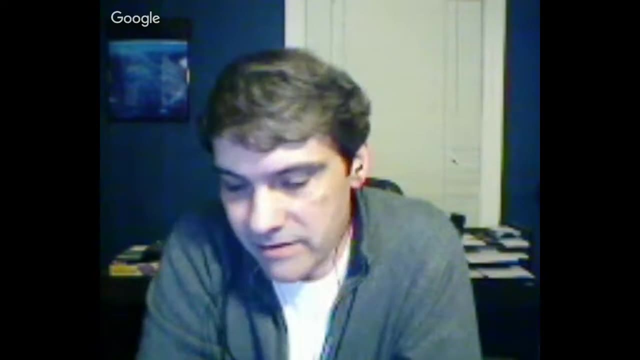 Exactly. Yeah, you really. I mean you want to try and do as good as you can when you submit these things, because the folks at the Minor Planet Center are just overwhelmed by all this data they're having to deal with, And if you've got one person, that's kind of 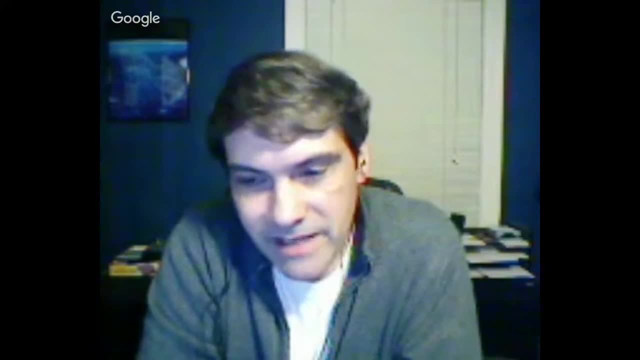 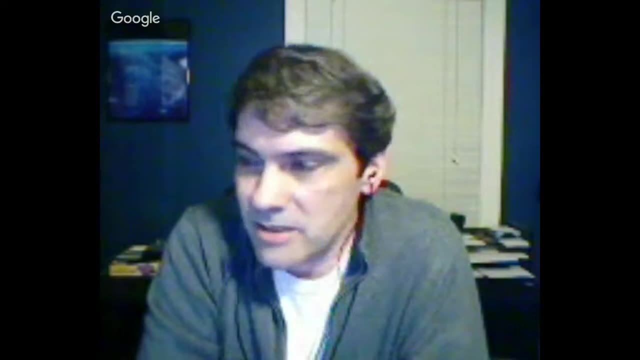 you know, submitting flaky data. it's just something that they don't really have the time to deal with It really, you know, they are just overwhelmed, Yeah, And they don't know them as much as you can imagine there. 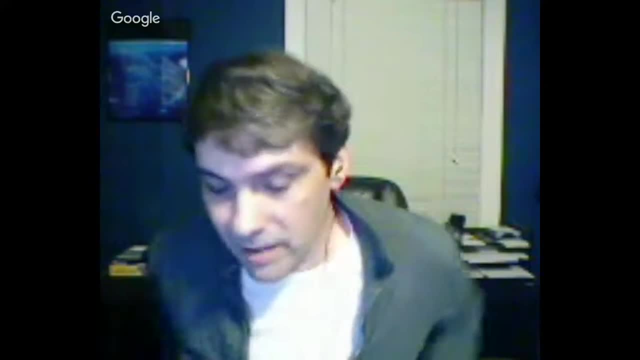 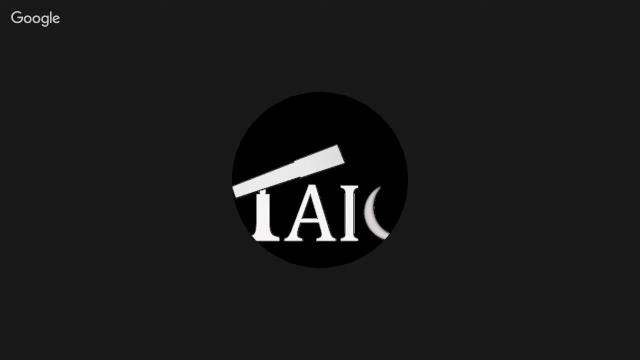 But they do want, you know, they do really need people to do follow-up. It's just you've got to be careful, Right, Yeah, and Steve's saying what about? well, so Dennis is saying you can request another code. 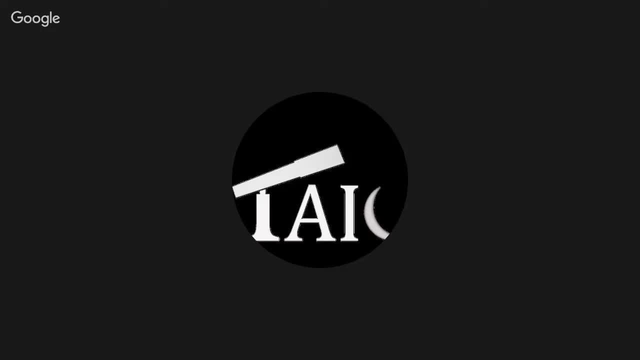 if you use the same remote site, which might give you an opportunity to use that, I think the internet. you need the internet to constantly update your time or constantly correct your time. There are a few things to overcome, So you want to be certain you're getting good data. 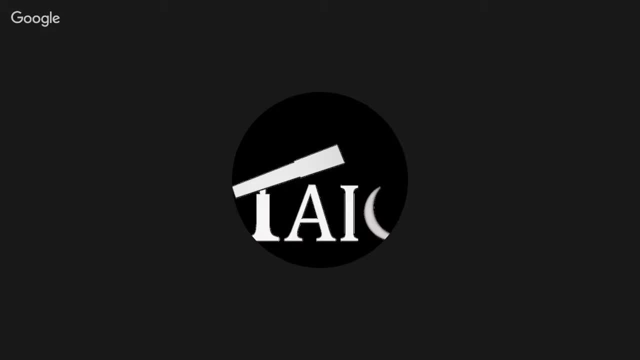 with everything adequately stamped. I mean, if you want to test it out and see what you could do, you could probably test it out. But I think before submitting it you want to make sure that it's kind of that it's something you'd be willing. 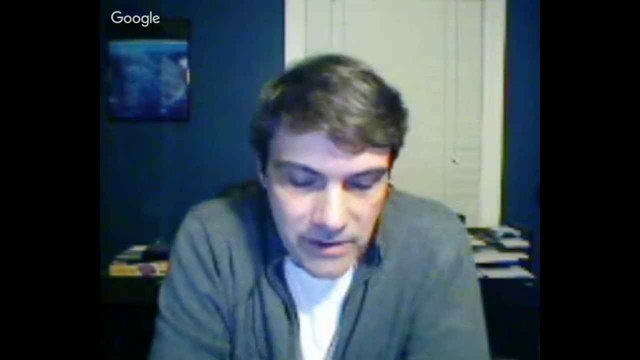 to sign your name to. Oh sure, Yeah. And actually in one of the screencasts I talk a little bit about, you know, hey, you can take your TAL score. you know, hey, you can take your TAL score. 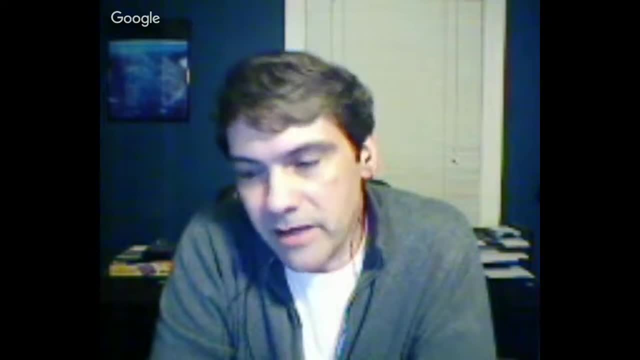 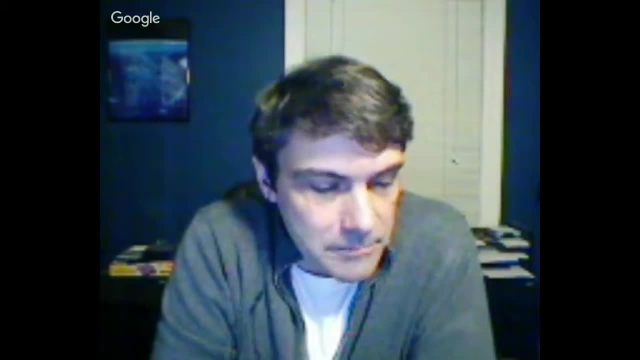 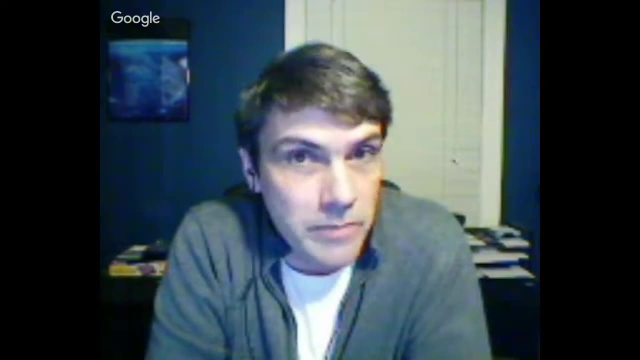 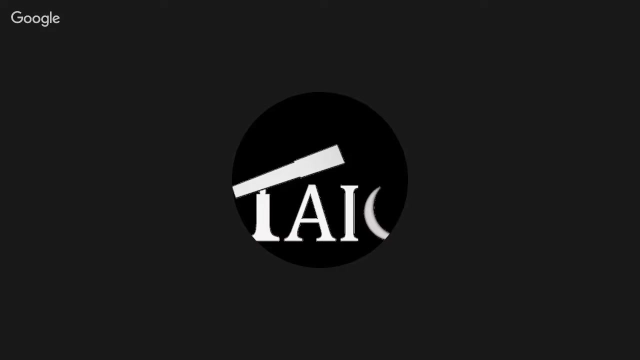 or wherever- take some measurements, measure them and then you can do a little fudging in the Findorb program And you can compare your measurements right there with all the other measurements, just to see how you're doing. Mm-hmm. 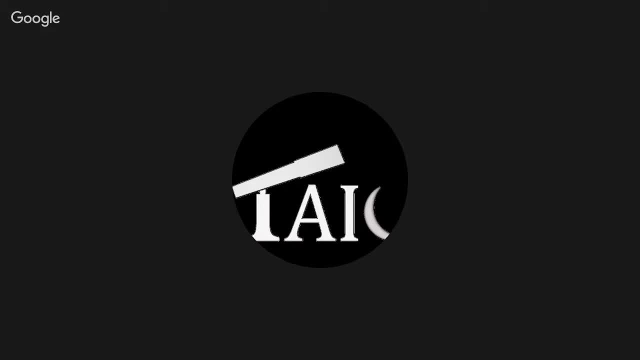 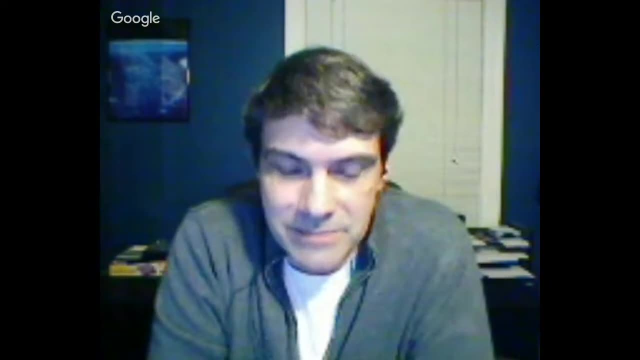 Cool, That was a cool-looking Clark telescope. You get to use that frequently up there. Yes, I've been a volunteer at the Cincinnati Observatory since about 1983. And I've spent many hours with that telescope and with the very old one from 1845,. 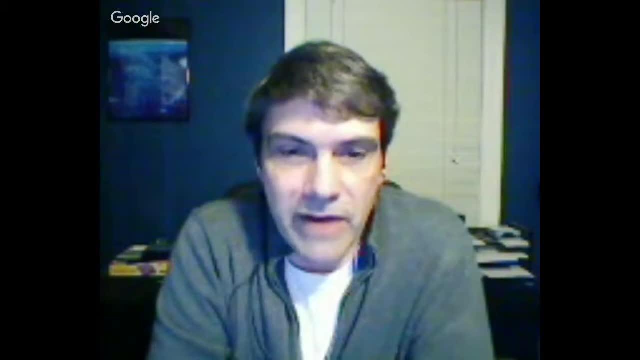 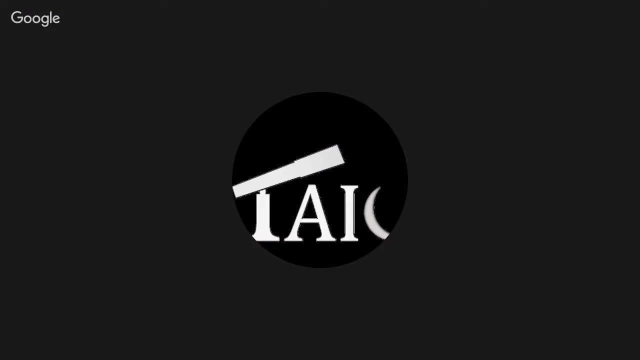 the 11-inch Mers and Mahler refractor. That is a beautiful antique telescope that still works quite well. Mm-hmm, Mm-hmm. And the Clark was a 16, you said right, Yep, That's circa 1904.. Yep. 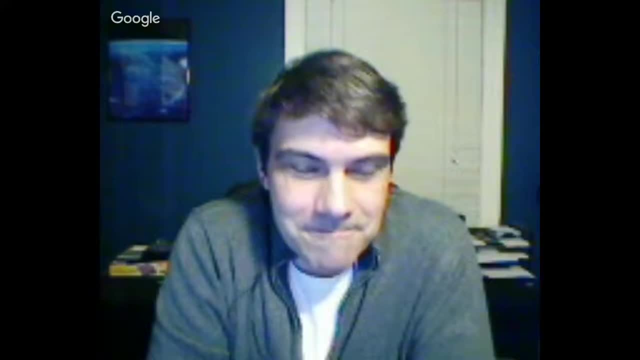 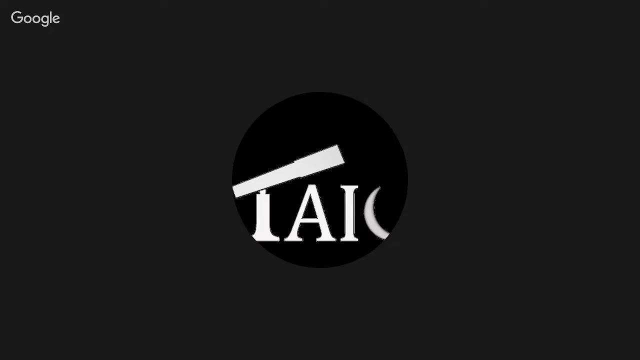 That's insane. That's a big refractor. Yep, Our club has an 8-1⁄2-inch Clark lens on. I guess the tube just didn't make it over time- And I think of that as being a big telescope. 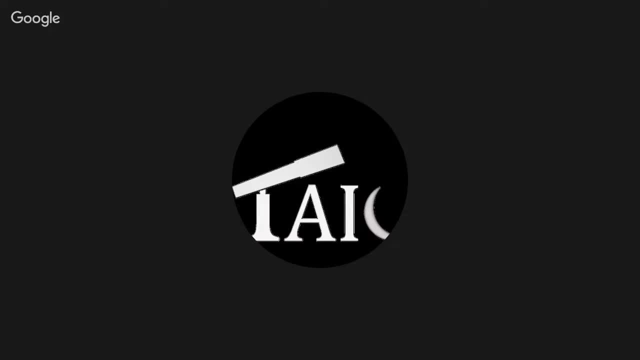 But a 16-inch refractor? that's kind of crazy. It's a beast. Yeah, It is. This is your Parker in the haya. How did all of this break down? Thanks for defaulting. Just joking A moment. I won the fyro for a bad guy. 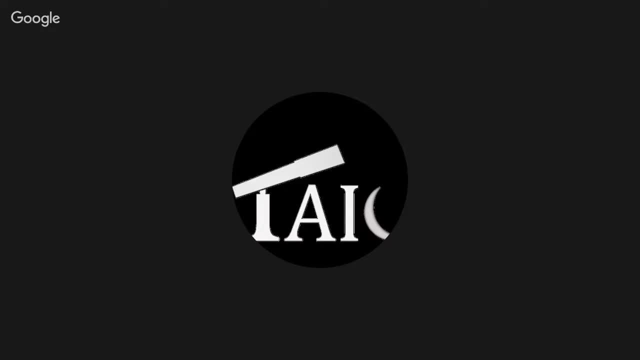 Back to theory. Heику, what did I just see here? Did anyone go into NEAC? I know Alex is going into NEAC. I'll be at NEAF, In fact next week's session. I'm hoping to do kind of a recap of NEAF so I could try and practically look at what some of the interesting things I saw at NEAF were. then expion all you weird animals in the PCs where you went. 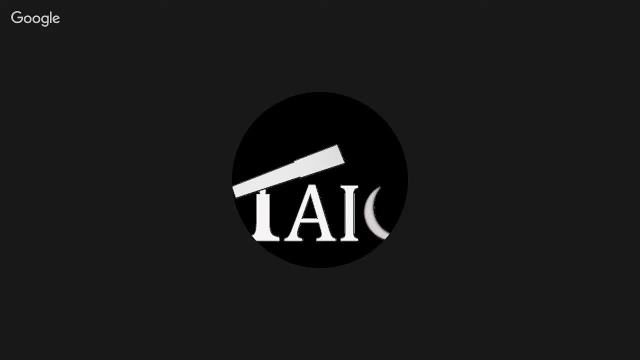 What did you look for, Alex? Nice, very nice, Thank you. In one of the follow-up presentations we're going to go in more depth and hopefully have some other stuff to present. Wow, Dennis Wild's club has access to a 23-inch Clark.